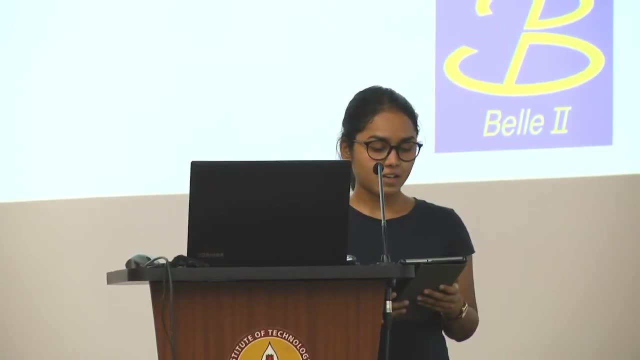 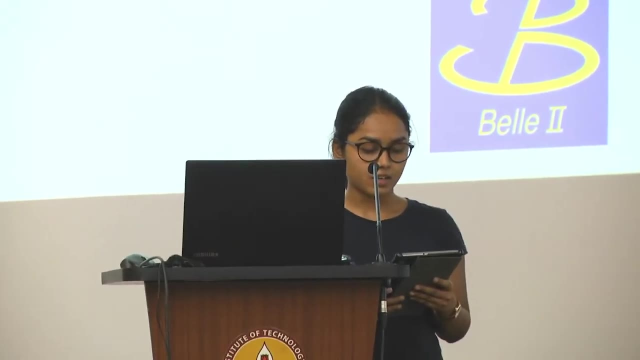 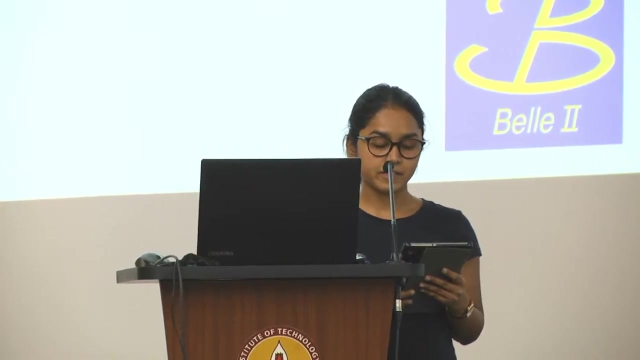 I welcome you all to this semester's in-house colloquium lecture. Our speaker for today is Professor Jim Leiby, who is going to talk about flavor physics at the intensity frontier at Bell 2, with very promising physics prospects indeed. Professor Leiby is an experimental particle physicist in the Department of Physics here at IOTM. 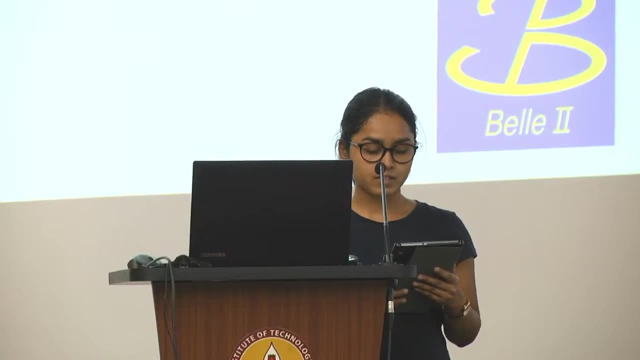 He received his doctorate from the University of Oxford, working in electrophysics- electrophic physics, with the Delphi Experiment at CERN. Since then he has worked primarily on flavor physics, focusing on the measurements of matter-antimatter asymmetry. 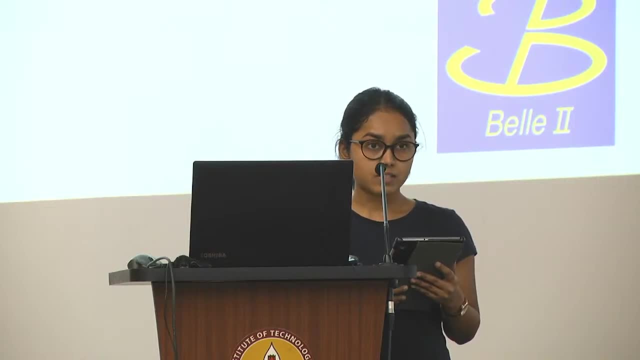 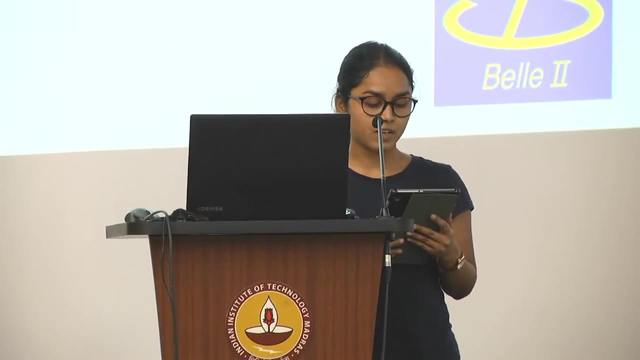 in the bottom and charm hadron decays, as well as on rare decays and instrumentation. He has held research positions at Stanford, CERN and the University of Oxford, while working on various experiments like LHCb, BABA and CLIO-C. 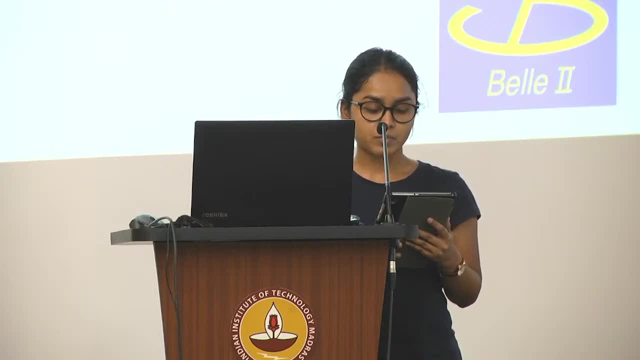 He has been a member of the IOTM faculty since 2009,, working primarily on Bell and Bell-2 experiments located at Keiki, Japan, on which we shall be hearing extensively from him in today's lecture. So, without any further delay, let us welcome Dr Libby. 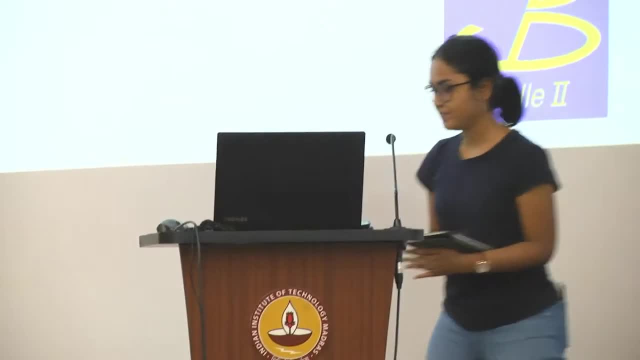 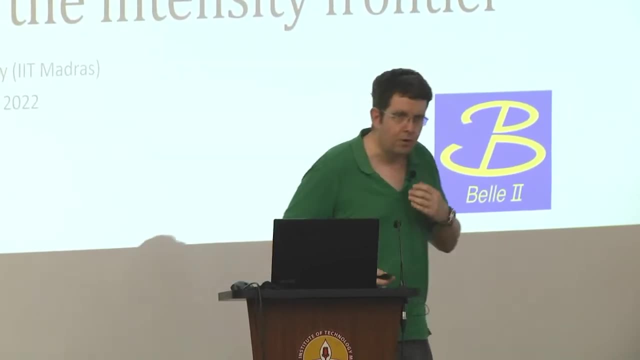 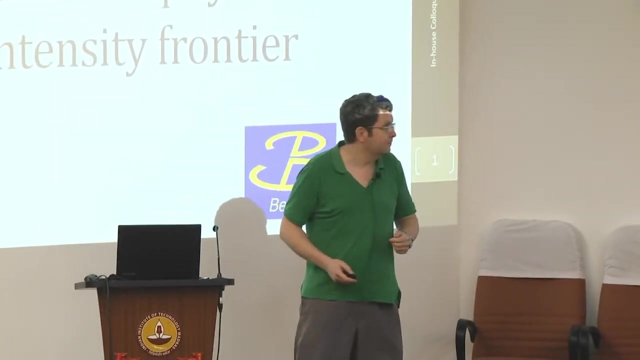 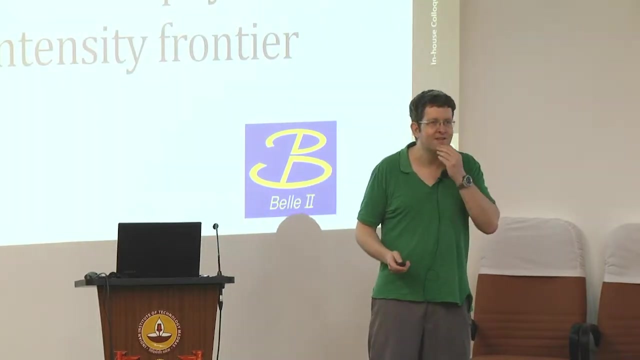 on stage. Hey, can you hear me? Yeah, So thank you very much, Anita, for the introduction. So it's a very novel experience I'm having. I don't actually remember seeing this many people and speaking to them for a very long time. 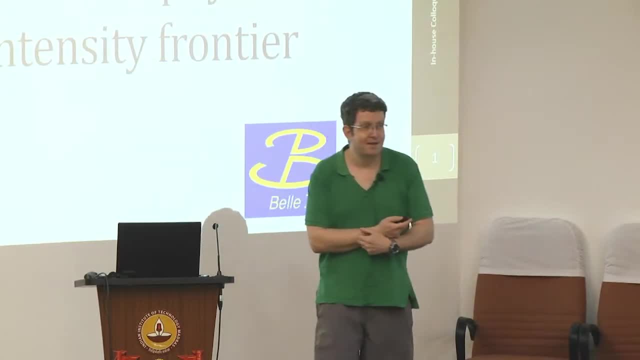 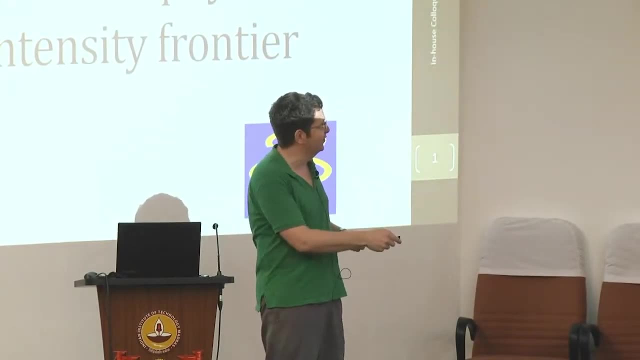 But I know you're just here for the cake, so I hope you enjoyed it. But I'm going to continue the culinary theme slightly by talking about flavor physics And I have to sort of spend a bit of time really defining what these two things are: what flavor physics is and the 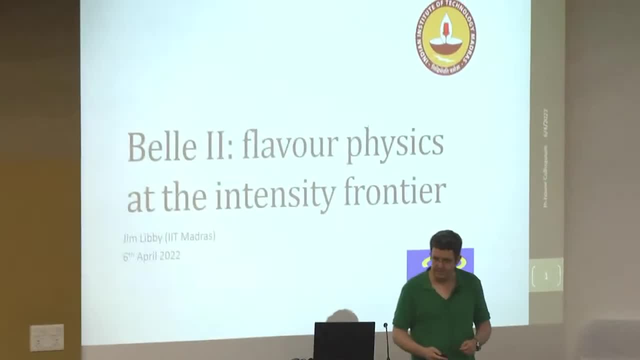 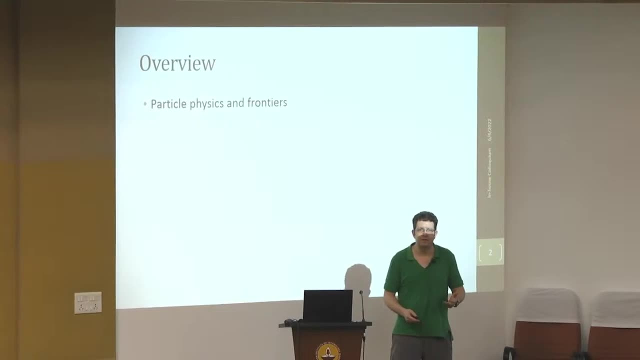 intensity frontier before I'll talk about the Bell-2 experiment. So just to give you an outline of what I'm going to talk about, first of all I'm going to introduce this idea of frontiers and how we're tackling problems in particle physics. 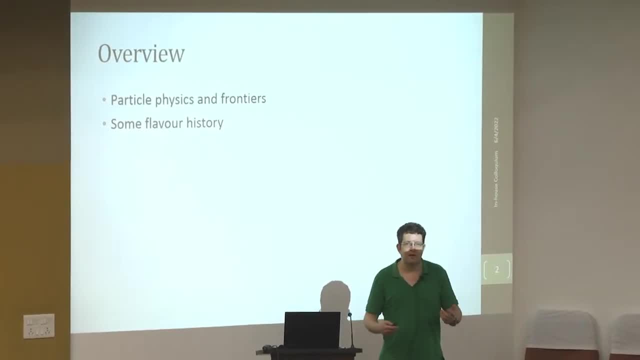 today. And then I'm going to talk about flavor physics in particular, what it is, what it's done in terms of establishing the standard model of particle physics and particularly its role in predicting things that are found at a later date, And I'll explain that in more detail. 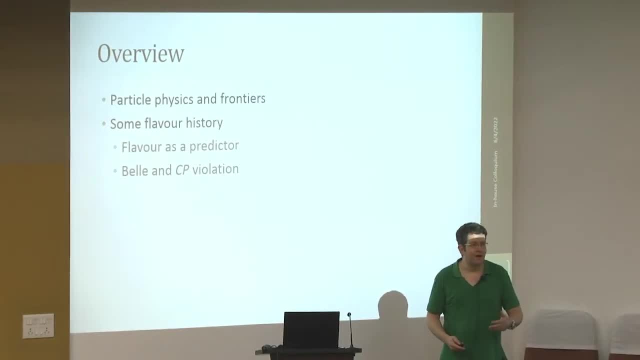 Then if there's a Bell-2, there was a Bell, And I will tell you about the Bell experiment briefly, and the principal thing that it discovered or is famous for, which is CP violation. It's something that we work on here in IIT Madras. 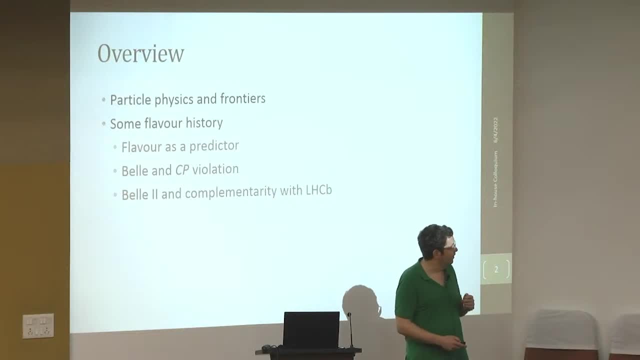 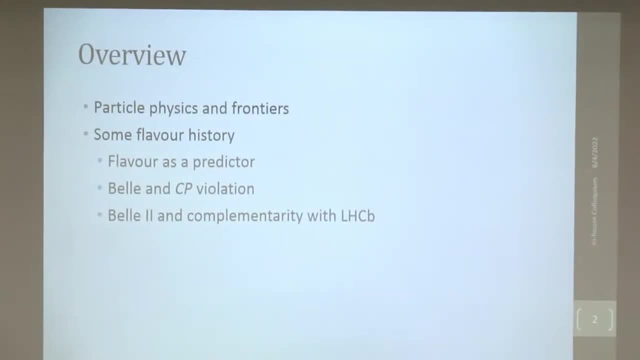 as well, and I'll show you more results about that later on. And then this is a little bit more for the experts. Anyone who knows about flavor physics knows there's a very successful experiment at CERN that is also doing flavor physics, And I want 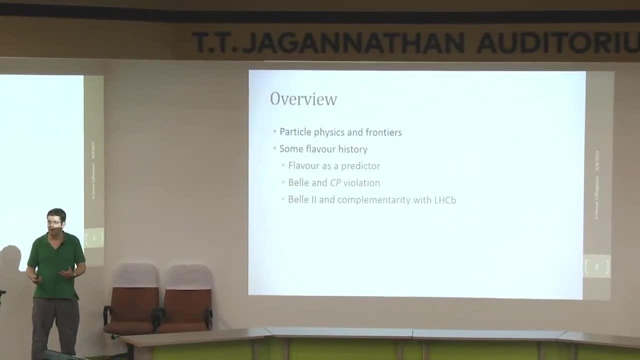 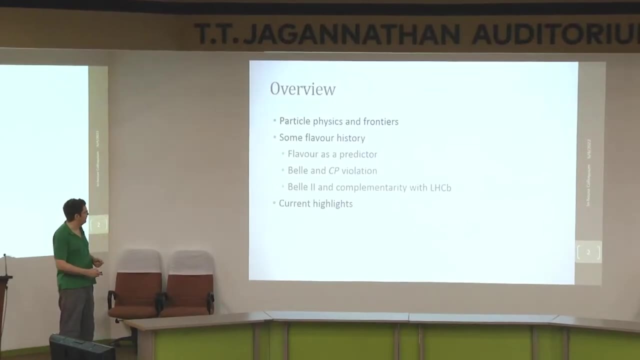 to just try and describe to you a little bit of what's special about Bell-2 in comparison to LHCb And what we like to refer to as a very friendly rivalry, as the complementarity, And then, just to close the talk, I'll show some current 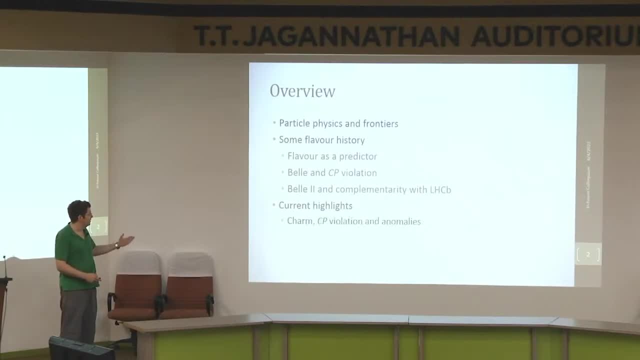 highlights of the measurements that we are making, And those relate to these three topics, which I'll explain as I go through. And, of course, the one that may be of most interest are these so-called anomalies that we're seeing, which may be an indication of some breaking. 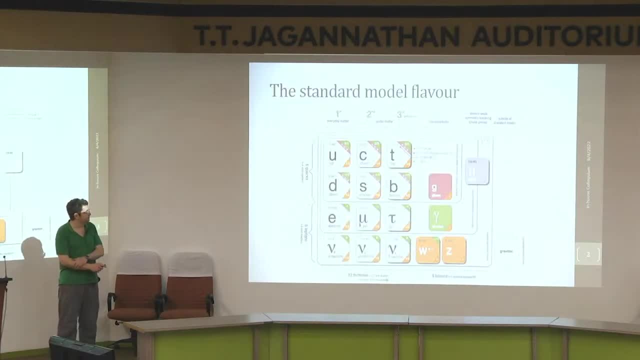 in the standard model. Okay, So any talk about particle physics, one should start by looking at our current best paradigm, which is the standard model, And this is the particle content of everything we know about in the universe. So we have up here. 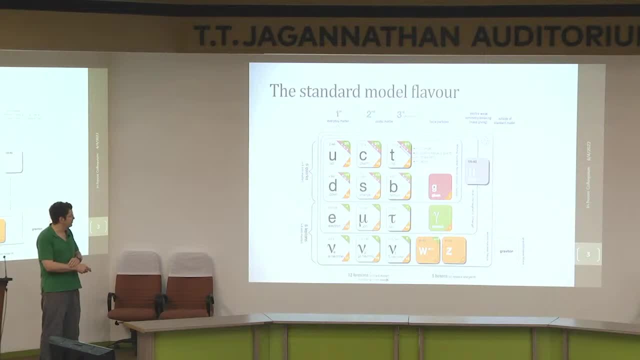 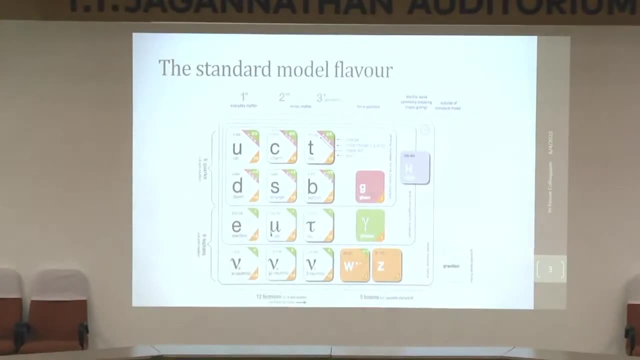 the quarks and down here the leptons, And then on this side we have what we call the gauge bosons, which mediate the different forces. So the quarks feel the strong force, The quarks and the charged leptons feel the. 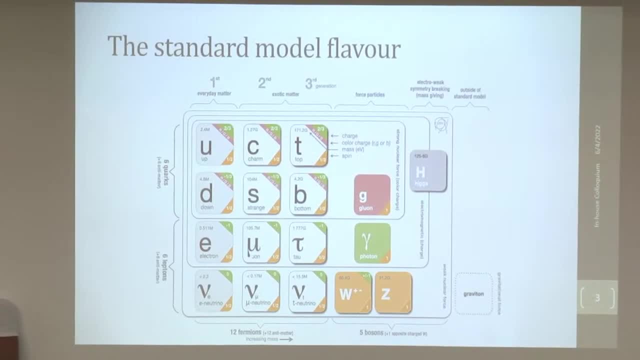 electromagnetic force And then all of them feel the weak force which is the W and the Z. down here Off to the side was the last big news in particle physics, which is the discovery of the Higgs boson, which gives mass essentially to these gauge. 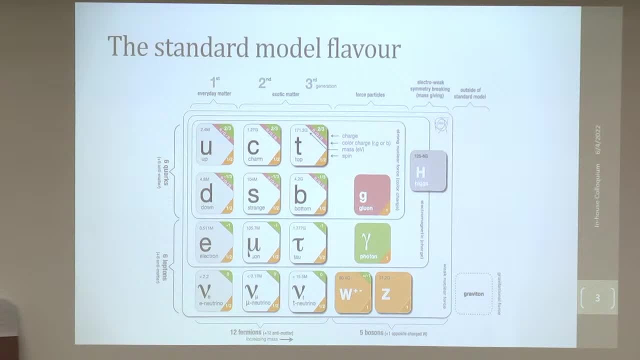 bosons down here and in turn can give mass to the massive fermions as well. So flavor physics is a description of these quarks. the three generations of quarks, up down, charm strange top bottom. So we think of those names. 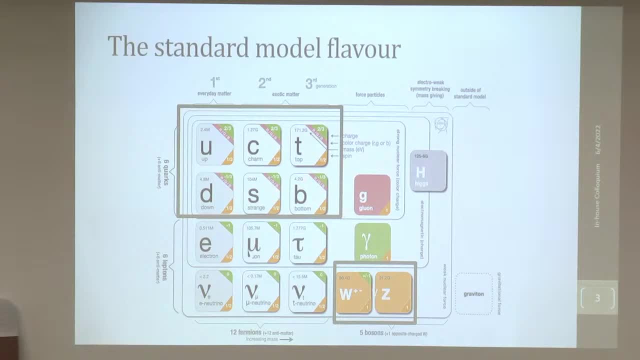 as flavors And the flavors. physics is talking about the interactions between these quarks, which happens just through the weak interaction. So this weak interaction is special because it communicates between the different flavors. The strong and the electromagnetic force just communicate with one type of particle at a time. 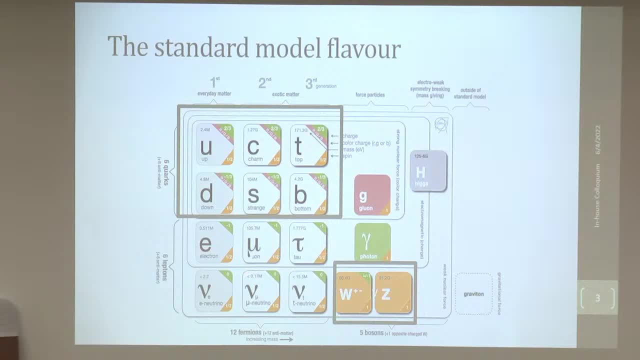 Of course, there's flavor also in the leptons that these electron, muon and tau also are the lepton flavors, But what I'm primarily going to talk about is quark flavor. So this is an extremely successful model. 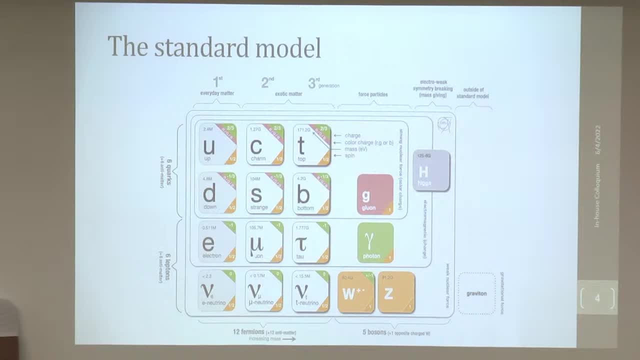 And to show that, I'll show you the number of Nobel prizes that this model has been awarded over the years. So it's been 50 years in the making And I could go through these exhaustively, but for various discoveries along the way. 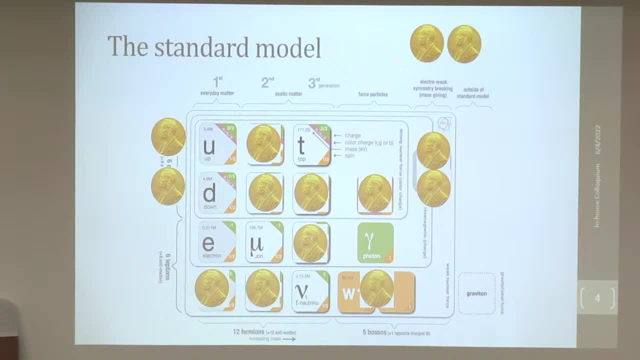 of certain particles, paradigms of the model. So this is Glashow-Salam-Weinberg and Tehuft and Veltman, And then, of course, going up to the Higgs boson and the symmetry breaking, So most other. 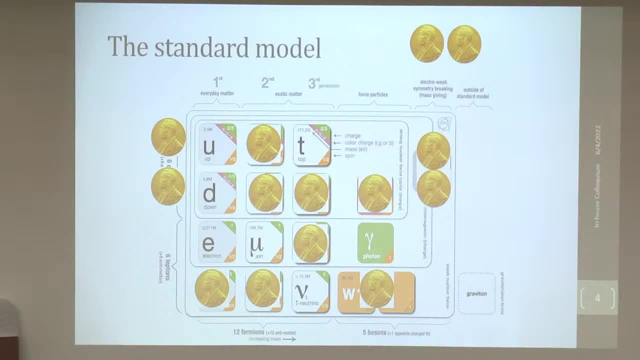 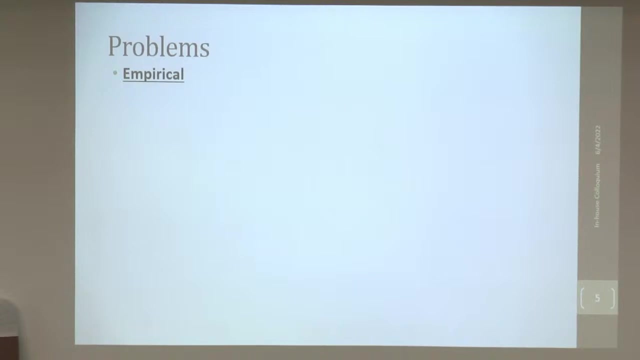 areas of physics gets very frustrated. The particle physics has been rewarded so much for one thing, But it's essentially got very few experimental flaws that we can find in the laboratory. But we know it's not a final theory of particle physics And there are certain problems with it. 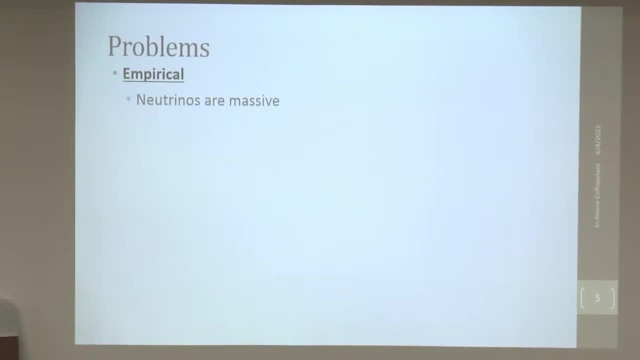 Particularly, one that's actually well known and has been around for a while, that the neutrinos are massive And that cannot be incorporated within the standard model of particle physics, And that has already been awarded a Nobel Prize for that observation. So, Kajita-san. 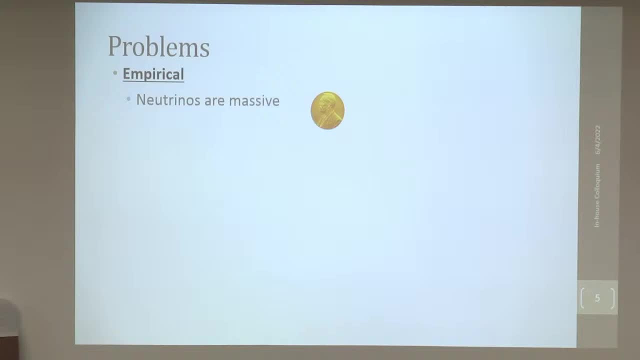 who spoke, I think last semester, was awarded that along with Art MacDonald. So there are other things, usually coming from cosmology, that we now know about. There's dark matter in the universe, There's dark energy. I can't tell you much about that, I don't think. 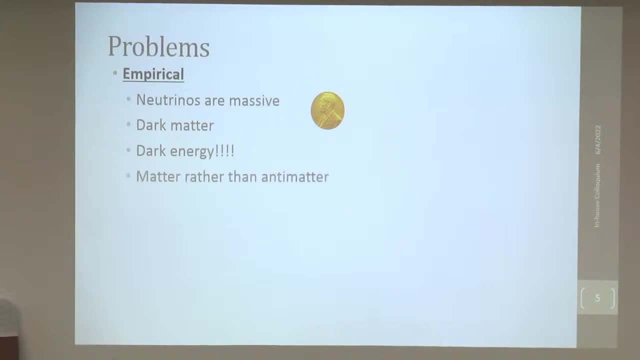 anyone can, And there's much more matter than antimatter in the universe. That is something that is related to my talk, though, again, we probably don't have the solution in quark flavor physics. And, of course, there's gravity. 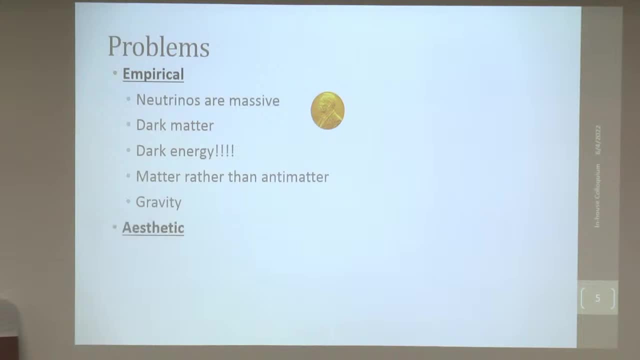 There's gravity that stands outside the standard model. Now there are aesthetic problems with the standard model as well, And those are things that theorists like to talk about a great deal and try and come up with a better theory. For example, why do we have three generations? 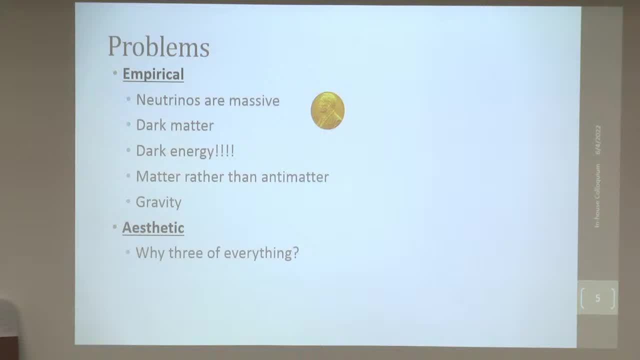 of these quarks and leptons? That's an arbitrary number. Why not four? Why not two? Why not five? The model is very empirical. We have measured 18 parameters that go into it, to high accuracy in some cases. But why do we need all these? 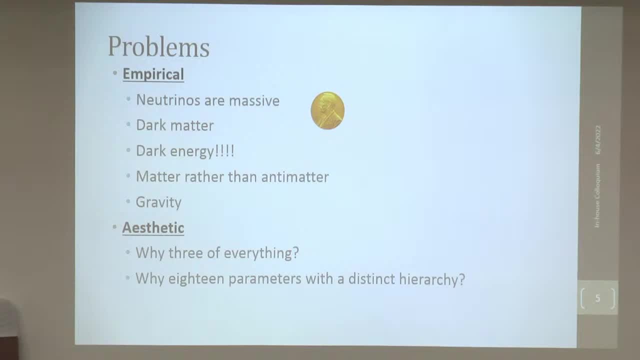 parameters and why do they have such a distinctive hierarchy is not well understood, And, as an example of this, there are certain parameters, particularly the Higgs mass and electroweak couplings, that have to be tuned to the 18th decimal place, which is 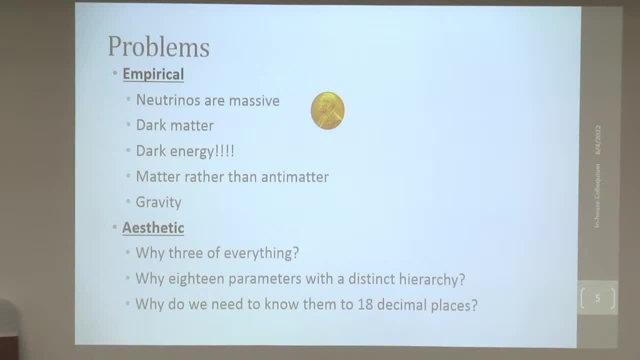 a highly unnatural thing to do to get the model to be stable, Because we can't measure to that level. but we just need the numbers to work out And there are solutions beyond the standard model physics which will solve many of these things. Of course, the ultimate goal is to unify all. 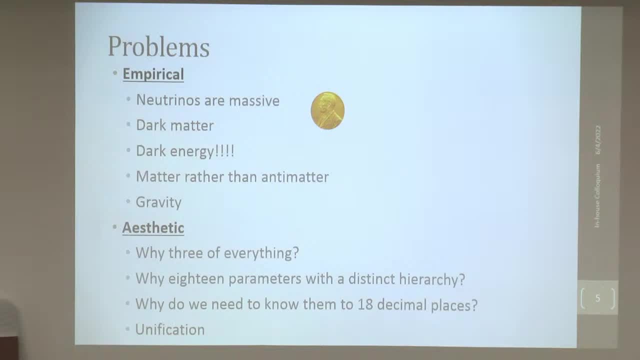 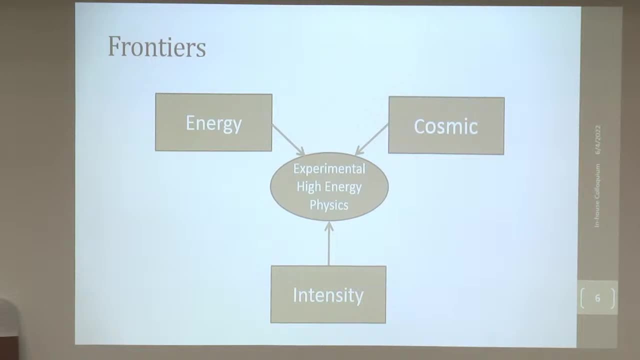 the forces together, We've managed three. Why not include gravity as well? So how we tackle these outstanding problems is in terms of frontiers, or experimental frontiers, And there are three of these: One is energy, one is cosmic and one is intensity, And I'll briefly describe. 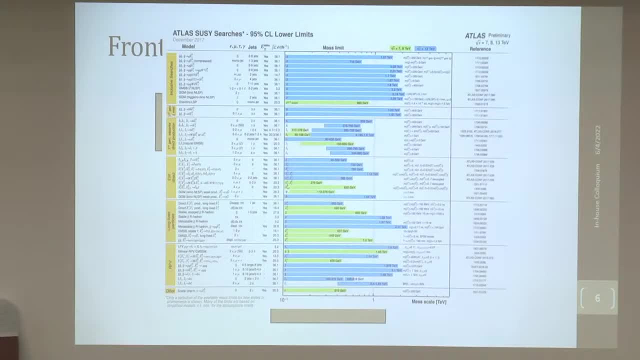 the energy and the cosmic before moving to the intensity one. So this is the energy frontier, This ghastly-looking plot I won't ask you questions about. but what it's saying is we've looked for an extension of the standard model, something called supersymmetry. 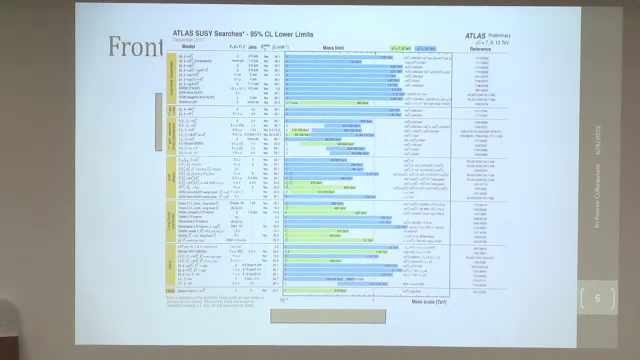 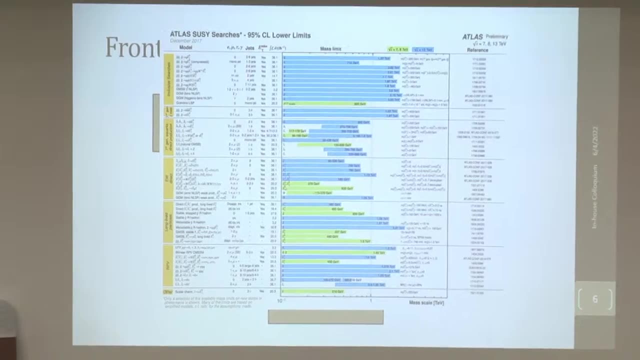 which may well be familiar to many of you, where a boson has a fermion partner and a fermion has a boson partner. And these are limits set by the ATLAS experiment at the LHC, which is colliding together protons at the highest energies. 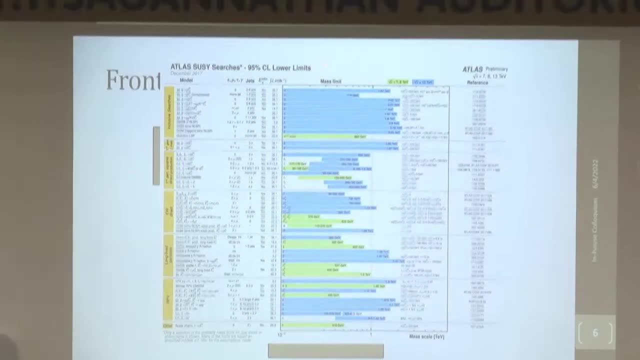 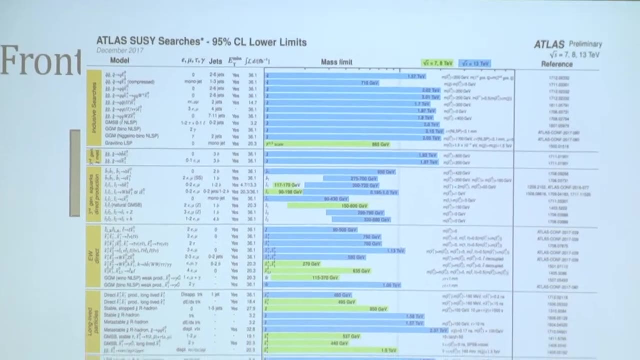 we've managed in a collider at 13 TeV And they haven't found anything. but they set a limit of many TeV on some of these particles, or several TeV. So that's the energy frontier, The cosmic frontier we know there's. 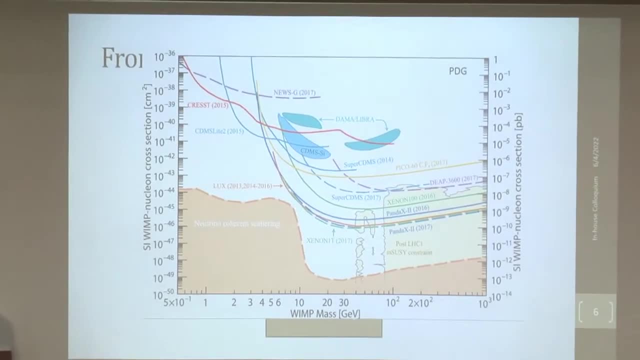 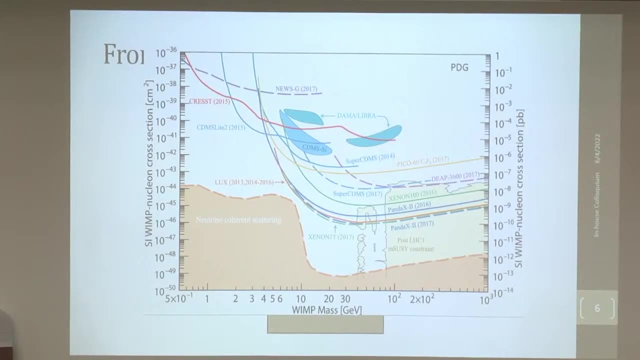 dark matter out there, And so, for example, there are searches for the dark matter that should be passing through all of us all the time as we go around in our solar system and in our galaxy, And this is a plot showing various experiments to very precise measurements. 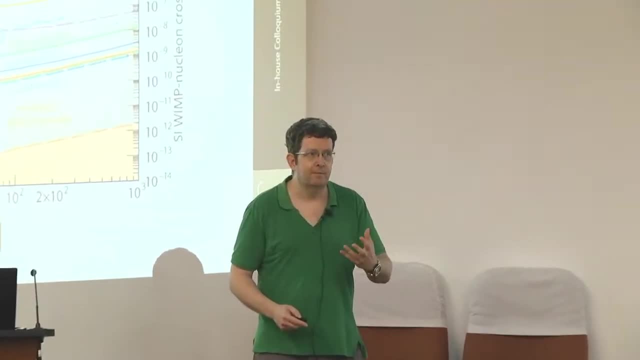 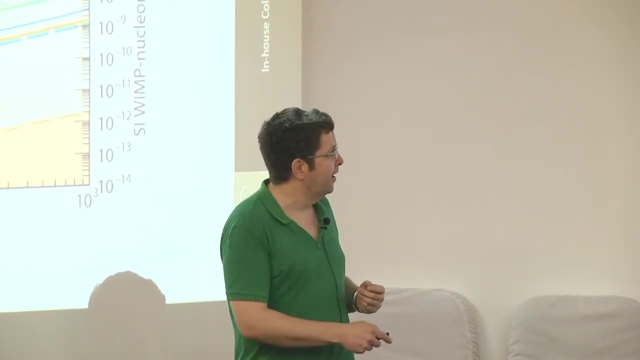 looking for tiny signals that could come from one of these dark matter particles which are not interacting electromagnetically, might be interacting a little weakly with new nuclei, And you can see their signatures And they set limits down to some very very. 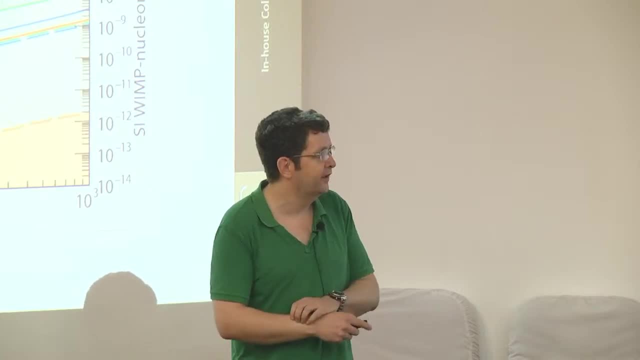 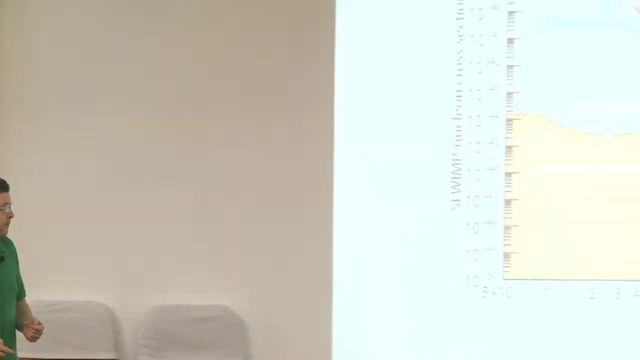 small numbers in terms of cross-sections, down here to 10, to the minus 46. And essentially we haven't seen anything yet, apart from some strange observations here which are not borne out by other experiments. There's no direct detection of dark matter. That's a kind of cosmic. 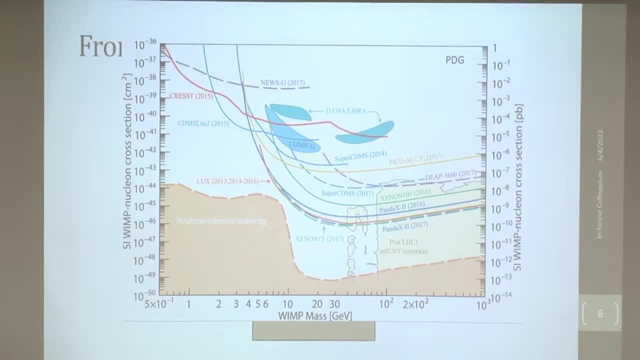 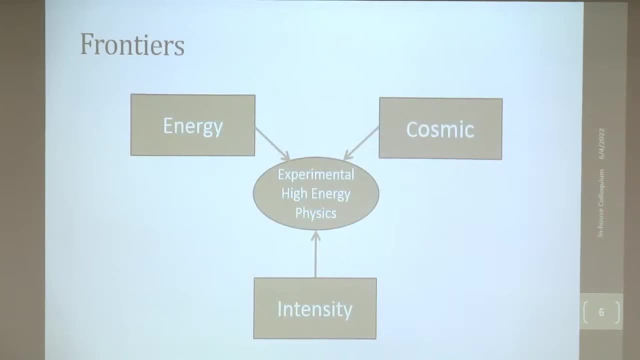 frontier experiment. You can also do things with cosmic rays and cosmic neutrinos and gamma rays and things like this. So I move to the intensity frontier. The intensity frontier is about making precise measurements and looking for very rare things, So we have to produce billions. 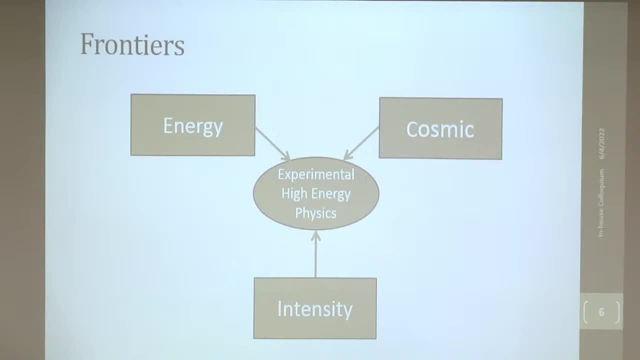 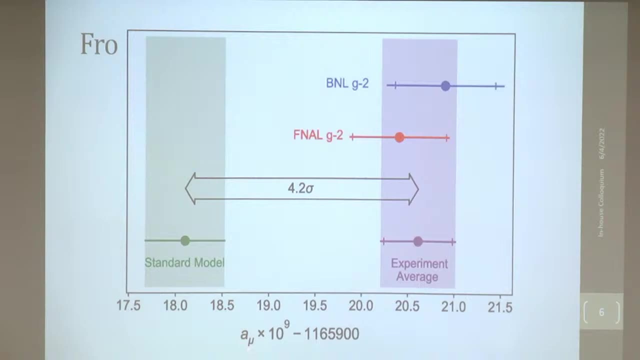 of particles to do this. So it's all about high precision. So a current example of this, which is quite been in the news last year, is this thing called AMU, which is the anomalous magnetic moment of the muon. So this is being measured by a. 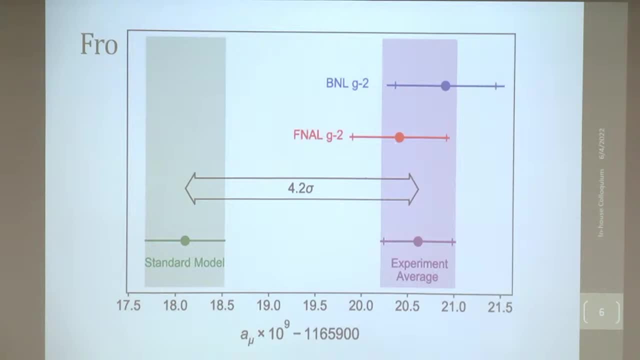 very intricate experiment at Fermilab in America, the so-called FNLA G-2.. And we can predict this, essentially the coupling of a muon with a photon, considering all the higher order corrections very, very precisely. And doing this we see: 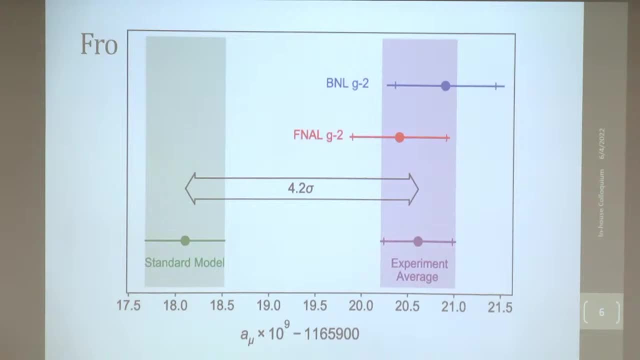 that this is offset by 4.2 standard deviations. This is quite significant. However, I'm telling you a partial story here, because there are other theory predictions that sit much closer to this, using an entirely different technique of prediction, But this is the kind of thing we do. 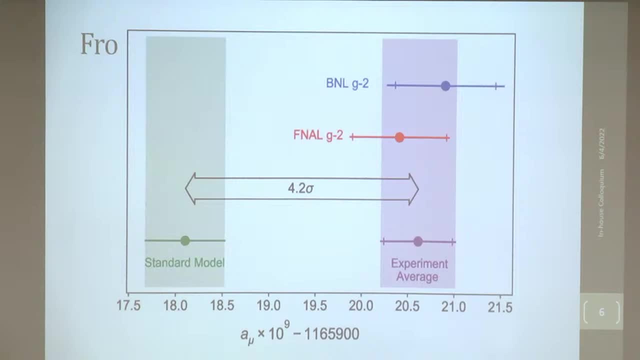 We make precise measurements and we compare it to precise predictions. If there's any tension, that means there's something that wasn't on my first slide, There's something beyond the standard model that has come and changed the results that we see. So 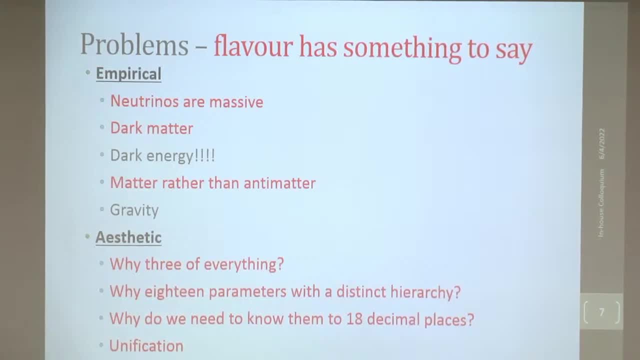 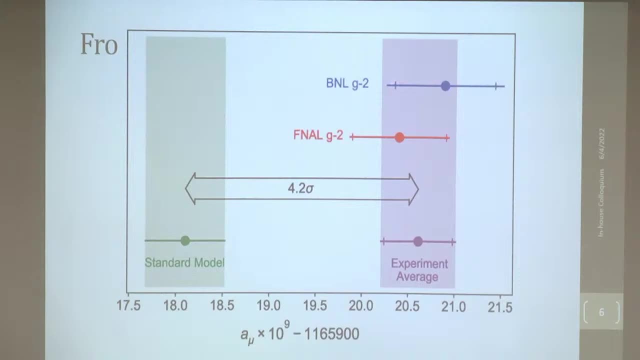 Okay, I could spend. This is a different talk. So this number, This bar here, is a statistical one, so they will take more statistics and this will shrink. This piece is the systematic contribution, which they can also shrink with more statistics. So this band, 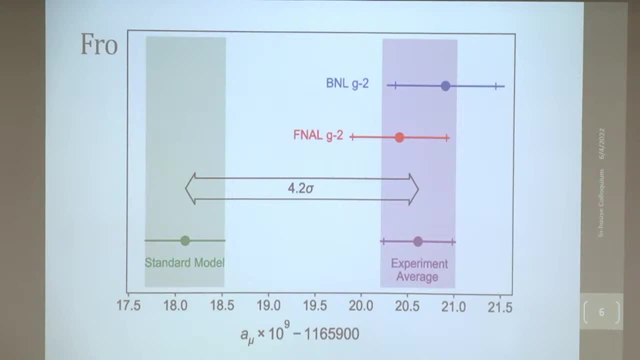 will get smaller. The questions about the theory predictions: there are experimental inputs which myself and Gaurav are now working on here in IIT Madras, But that's again a different talk which can help to understand if this is wrong. But 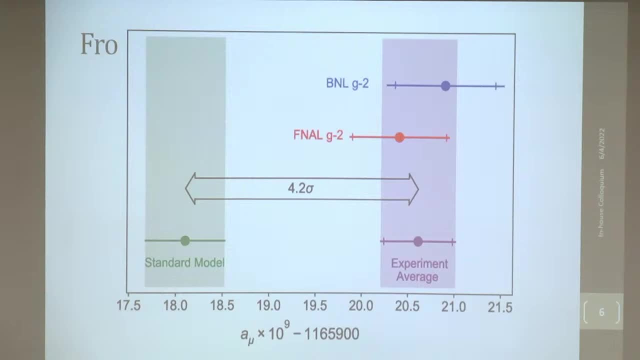 there's also lattice QCD predictions that have to be made and they have to be reconciled with one another. It's going to be a long time to figure this out. It's going to be several years, But it's So. you'd be brave to say this is. 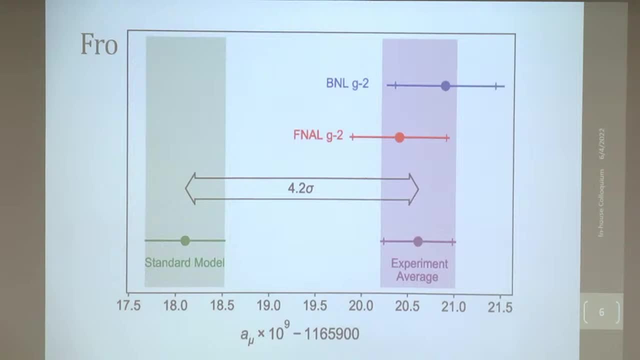 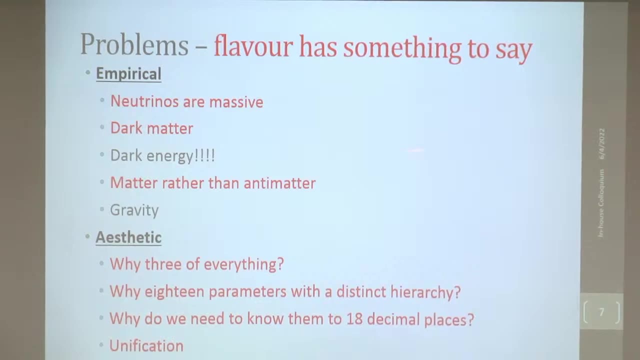 really a sign of new physics, but the current best guess is it's disagreeing. So back to flavour. Basically, flavour measurements can say something about virtually all of these problems, apart from dark energy and gravity. So maybe Sri Ram will lose interest and walk out now. 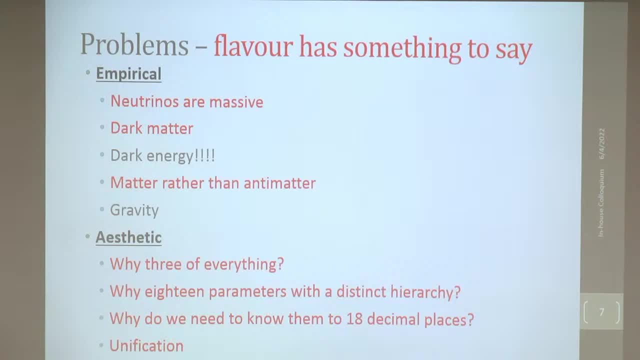 But this, All these other problems we can actually address in some way or another, using the Bell 2 experiment and making flavour physics measurements. I can't describe all of this today, but I'm just giving you a sense of what we're trying to do here when we're making. 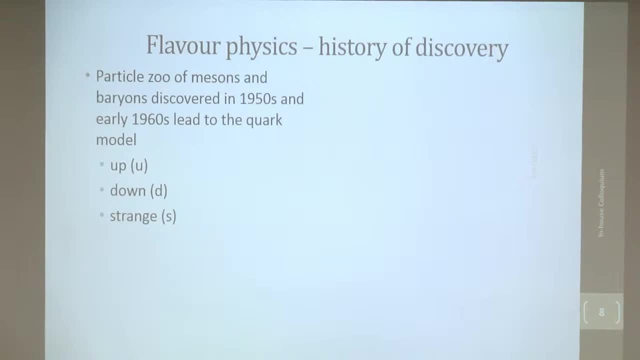 these measurements. So to motivate further, I want to give some history of flavour physics and bring us up to the Bell experiment. So, as many of you may have remembered when you were studying particle physics, we have all these particles. You have to remember what they're made up of. 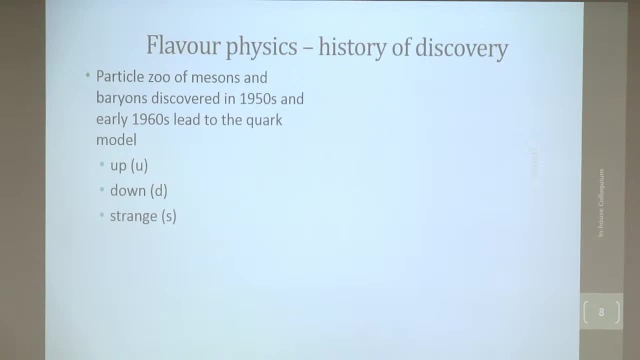 and these various diagrams that we have. But that was relatively ordered compared with what was there in the 1950s, where the same particle had two different names and there was no real structure to what was going on. So it came to something called the Quark model. 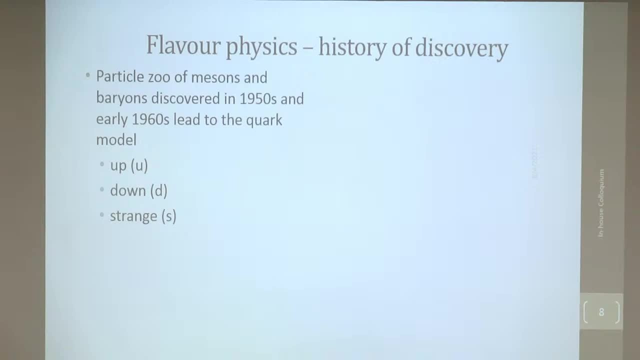 by Gell-Mann and others who suggested there were three Quarks, the Up-Down and the Strange, And with that they could describe most of the things that they were seeing in terms of those light particles, light-quark particles that were there, the pylons. 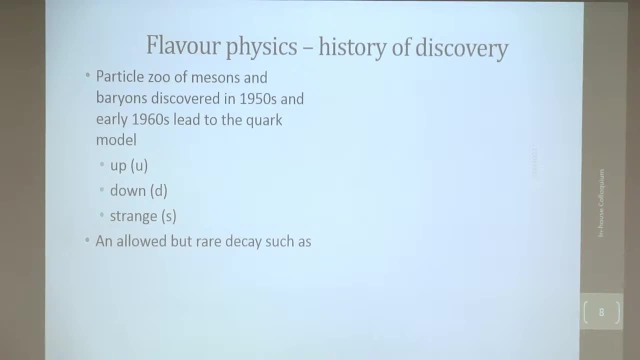 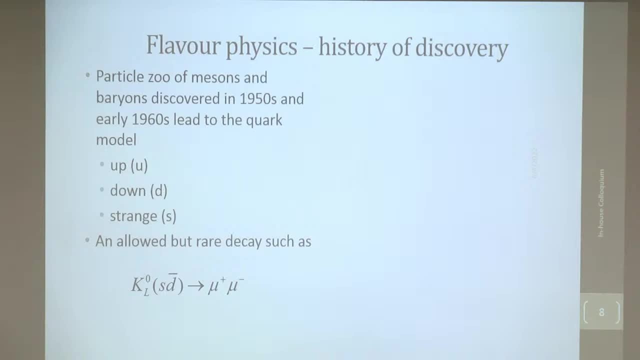 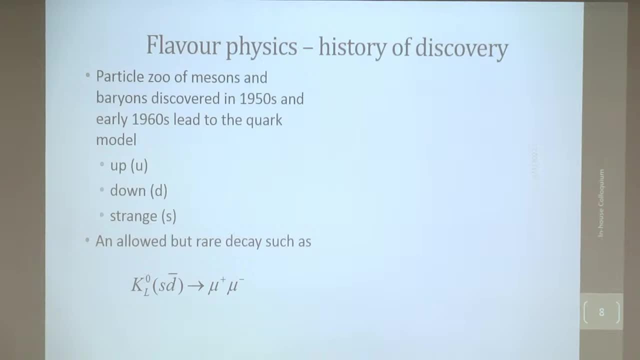 at some rate, And they kept looking for this. This is a really easy thing to see in our experiments, but they didn't see it. So to look at this in the Quark model picture or our modern view of particle physics, what you have is this Strange Quark. 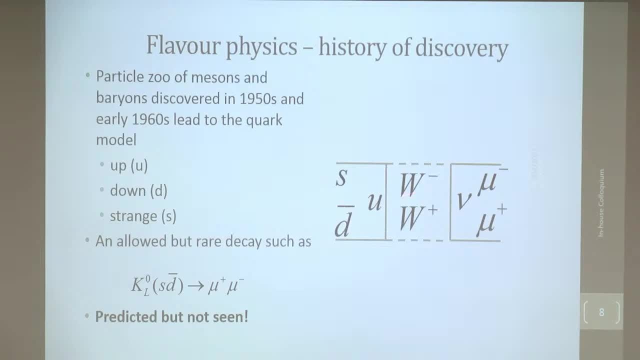 and Anti-Down Quark exchanging an Up-Quark between them, then producing two W bosons in this box here. So these particles are virtual, So they don't necessarily have to have the rest mass energies of all the particles involved here. 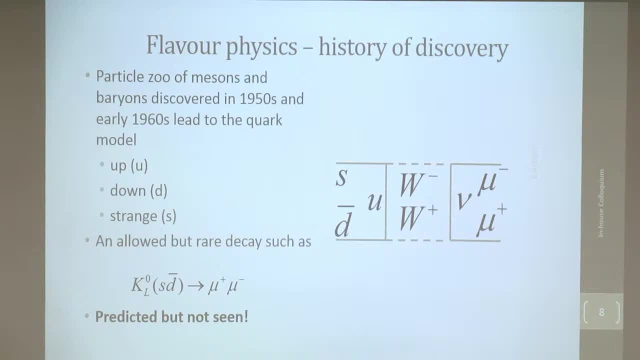 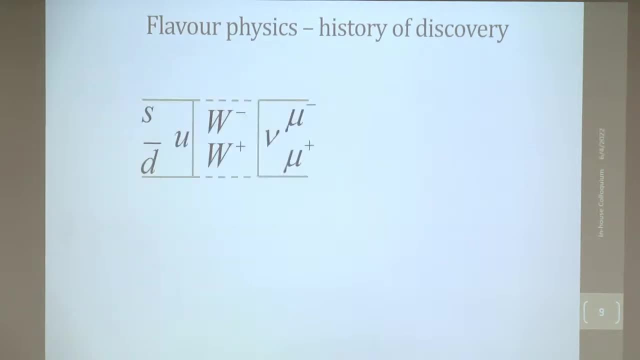 But then those Ws couple to leptons on the other side and produce your muon pair. So this was predicted, but not seen an idea of an anomaly. So how was this resolved? So these three gentlemen, Glashow, Eliopoulos and Maiani- 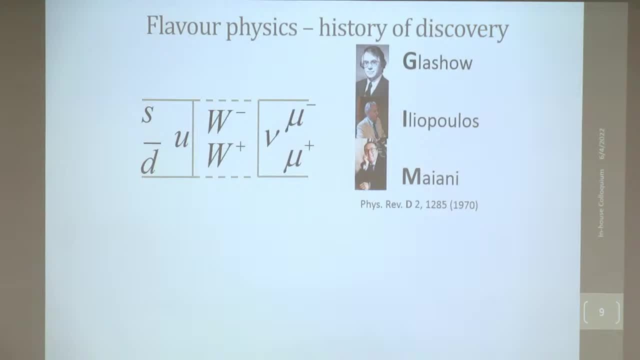 gym mechanism, as it's called. so I will tell an anecdote now. It's about time in the talk, 15 minutes in, So I heard this story- one of the many shocking stories about Donald Trump that you hear- that his staff were having a problem getting him to concentrate. 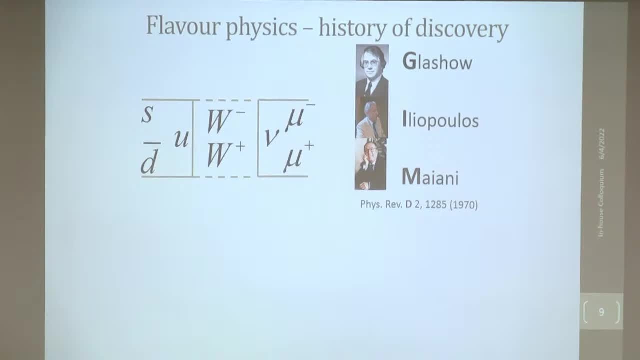 That bit is easy to believe, right. But what they found helped was they put his name into any documents. They said Donald Trump this, Donald Trump that, and he'd take an interest if it was about him. So this takes me to my second year particle physics lectures at university. 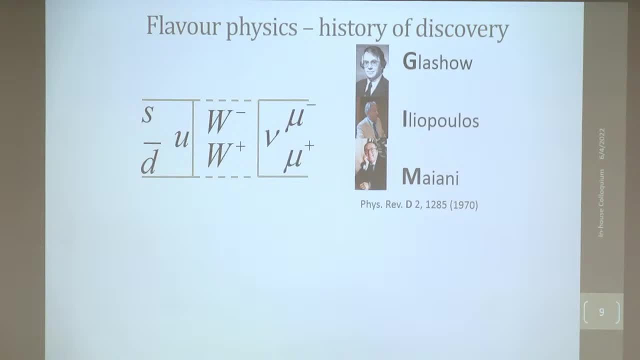 And someone somewhere mentioned the gym mechanism. I perked up, I listened, And here I am today, 30 years later, telling you about particle physics. So you know, maybe, that's probably, hopefully, the only thing I have in common with Donald Trump. 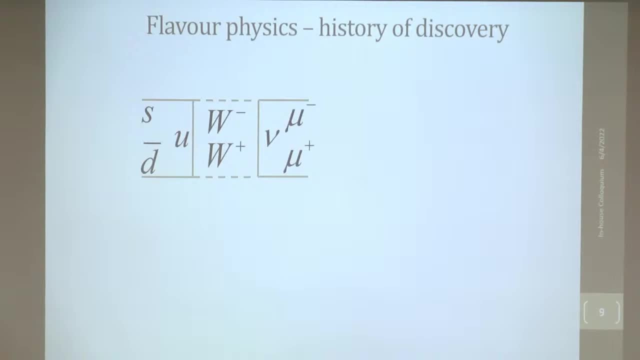 So back to the gym mechanism and my anomalous decay here. So how it was solved by Glashow and all was. they predicted a fourth quark, the charm quark, And if you put that into this box, you have these two potential ways to make this final state now. 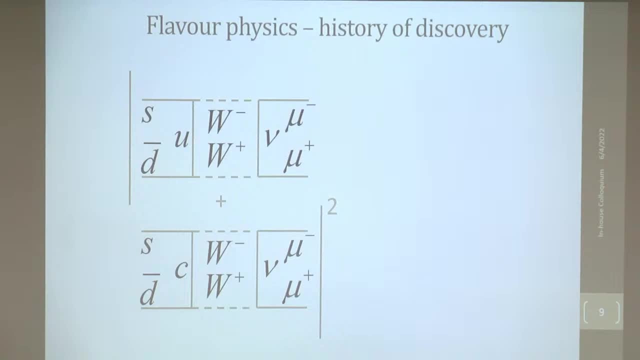 So once you sum these two probabilities together and square them, you'll get the total rate. Now, the trick was that there's this thing called the Kibibo angle, which I'll define on the next slide which comes. that varies the rate of coupling between the strange and the up quark. 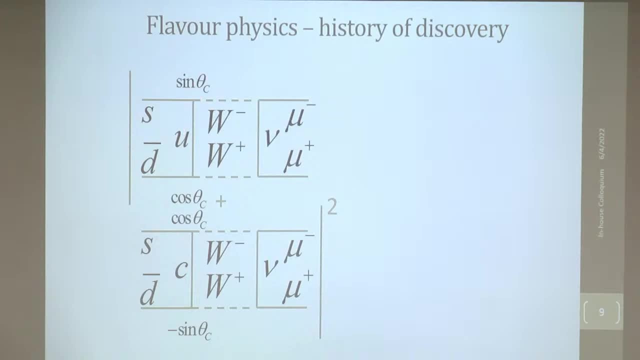 and the strange and the charm, quark and the down and the up, And what you find is that these particular things that come the lower diagram has an overall sign difference with this one. So these two diagrams end up having opposite sign. If the masses were identical it would be identically zero. 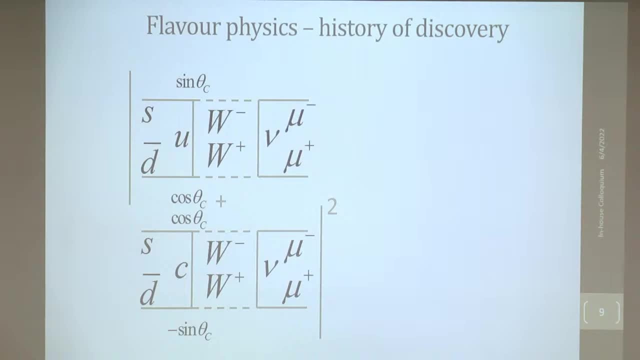 But the interference between these two diagrams is essentially suppressing the rate. So by their intuition, they realize that something else must be there to explain this anomaly that they were seeing. So eventually it was measured And the rate was measured, And the rate actually could tell you about what the mass of this charm quark was. 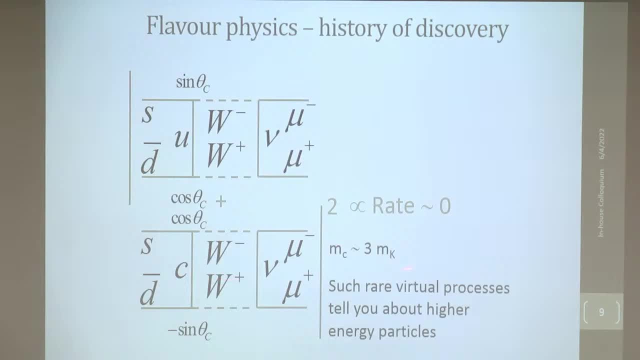 It could infer what it was. Even though the charm quark was very much heavier- three times heavier than the Kaon. they could predict it was around one and a half GeV, And then at Slack and Brookhaven they discovered it a few years later. 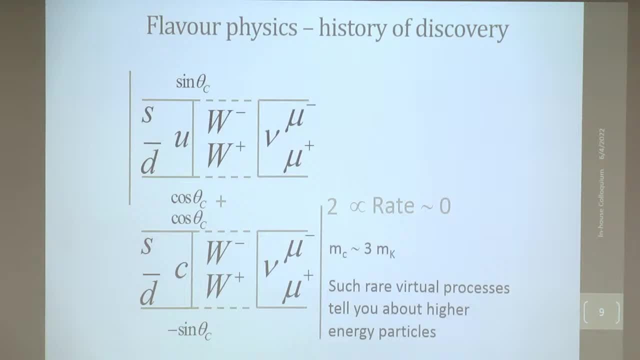 So this is what these rare virtual processes can tell us about things that we don't know about, And that's really the story that we're carrying on today is we look for these small deviations and think of ways that new physics could be changing them. 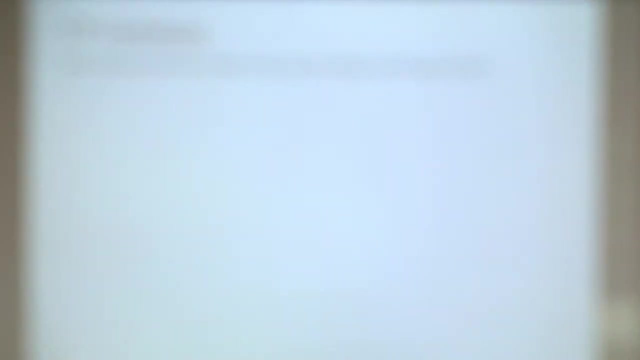 This brings me now to CP violation, which is a big theme of some of the results I'll show you, and also why Bell and Bell 2 exist. So, again, things you will have learned: Weak interaction has this odd property that it can tell the difference between left and right. 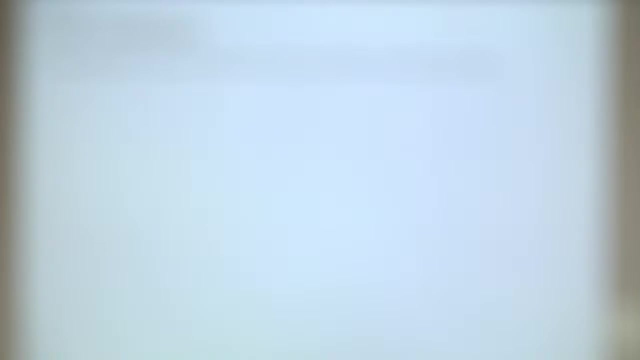 It's parity violating And that was established in the 1950s after Li and Yang predicted this by Wu. So that's most readily shown in terms of the standard model of particle physics By considering a neutrino. So this is a neutrino. moving to the right here, 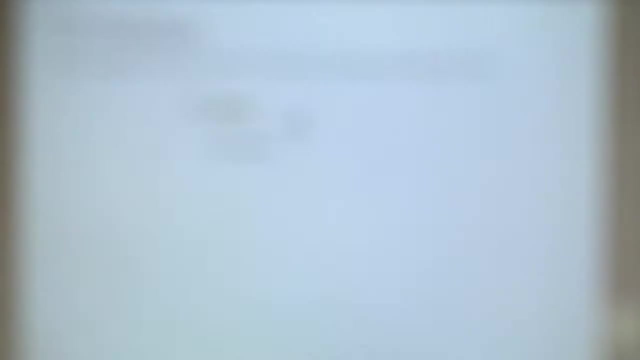 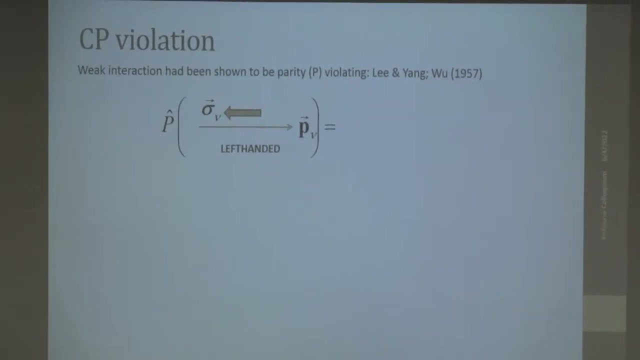 And this is its spin. And all neutrinos are left-handed. That means the spin is anti-aligned to their direction of motion. So if I operate on this with the parity operator, what I find is that the momentum changes direction. That's a regular polar vector. 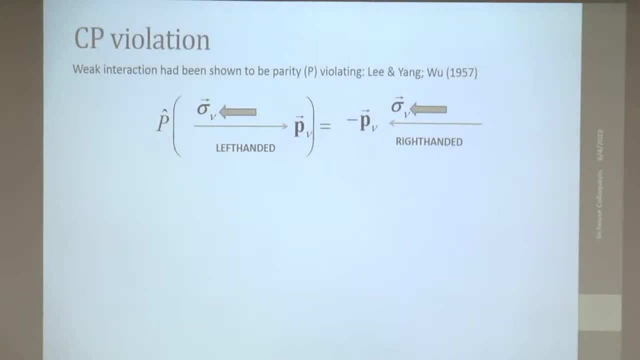 But the spin, which is analogous to the cross product of an angular momentum, cross product of a, a position and a velocity, does not. It's an axial vector. So what you end up with is a right-handed neutrino which doesn't exist. 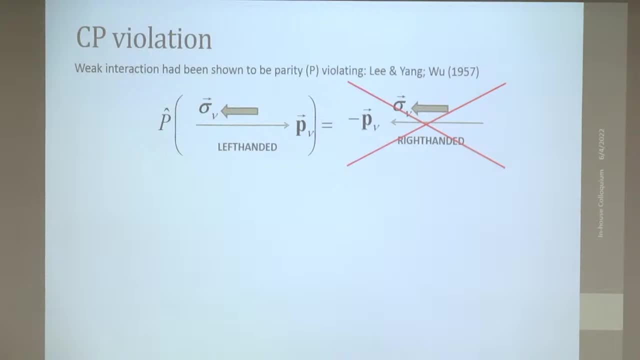 So that's a clear example of the parity violation that's there within the standard model, And it's related to the neutrino. because it's related, that's the only particle that only couples to the weak interaction. But then people thought, oh, maybe this is not so bad. 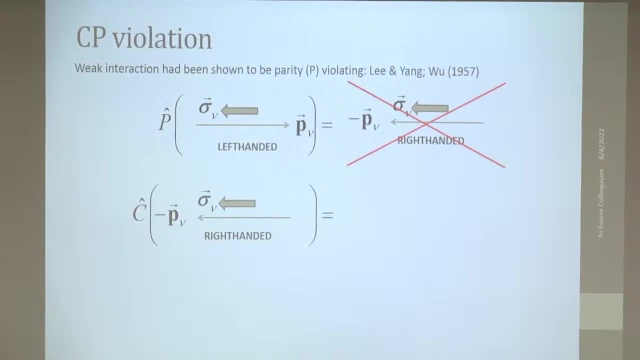 We can add charge conjugation to this. So this is this charge conjugation operator, which just converts the quantum numbers of the particle. In particular, it turns an antimatter particle into a matter particle, and vice versa. So what one gets here is an anti-neutrino. 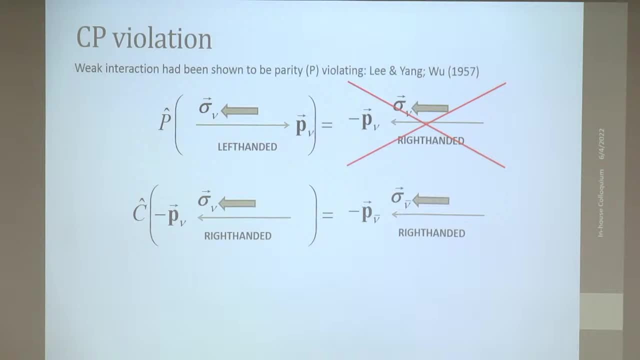 which is right-handed, and that is what we do observe in nature. So the CP transformation takes you from the neutrino to the anti-neutrino, naturally. So CP was thought to be a good symmetry of nature. But then, not so long afterwards, in 1964,. 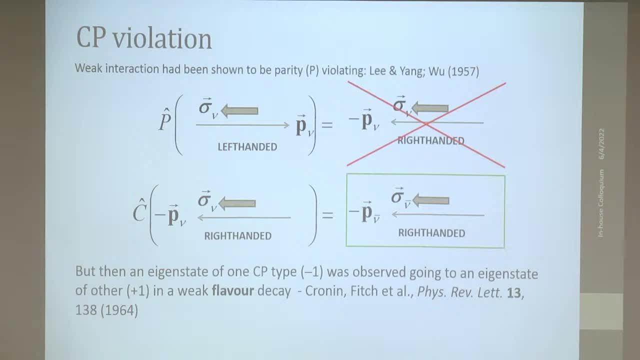 a famous experiment by Cronin and Fitch showed that you could have a known state of a certain CP decaying to something opposite, And this is CP violation: a difference between a violation of this symmetry which converts in fact, because this relates together matter and antimatter, to a difference between matter and antimatter. 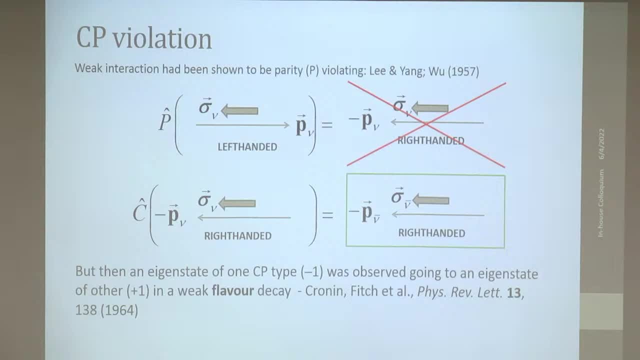 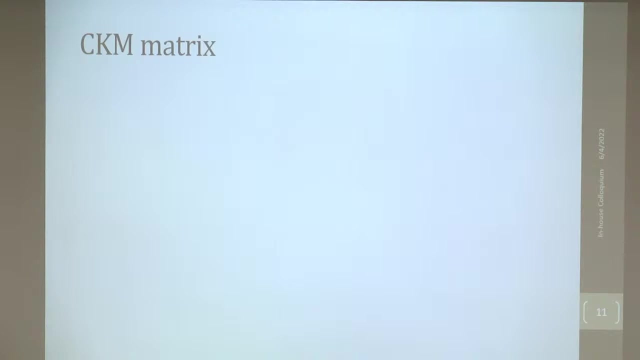 which is essential somehow to build up this imbalance that's there in the universe. Unfortunately, what we see in the standard model is nine orders of magnitude too small, so we need new sources of CP violation. So this effect was described within the standard model by another prediction in flavor physics. 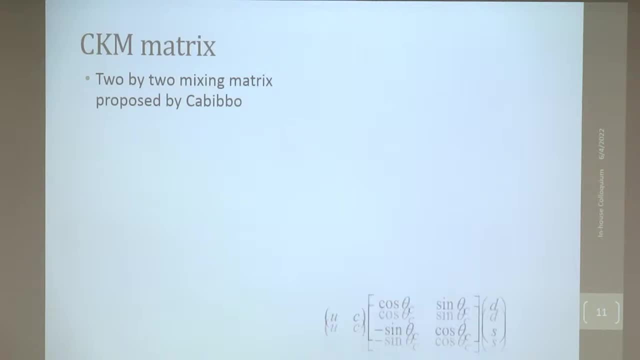 So this two-by-two mixing matrix, which I'd already talked about in terms of this Kibibo angle, is mixing together the weak interaction and the mass eigenstates, the weakly interacting eigenstates and the mass eigenstates of the down and the strange quarks, using this two-by-two unitary matrix. 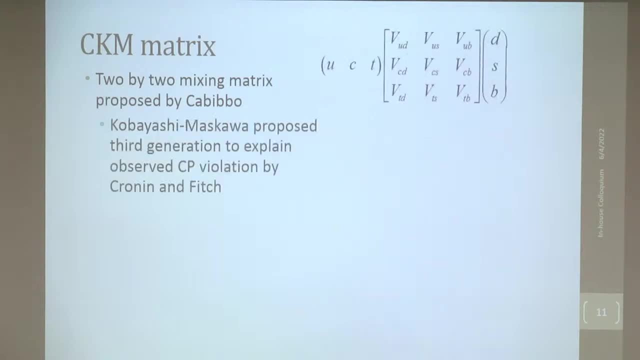 Couples to the up and the charm quarks. So what Kobayashi and Maskawa realized- this was, before we'd even discovered the charm quark- that you needed a third generation. You needed the top and the bottom quark and you extend this matrix to something called the CKM matrix. 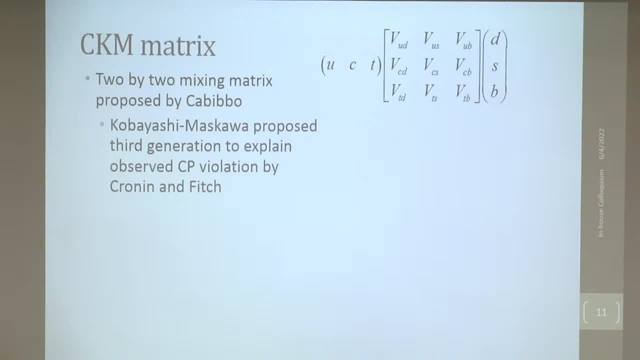 which has all these different elements. that describes the coupling between, say, the up and the beauty. quark here this VUB element, which I'll come back to And that can explain CP violation, because this unitary matrix can be described in terms of four parameters and five trivial phases. 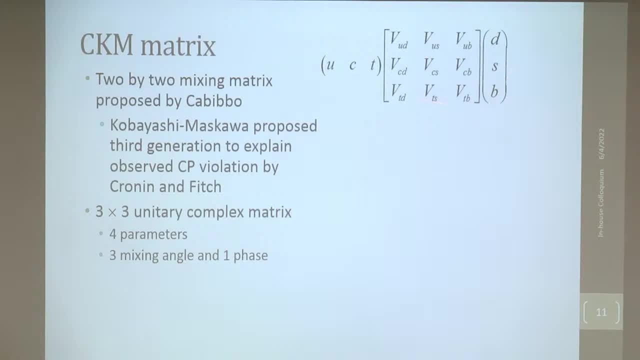 which get absorbed into these mass, These fields of the quarks. here You just need four parameters. So you have three mixing angles now, like the Kibibo angle, but you have one imaginary phase, and this imaginary phase is of different sign for matter and antimatter particles and hence can generate this CP violation. 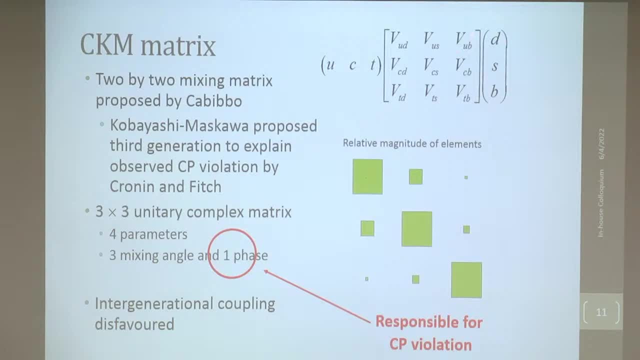 Unfortunately. why I'm saying it's so small is because this only really happens for these elements that are coupling together the third and the first generation, and you look at the magnitude of the size of these elements of this matrix. it's strongly diagonal, with only small couplings between the generations. So what this means is a up quark likes to couple. 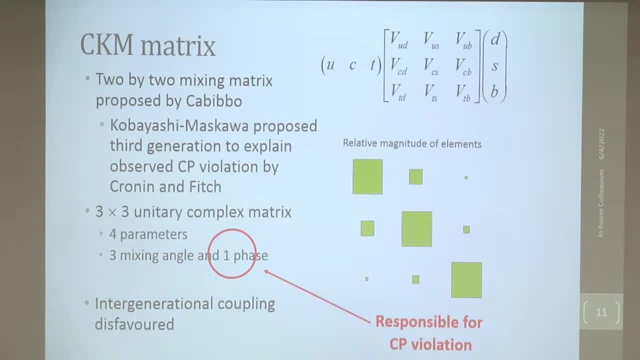 to a down quark. a top quark likes to couple to a beauty quark and it doesn't like to couple to another generation. So anyway, this CP violating phase was predicted, and they also predicted two new quarks, which turned out to be discovered many years later. So this is again an example. 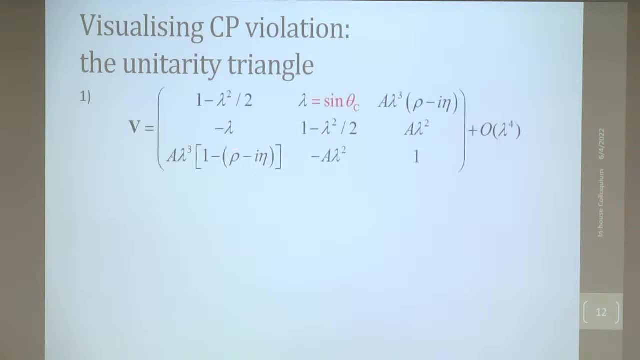 of flavor predicting. So I want to talk a little bit more about the CP violation now. and we look at this CKM matrix in a particular expansion, so-called Wolfenstein parameterization, where we expand in powers lambda, which is just sine of this Kibibo angle. 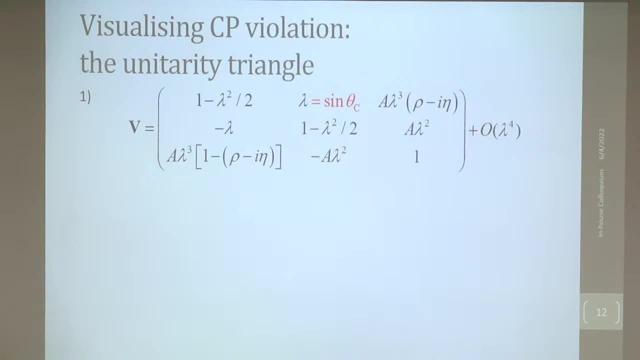 and there are terms up here which are higher order, which we won't worry about. And you see these complex numbers here, as I said, they're the ones between the first and the third generation, VUB and VTD, Which contain information about the complex phase. 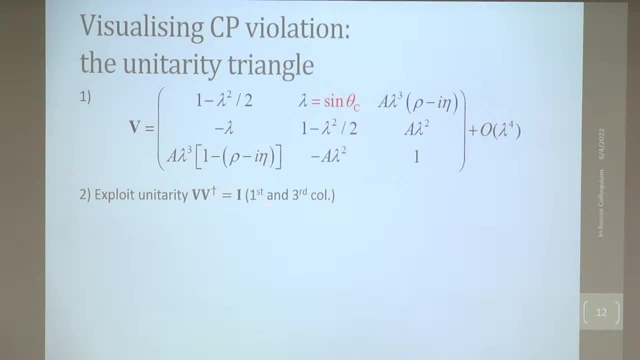 So you exploit unitarity of this matrix. you have to conserve the number of quarks, and in particular one looks at the first and the third columns, And here you write down a relationship between the element and the charge conjugate of another. and because these must be, 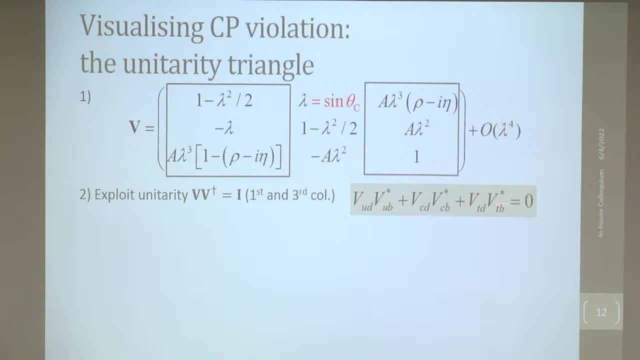 the zero terms in our identity matrix. they're the three imaginary numbers which sum to zero. So in the Argan plane, this is just a triangle and this is just a triangle, and this is just a triangle and this is just a triangle. 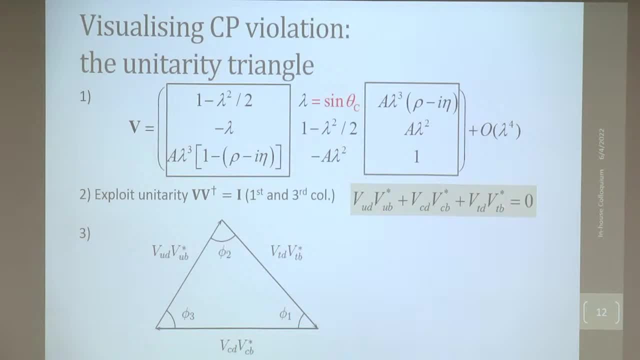 so each of these components on the left-hand side of this expression can be viewed as a vector in the Argan diagram and they must close together to give zero, And this is the so-called unitarity triangle, which is the way that we visualize the amount of CP violation in the standard model. 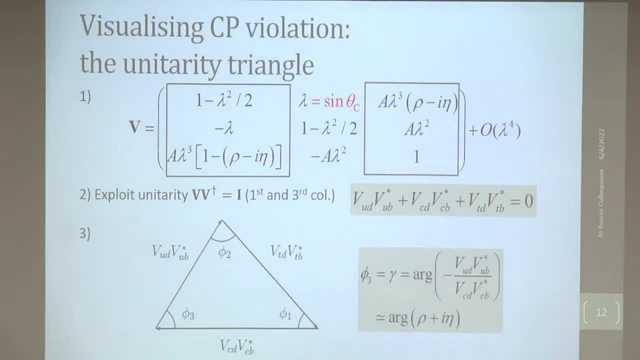 Now, this means that we can measure the angles of these triangles and measure the length of the size, and we can over-constrain or look at the length of the triangle and we can measure the length of the triangle and we can over-constrain or look at the length of the triangle and we can. 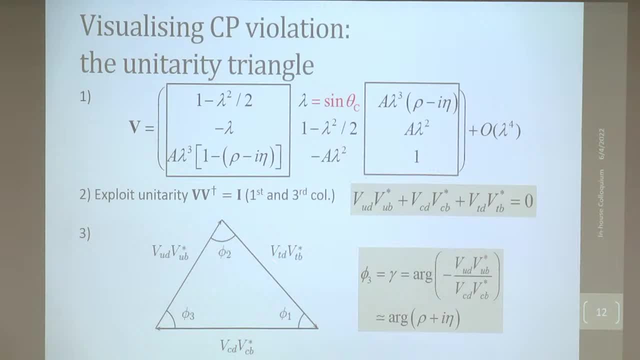 look in great detail at what's going on with CP violation. There's a bit of confusion in our field. Some people like to call these angles phi 1,, phi 2, and phi 3.. Other people like to call them alpha, beta and gamma, And if you work for a Japanese experiment, you're expected to call 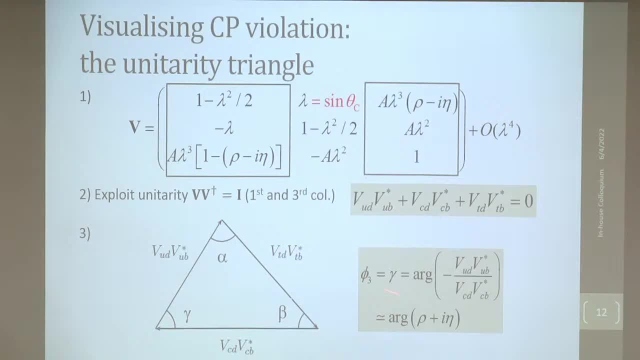 them phi, because the Japanese like to call them that. But you can see how you can get these angles by looking at the ratios of the sides and you can get the arguments and you can see how they're related back to this parameterization. So a lot of effort went on over the recent years. 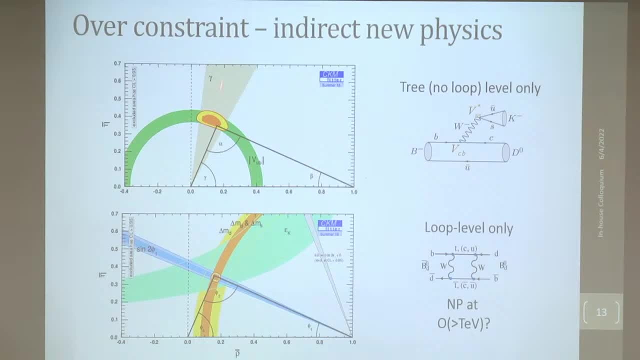 to try and measure this triangle very precisely And these are the current results, but again gives the indication of why we want to measure these things better. So this is the current knowledge of the unitarity triangle by just measuring things where you don't have any loops. 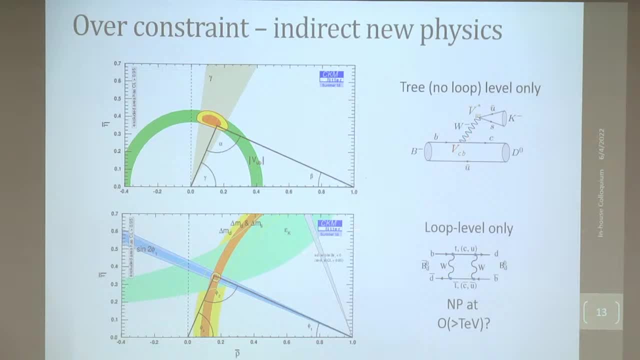 what we call tree diagrams. So I'll come back to this later. But you can compare it to where you have loops And, as I've mentioned before with K0, mu, mu loops tend to give you new things because you can have heavy new particles in these loops which you haven't actually directly. 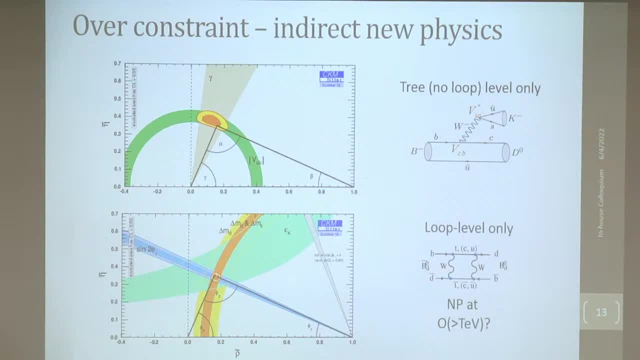 produced in the laboratory before. So you can actually see that the apex of this triangle, which is telling you about the amount of CP violation. if this triangle had zero area, there'd be no CP violation. It's not well known directly. We have to rely on all these loop. 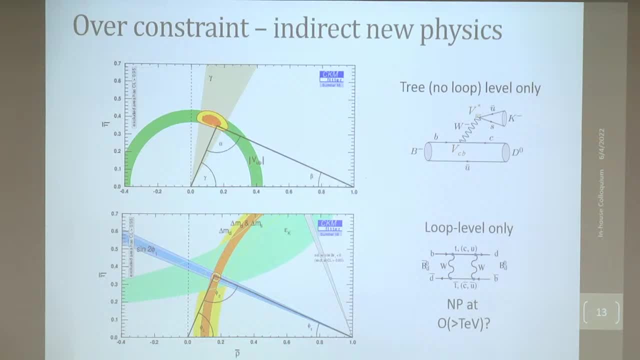 measurements. So what we're trying to do is improve the measurements here to see if there's any tension between these two. And there is scope for considerable tension between these A few degrees difference in the measurements of these angles. So again, 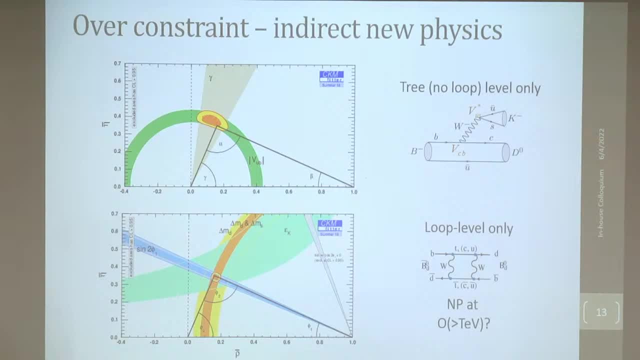 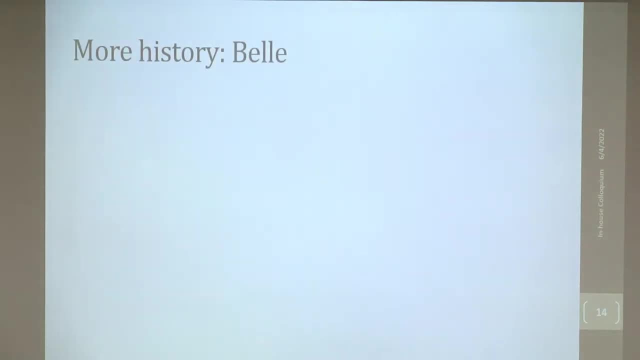 this is an example of these kind of precision measurements that we're trying to do, which may tell us something about other sources of CP violation beyond the standard model. Okay, So before moving to bell two, I must say something about I have a paper in the spot. 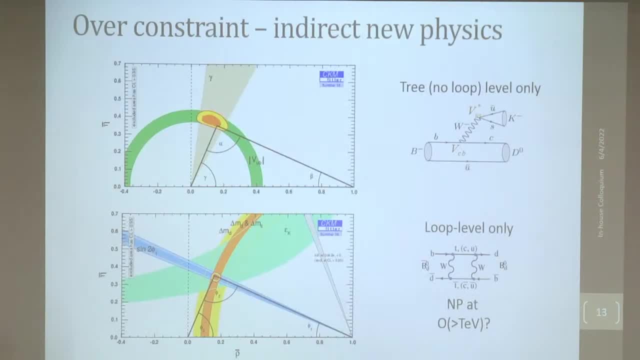 On the standard model theories like to say there's no new CP violation because it makes life difficult for them for other Other observations. So most people favor that the new CP violation is there in the neutrino sector. So there's this equivalent matrix, this PMNS matrix, which could, if that has 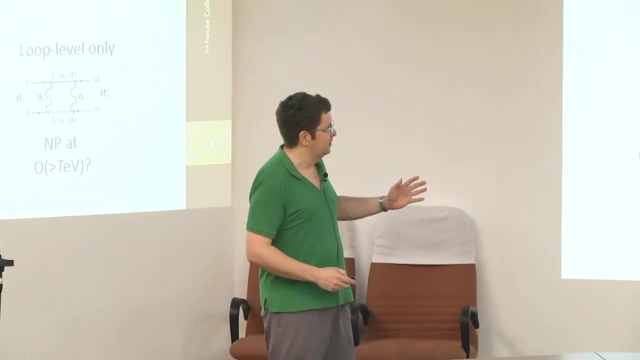 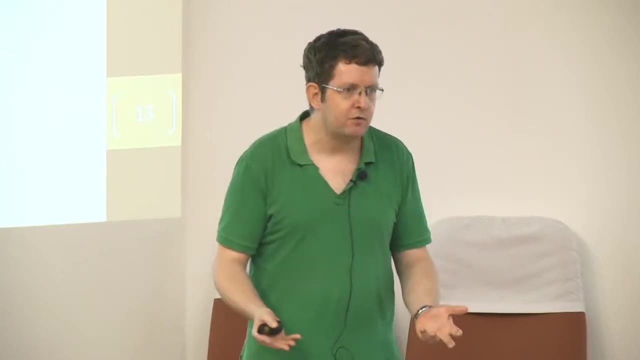 CP violation in. it could explain things. But if we have a new theory, if our current theory already has this mixing between the quarks, there should be new sources of CP violation. You can continually add phases if you've got a three-by-three. 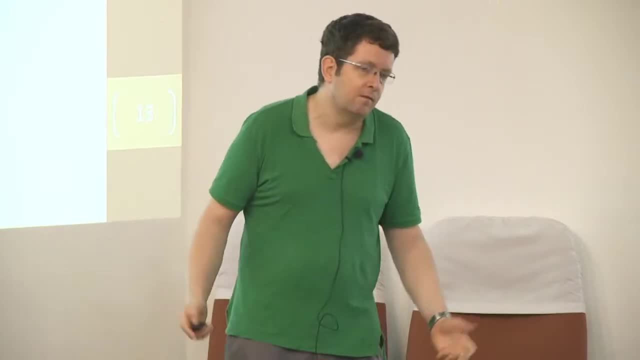 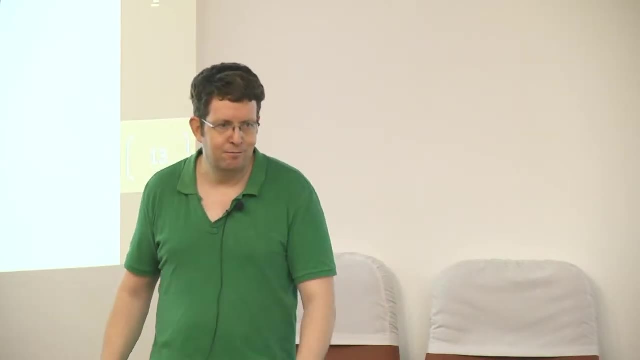 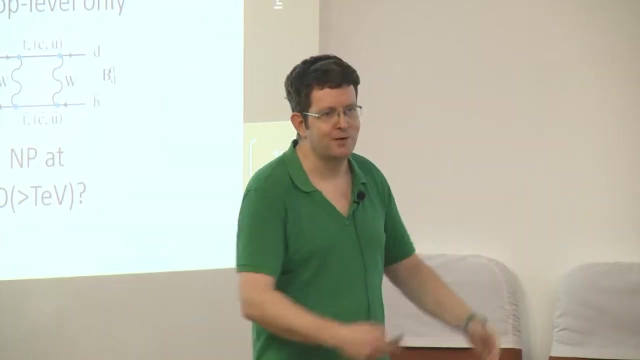 Or four-by-four structure that some of these things have. So there's prejudice one way or the other, if you like one theory, Some people like an extra generation, Some people like supersymmetry and no CP violation. We have to measure it. 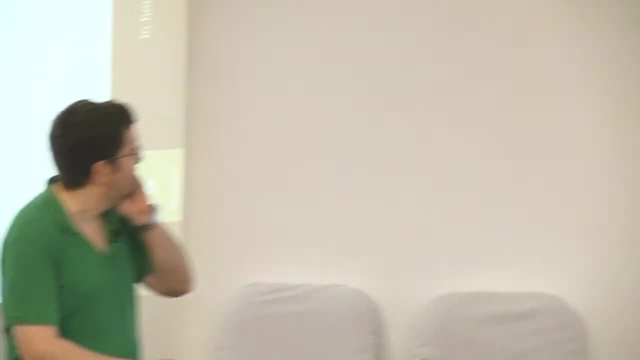 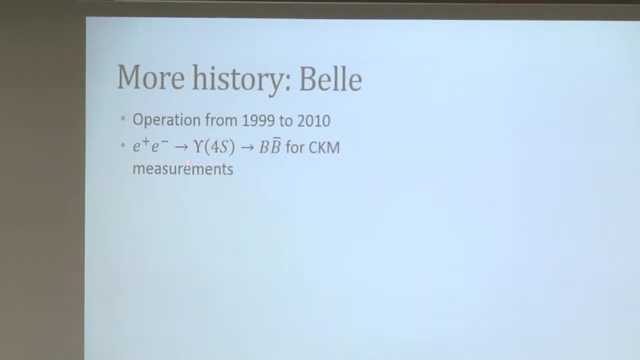 So what this is is an experiment that collides together electrons and positrons. The E plus is the positron, the antimatter electron At a particular resonance called the epsilon 4s, which contains a beauty quark and an anti-beauty. 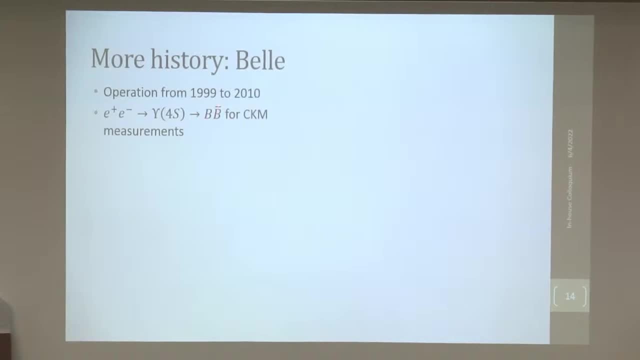 quark, And this declares almost exclusively to a pair of B mesons, which is a B quark and a light quark. So either a B minus, which would be a B quark and an anti-up quark, or a B0 bar, which is a B quark and an anti-down quark, And we use these primarily for measurements. of CKM and also to search for the B quark, And we use these primarily for measurements of CKM. and also to search for the B quark. And we use these primarily for measurements of CKM. and also to search for the B quark. And we use these primarily for measurements. 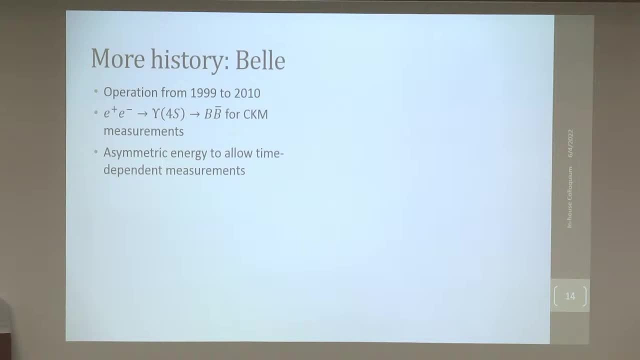 for rare decays. I didn't write that here. It has a special feature that there's an asymmetric energy between the electron and the positron. The electron is faster than the positron and that boosts the center of mass frame. So these B mesons are moving in our lab frame And because of this and because they have 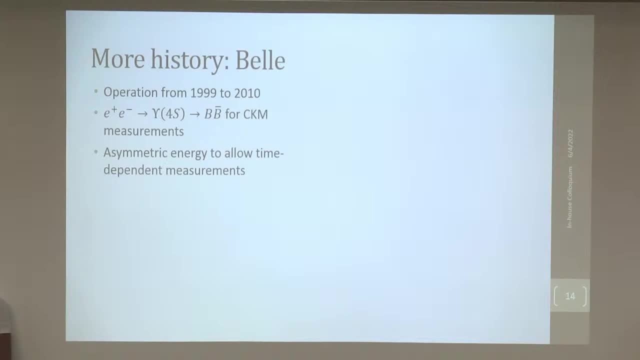 a relatively long lifetime of 1.2 picoseconds, which doesn't sound very long, but that means that they travel a macroscopic distance which we can measure before they decay For when they're produced, Whereas something that's decaying strongly will have a lifetime. 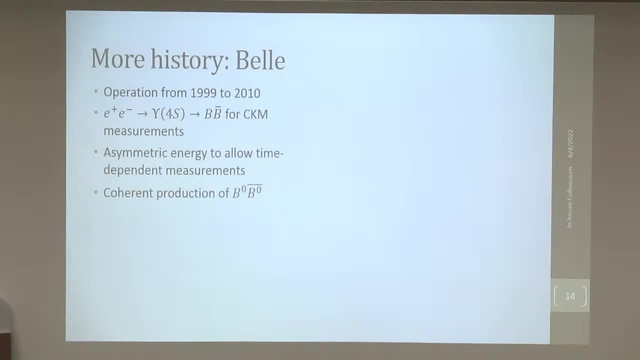 of 10 to the minus 20 seconds or so, So we can exploit this and it allows us to make time dependent measurements. Again, I won't go into the details of this because I'm not showing any of that today. I won't talk about coherent production, But this: E plus, E minus. 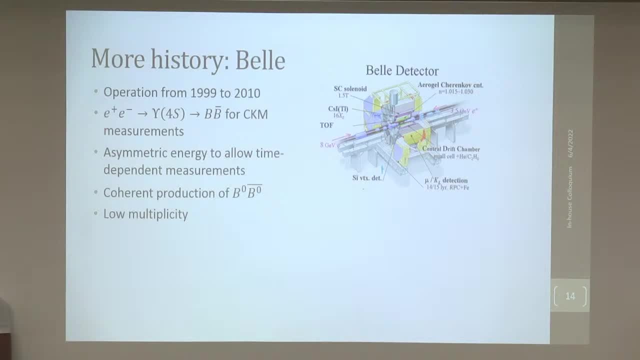 environment is important to understand why we're not doing some of this at the LHC. When you bang together protons, you get lots and lots of particles. When you bang together electrons and positrons at low energy, you get here. And when you bang together protons, 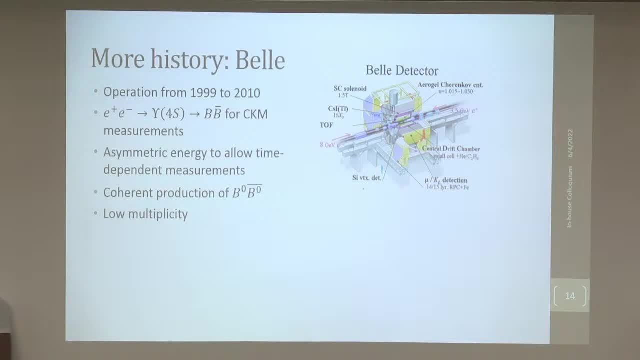 low energy. this is only 10 GV compared with 13 TV. you get very few. on average we get between 8 to 10 particles. it means that we can do very precise reconstruction. we can reconstruct everything and even measure the missing particles like neutrinos. so so belt 2 runs with 7 and 4 GV for the electron. 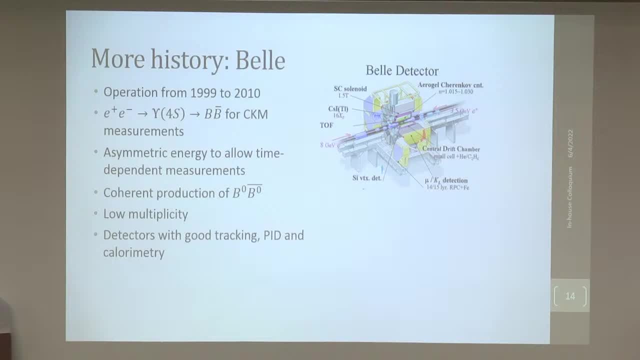 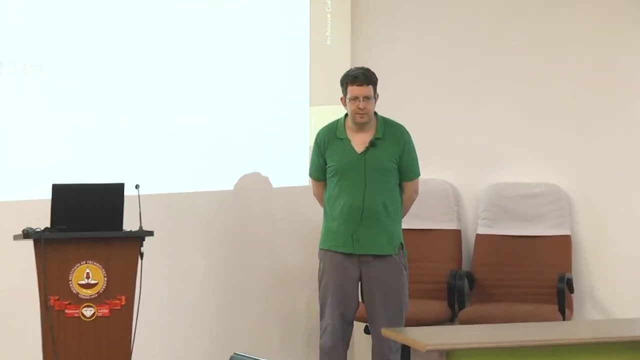 positron respectively. so I know no two separate beam pipes, so it's a separate lattice for each one magnetic lattice, all right. so if it for the weekend interaction, because the strength of the coupling is so small, so any it's I collect, it's like QED, right. so it's QED actually. suppress further because of the. 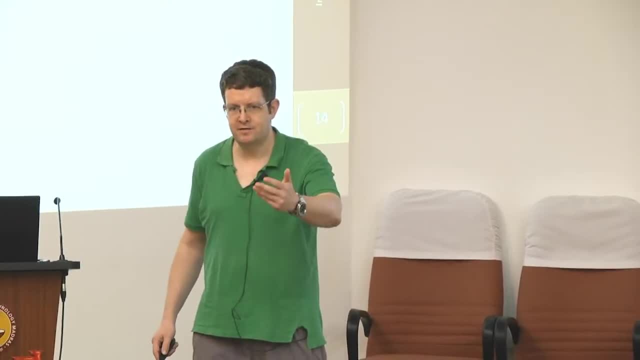 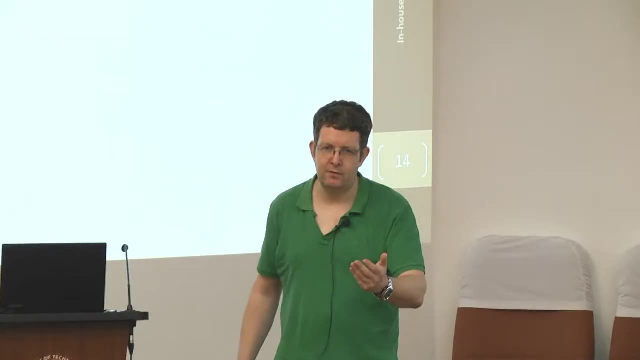 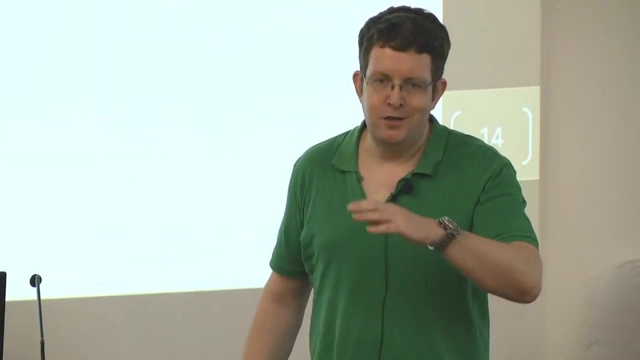 mass of the W. so so higher-order weak corrections are essentially negligible. higher-order electromagnetic corrections: you can start to worry about those in certain processes. we do worry about alpha, QED squared type corrections for the strong interaction. you're screwed right because alpha S is of order one. 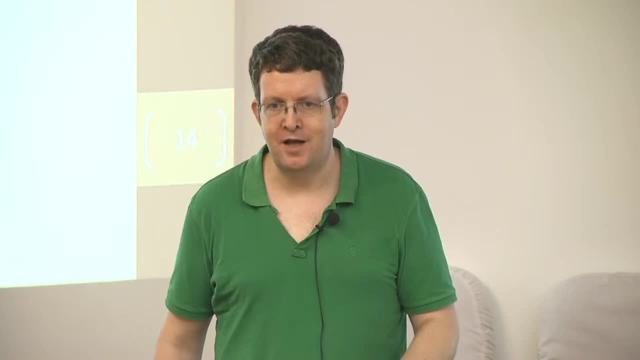 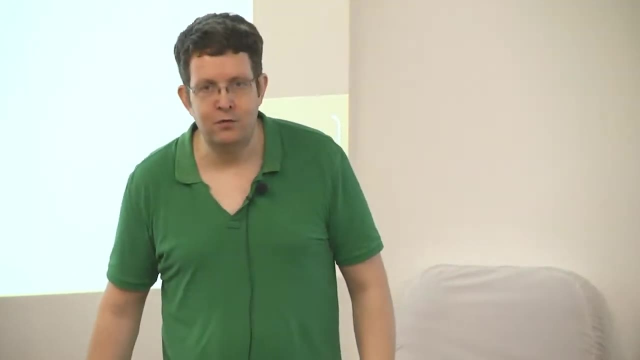 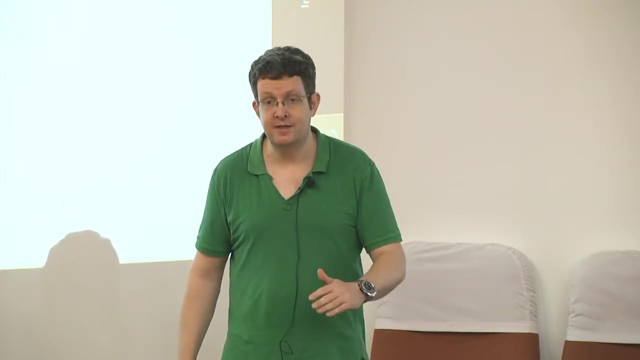 particularly at low momentum transfer. and then you have to sum to all orders and you can't actually make the term perturbative expansion. so QCD is a problem in many of the measurements that we have, because it's hard to predict. so we devise ways to measure the relevant parameters and essentially have them as 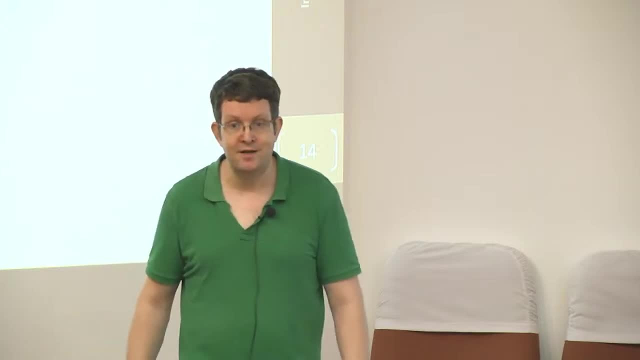 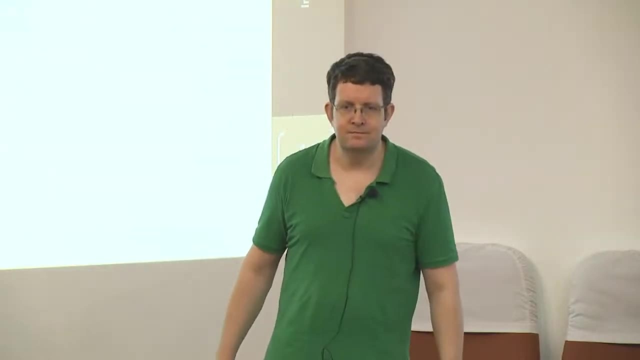 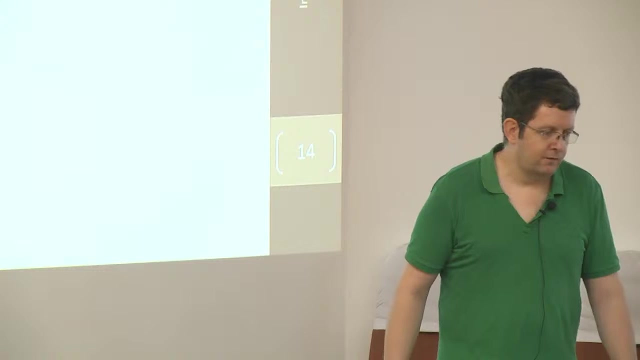 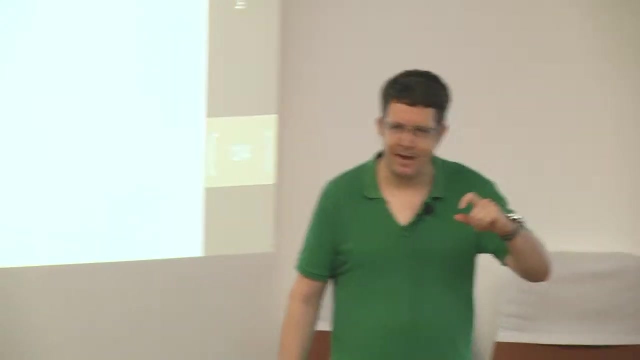 nuisance parameters and extract them in our fits, because we don't, we, we don't want to be reliant on calculations. so so those for extracting certain things from B physics, particularly the magnitudes of the CKM, matrix elements, VUB and VCB in particular, we rely on. 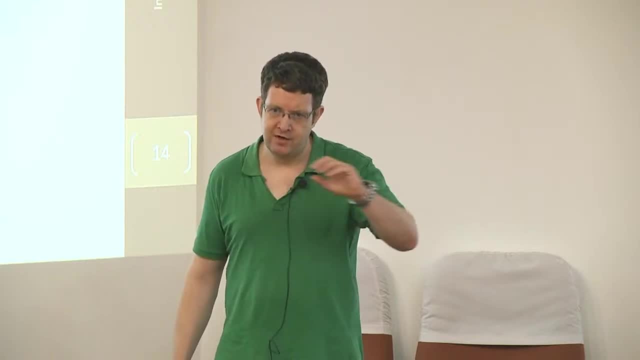 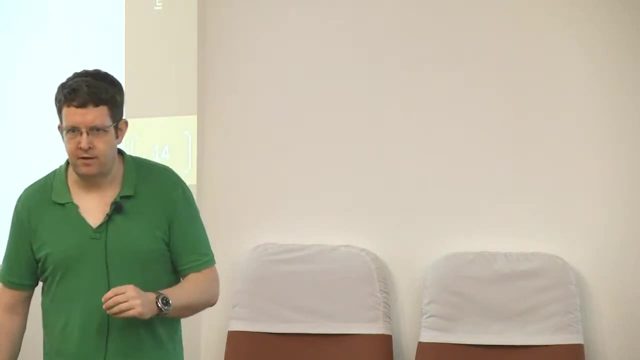 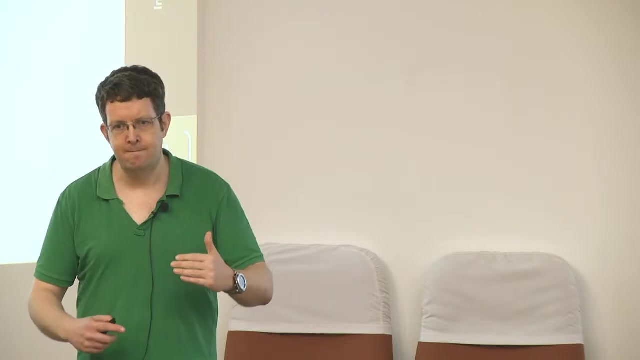 precise calculations of the form factors of the B, transitioning into a lighter meson, which can be done on the lattice. however, there is great distrust of the lattice because it's very hard, and so we have to find ways of calibrating the lattice as well. so there is, there's no, not, I say. 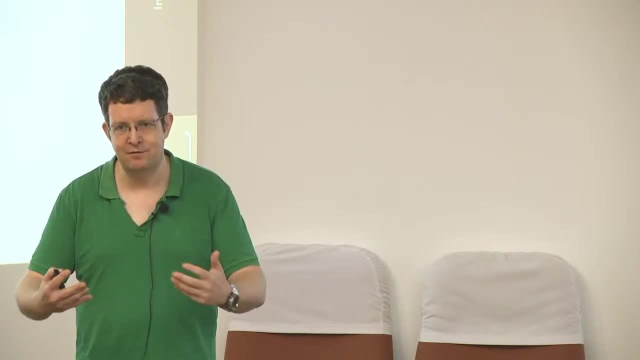 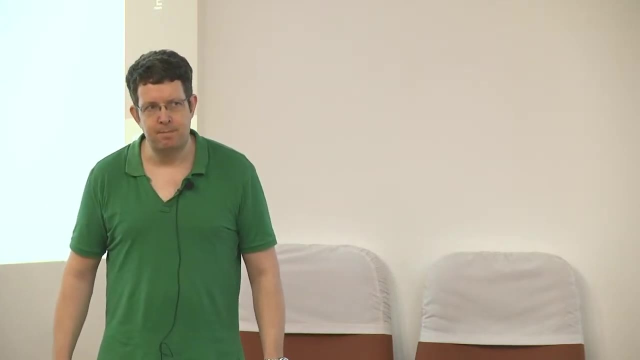 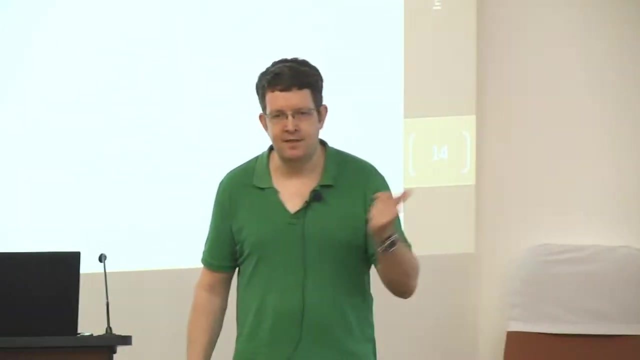 distrust. it's because these calculations are so intensive computationally and to discretize space and time more and more it's incredibly difficult and but. but they're improving all the time and we hope to get a few percent precision based upon lattice calculations on the length of the site. but again, that's. 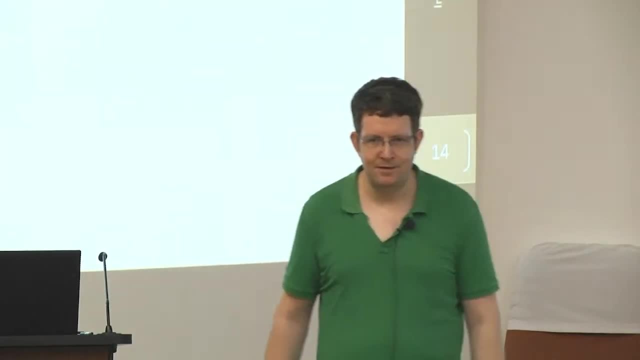 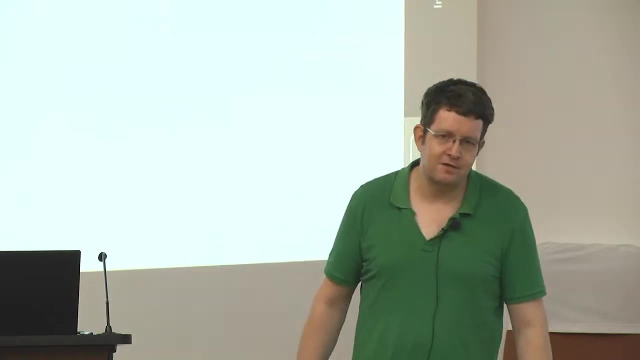 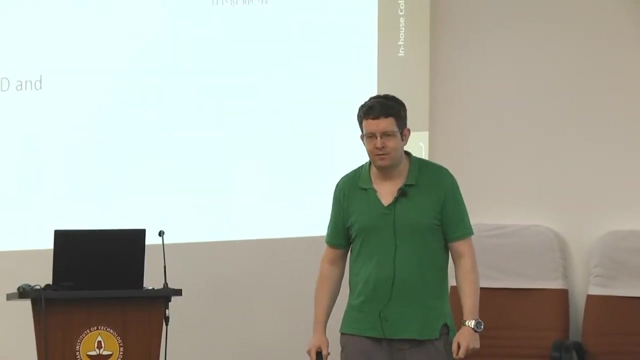 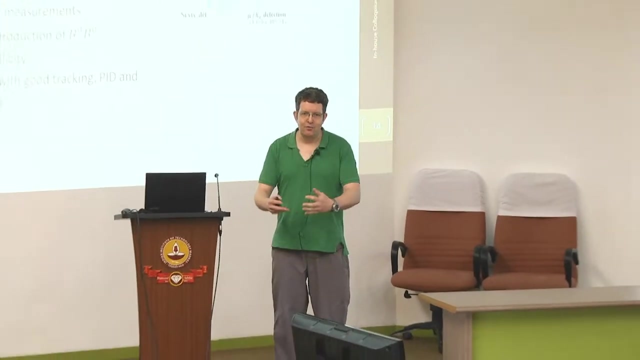 not coming later. there are Benicio calculations, which basically they discretize this lattice right, and then how they actually do the calculations. I'm not the right person, but some of it will be Monte Carlo integration, some of it will be analytic and it's a combination of these and I know there are things that have problems. 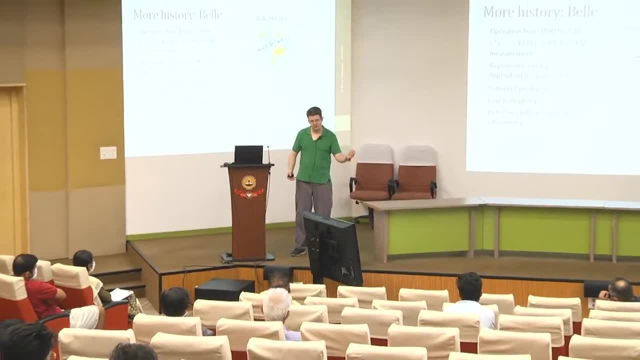 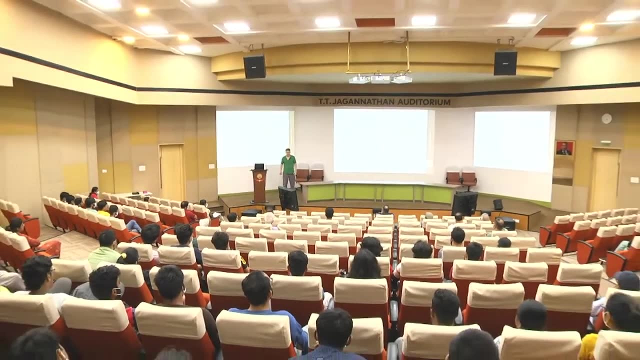 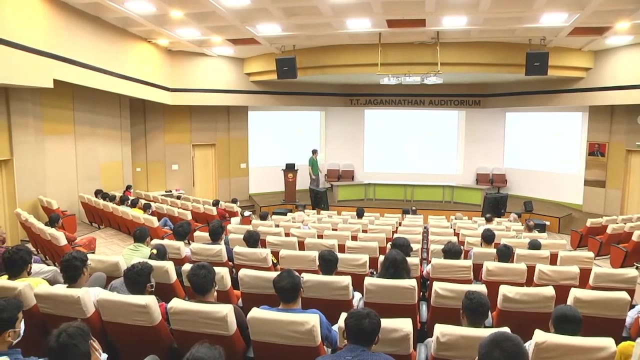 with. they have to do it all with certain masses and then extrapolate and to the real mass is later on, because you have to do it in a chiral way where things essentially zero mass. it's a minefield. but we should get someone to come and speak about lattice QCD because it's a very interesting topic, okay, uh. 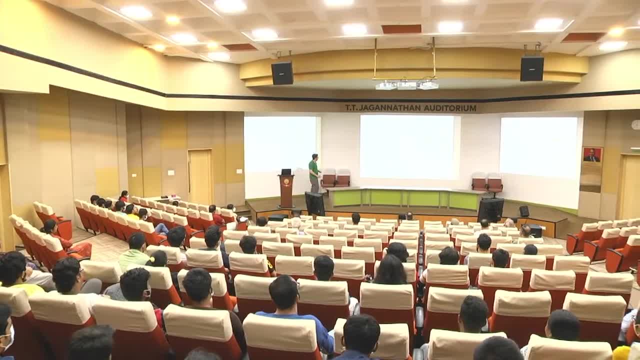 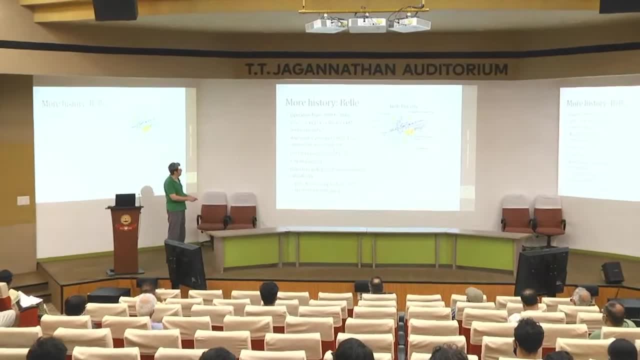 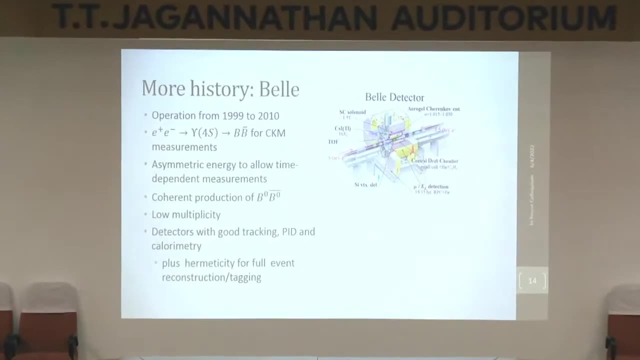 it's. I think I'm doing okay. yeah, I'm about halfway through and halfway through the time. so, yeah, going back to this clean environment, we have this detector up here, which is the Bell detector, which encloses where the particles collide in here, and then we have these sort of cylindrical layers which measure. 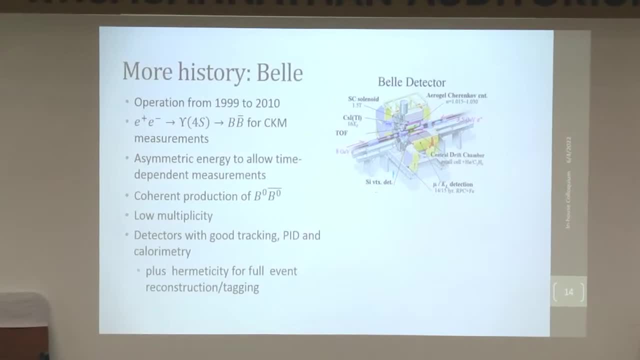 different properties of the particles. so there are some that measure that where they decay very precisely. some measure the momentum, others manage, measure the electromagnetic energy and then if, if a particle escapes, the whole thing, it's likely to be a charged particle, that is, it's likely to be a muon. so you have. 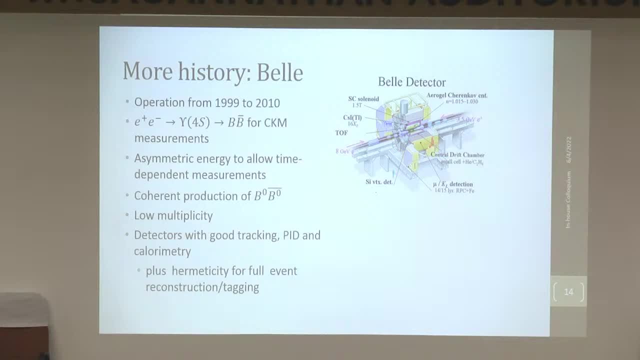 muons outside and we have specialized detectors to tell the difference between pions and kaons by PID here. so these experiments, there was Bell. there was also Babar in America. they had problems with their accelerator and they didn't accumulate as much data as Bell and they stopped somewhat earlier here in 2008. 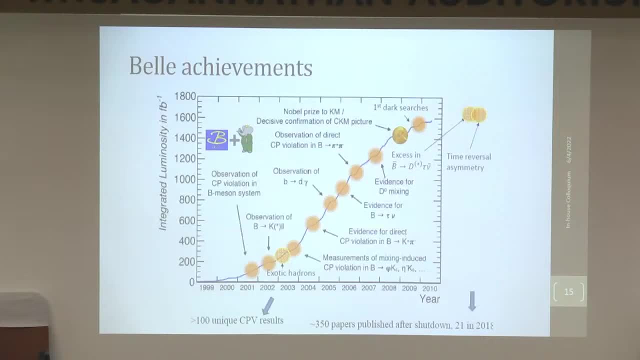 whereas Bell went on to 2010 with this data. they did several things. I can't go through all of this. I want to highlight this Nobel Prize up here, which was for Kobayashi and Muskawa, because we measured the triangle very precisely and showed that their description of CP violation in the standard model was 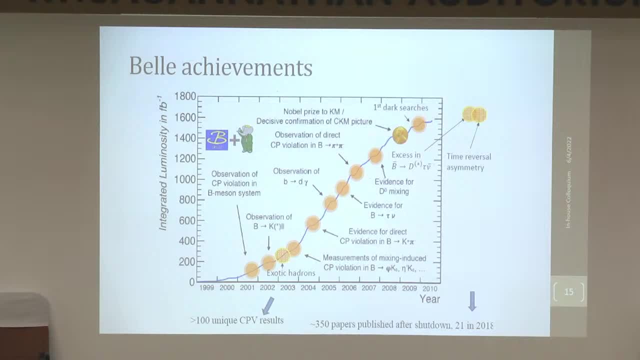 correct. and then this is give you an example of the diversity of the measurements that we make. and then I want to talk about anomalies a bit later, and one of these is the success in this B decay to a charm mise on a tau and a muon, and this is what's causing some excitement in flavor physics, in. 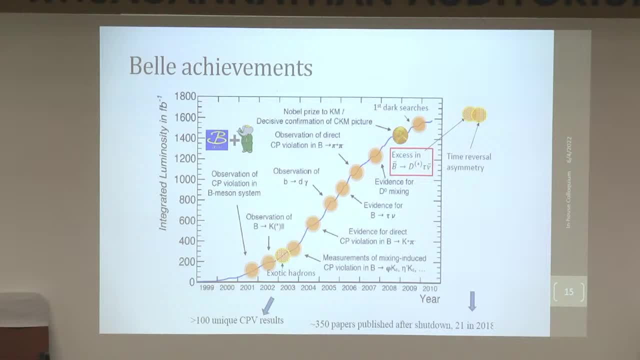 particular and part of it in general today. so, and then just to go back to things, I said earlier that we can even search for light, dark matter in our collisions and things, and this is what these first searches were done and we're going to make them much more precisely at Bell 2. 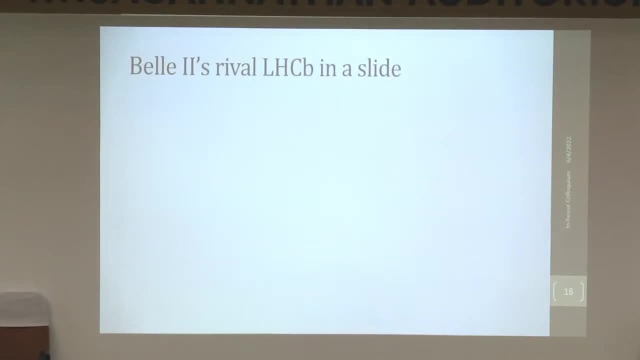 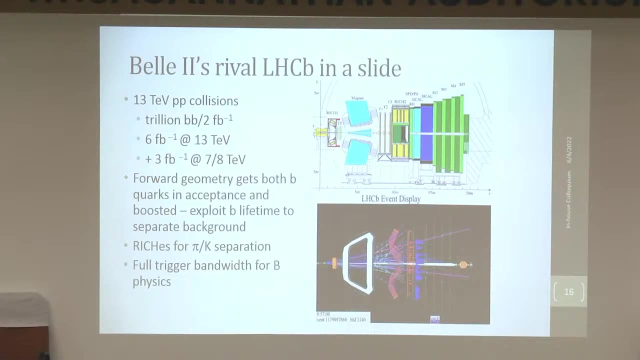 so to put in context Bell 2, I just wanted to spend a little bit on LHCb. I won't go into detail on this. this is an experiment at the, obviously at the LHC, which is collides together its protons here and then it. 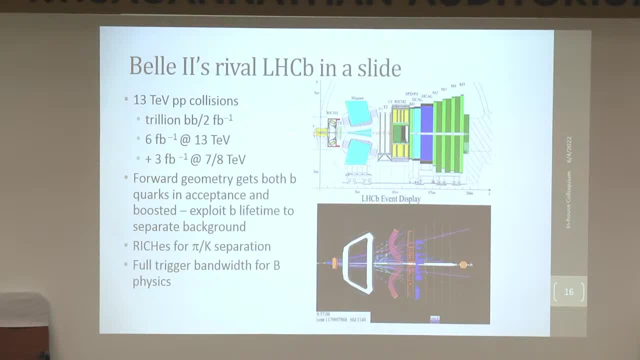 instruments, a small forward region, as everything is boosted into their acceptance. and this is because the pieces of the proton that collide, which are essentially the gluons, have differing momentums whether they're traveling from the left or the right, and so they're always boosted in some way. 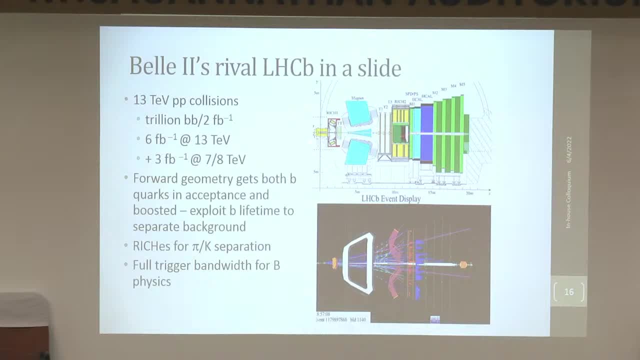 and and by doing this you often get both b quarks in the acceptance and they can make measurements and they have all the same things. they have precise tracking, particle identification, muon detectors and tracking and into measurement and they have been very successful in the last decade. they've 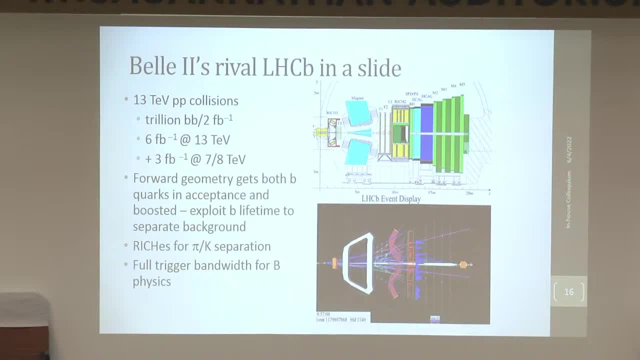 trillions of be mesons compared with the billions I'm going to talking about. so they have a huge statistical advantage. but there they have issues in that they collide together things at 40 megahertz but you can only read this out at a few kilohertz, so they lose a lot of data. this will change in their upgrade. they're. 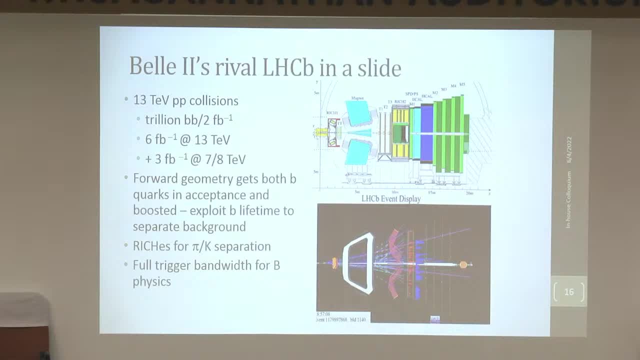 going to try and read everything out at 40 megahertz, but they've been very, very successful. they are the ones who've discovered some of the anomalies. they've discovered many new particles- spectroscopy- these are new states of bound quarks and they've made the most precise measurements of the unitarity. 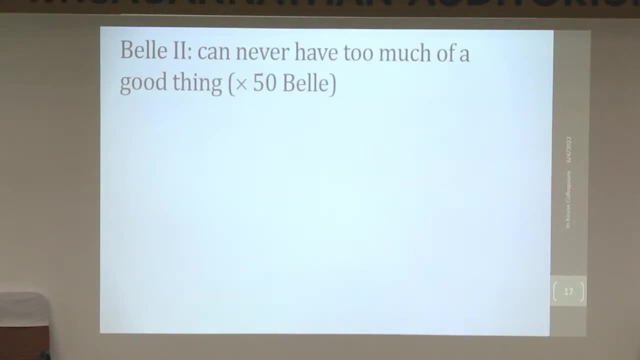 triangle now, so we're trying to play catch-up, but all too, in essence is, you can't have too much of a good thing. Bell was very successful leading to this Nobel Prize for km, so we're trying to integrate a data sample 50 times larger so we can make more precise measurements and also search for. 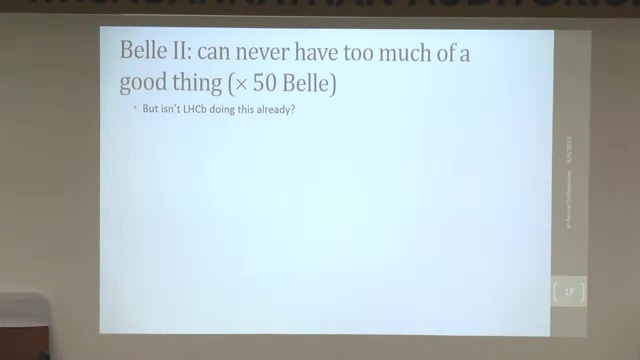 rarer and rarer decays. But you must ask yourself: if there are trillion bees in Geneva, why are you trying to do this in Japan? So in this big table here, I'm trying to show the complementarity between these two experiments. 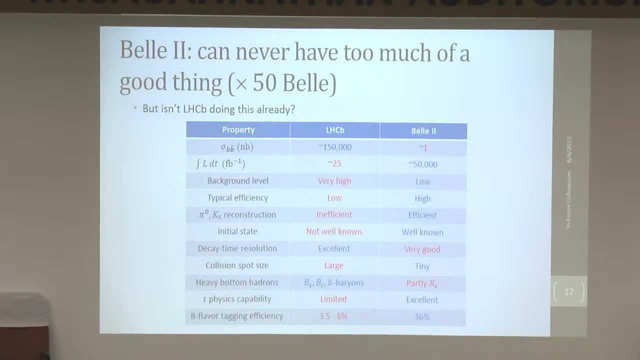 A lot of these terms are a little technical. One thing you can see is that we're trying to greatly increase our luminosity here, But we don't. LHCb doesn't have to do that because they have a huge cross section which 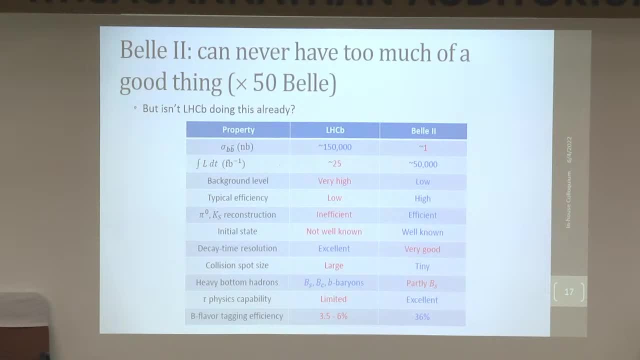 is 150,000 times larger than for producing bb-bar pairs, But we have this low background level. We have very good reconstruction of neutral particles, particularly a pi 0, which decays to two photons- This LHCb event, which I didn't talk about here. 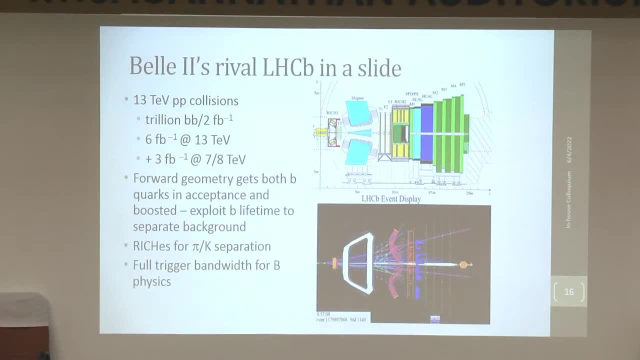 you see how messy it is. There are tens of particles coming out here And it's quite hard, And all these clusters in the calorimeter. it's very hard to reconstruct things unless, like here, there's a pair of muons. 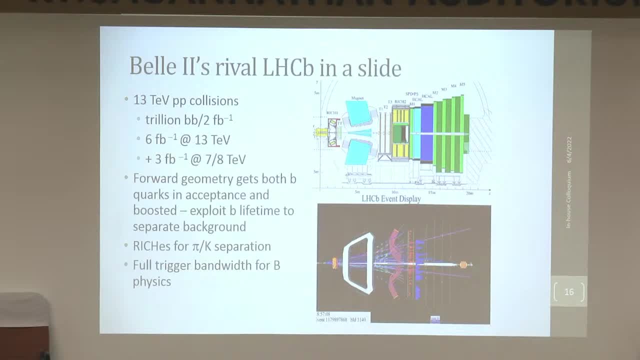 that you can see clearly which are coming from a b-medium. They can do this well if it's fully reconstructed, So if it's all charged tracks, that boost is enormous. So it actually flies like a centimeter or so before it decays. 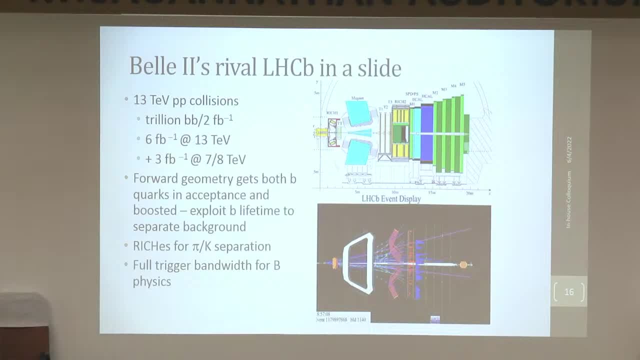 And they have a very precise silicon detector And they can see very clearly the decay point And that gets rid of a lot of the background that's coming from the underlying proton-proton collision. But as soon as you've got a neutrino or a pi 0,, 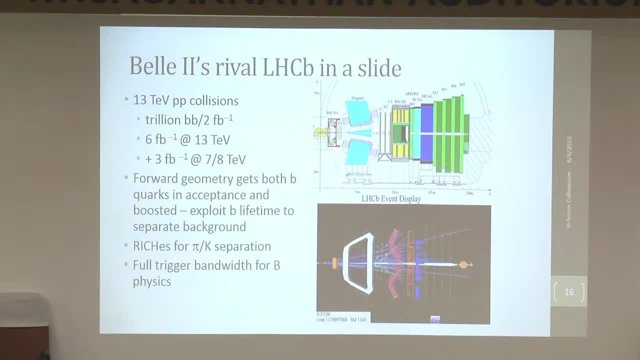 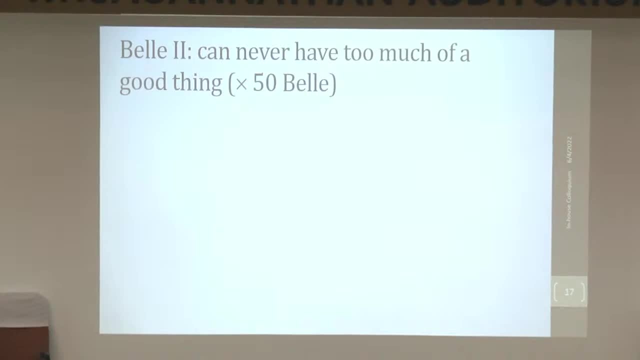 they have lots of problems. They are making nice measurements using those modes, But in principle we should do them better. That's really coming back to our strengths. We have this well-known kinematic, so we can measure the neutrino And we can measure these neutrals. 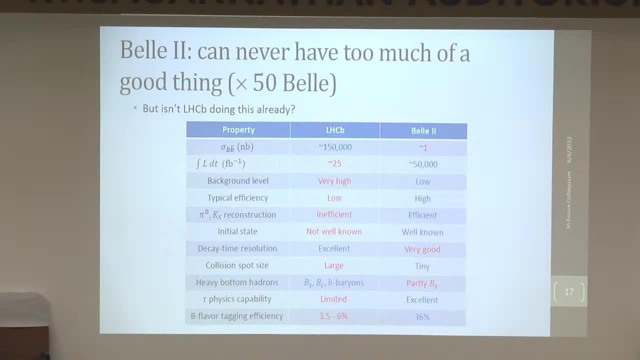 And something again I won't talk about. When you produce b quarks, you're also producing lots of tau leptons And you're also producing lots of charmed particles as well, And there's lots of interesting physics you can do with those. 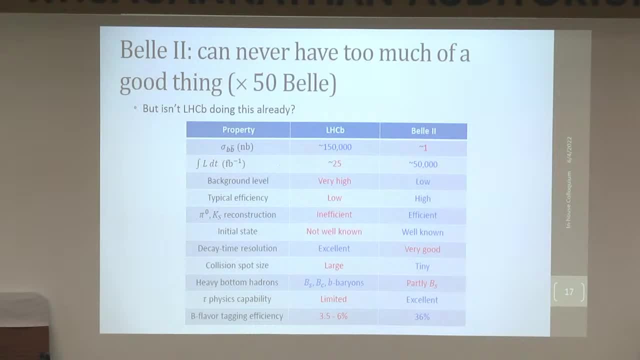 I'll show one result from charm. So you have many different things that you can do, So these complement each other. So for things with all charged tracks, LHCb will always lead the way. They're going to run through into the 2030s. 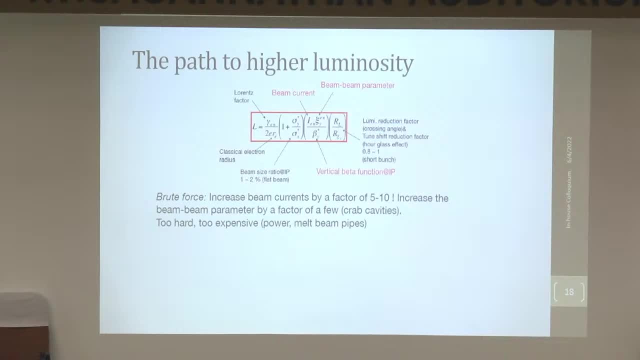 But we have lots of other things to do which are complementary, And I'll give an example with the very final thing that I show about that. So this expression here is how we define our luminosity. How we get to 50 times higher is to increase. 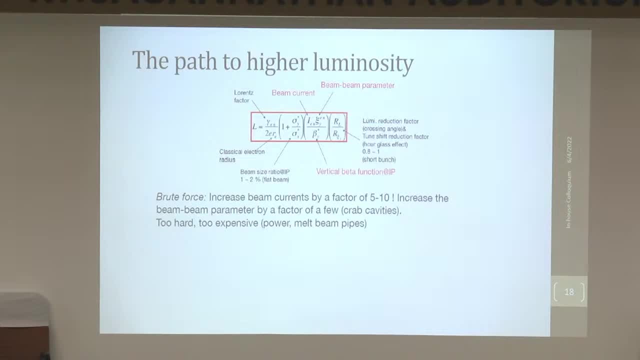 the luminosity of our accelerator. This is essentially a parameter of the machine that you multiply with the cross-section to give you the total number of events that you expect. And this luminosity relates to lots of quantities here which I won't try and explain in too much detail. 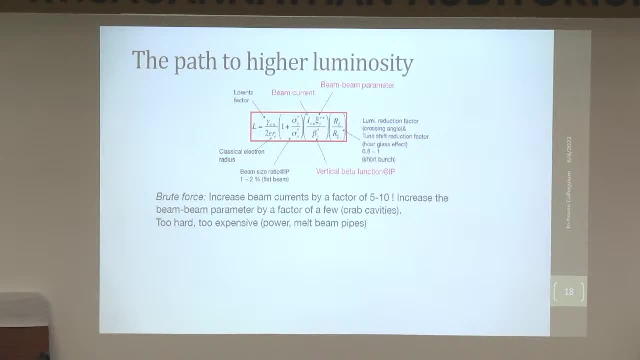 But I'll highlight a couple of these. One is kind of obvious: If your beams contain more current, you'll get more collisions, So you just try and increase the current here. This one is less obvious. It's called the vertical beta function. 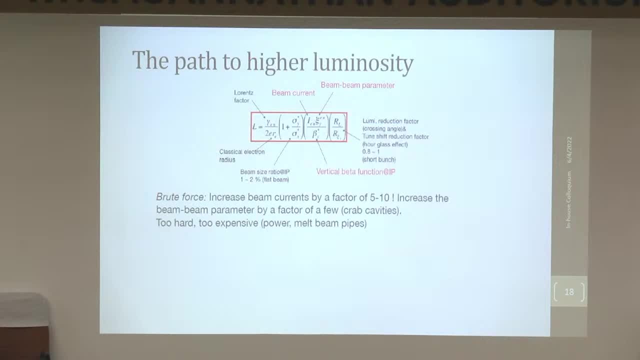 But essentially it's the vertical size of the beam. So if you can squeeze the size down of the beam and get more and more electrons and positrons in a small space with high current, you'll get more interactions. And how we try and tackle this is 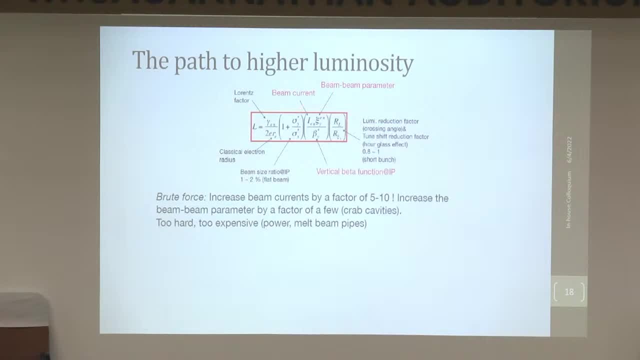 by reducing this beta function to boost the luminosity and increase the currents. But there's a real limit on how much you can increase the current because as an electron accelerates around, it's always radiating photons. This synchrotron radiation would actually 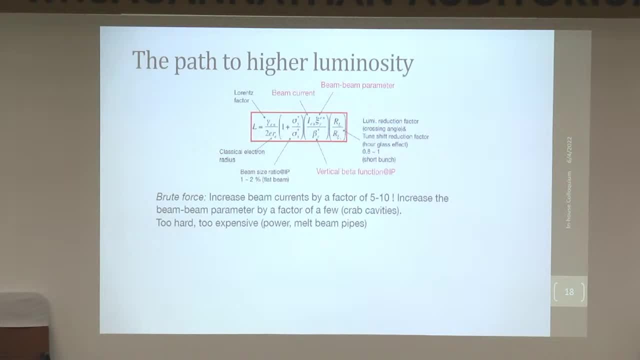 be so intense that it would melt the beam pipe. So we have to. if we were just going to say, OK, we're going to boost it by a factor of 10. So what's being done? I wouldn't say we. 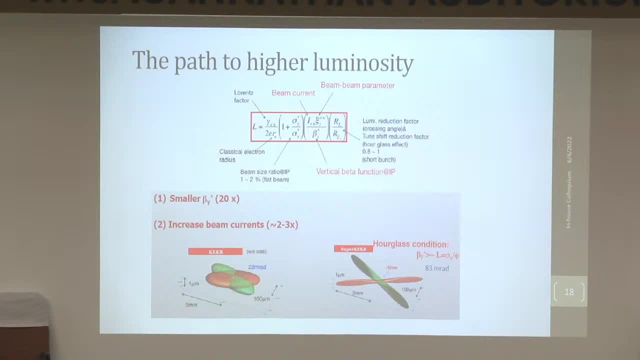 because it's very clever people from Italy and Japan who've done this- is to reduce this beta star function. So this cartoon down here is showing how a bunch of positrons and electrons interacted with one another in Keck B, which was Bell's experiment. 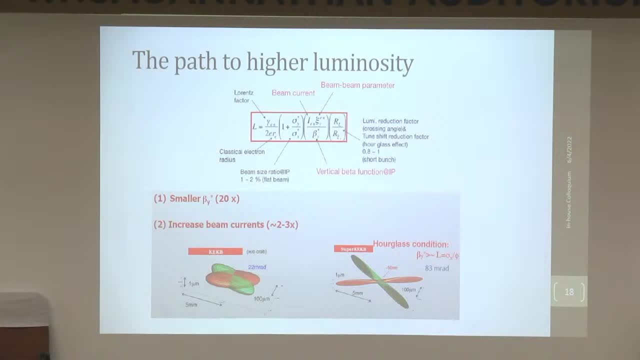 So that's what? two sort of ellipsoids that go through one another And you get your collisions formed here. But how we're doing this at super Keck B is we're reducing the size of this interaction region to a very small level, particularly. 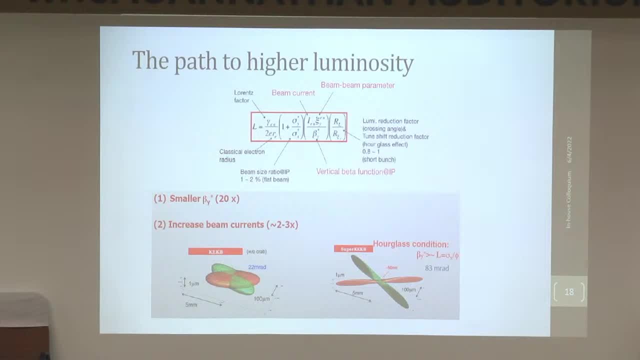 in the vertical direction. This is this beta star parameter, And we're going to increase this beta star parameter by a factor of 20 or so. And this is our big challenge is to make these bunches. And there's lots of fancy magnets. 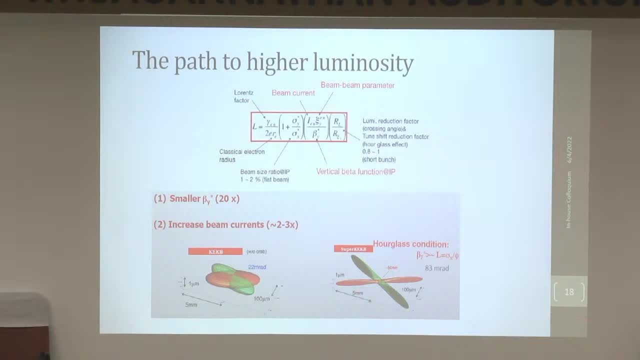 that go into making these sort of hourglass shapes of the bunches of particles so that they cross in this very, very small region here, And we've established this. I don't have the plots here, but we can measure the interaction regions much smaller now. 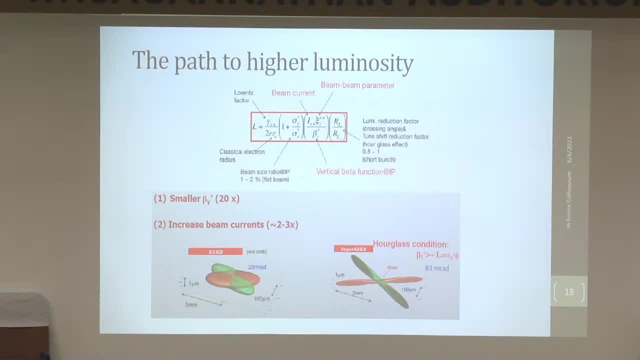 at super Keck B. Is it mutual or a small region? These collide straight, But there is a beam-beam interaction. This is this beam-beam parameter up here which I haven't talked about, Which you have to try and keep that as large as possible. Otherwise your luminosity degrades, And it's to do with something called the emittance, which is how well contained the beams are in their phase space, And so you want them as narrowly confined in phase space as possible. You want the smallest emittance. 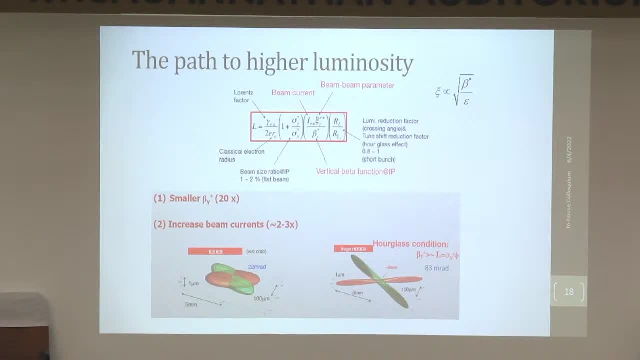 And that allows you then to do all of this without too much perturbation. But if you have too diffuse and too wide a range of different momenta in terms of the beams, you have lots of problems Because you're trying to contain particles with very different parameters in phase space. 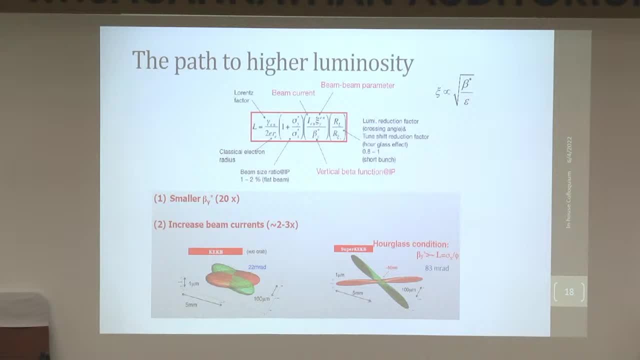 So you need to really reduce the phase space of the beams to be able to do this. Synchrotron radiation here is not a problem because this bit's in a straight line. It's only in the curves of the machine where we get lots of synchrotron radiation. 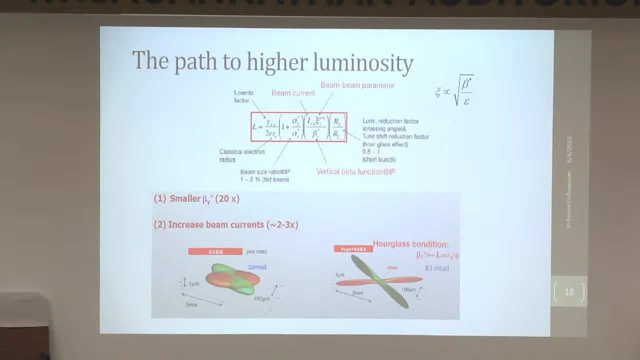 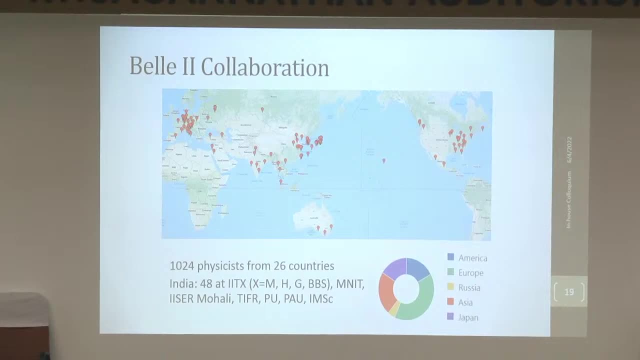 There's blow-up effects, There is interactions, but it's not synchrotron radiation. So that's a bit about the accelerator and how we get this huge luminosity. A bit about the experiment now, before I show the results At the end of the talk. 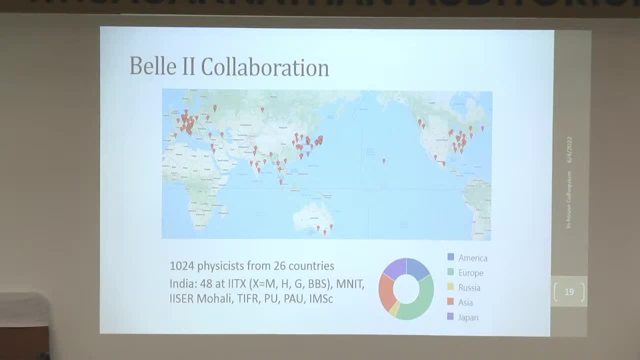 So it's a big collaboration. It's about a third of the size of the LHC experiments And it takes people from all over the world. There's around 50 of us from India working on this, Various universities and TIFR. 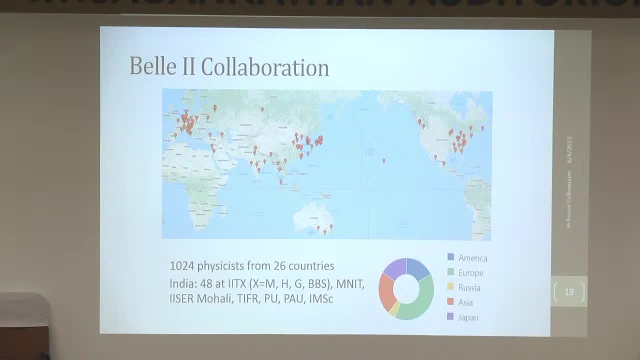 And it's split between Europe, America also There's also- this plot was made not in recent times, but Russia is singled out here. That's not on purpose now that we have to treat them so differently. This was done before for other reasons. 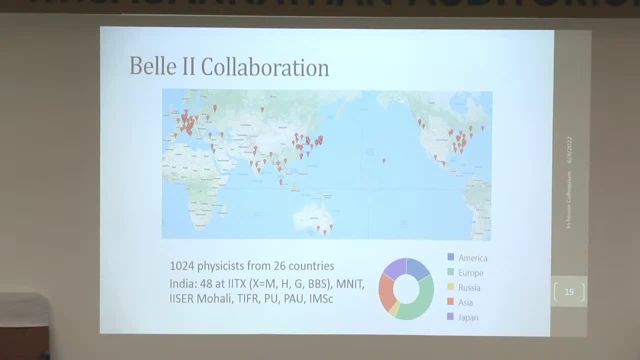 I don't want to go into the politics of this, but this is causing huge problems at the moment for us, But we currently are not submitting any papers, So it's like it is for everybody, But of course we feel for our Ukrainian group. that's here. 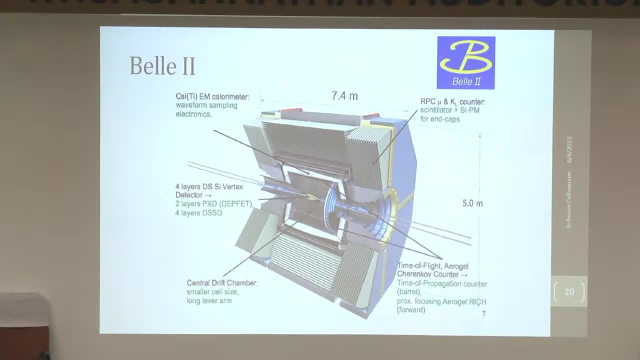 So the detector Is quite big, but not huge. It's five meters tall and about seven and a half meters long And has very similar structure to Bell and actually reuses the magnet, which is one of very expensive pieces: 1.2 Tesla solenoid which causes curvature of the charge track. 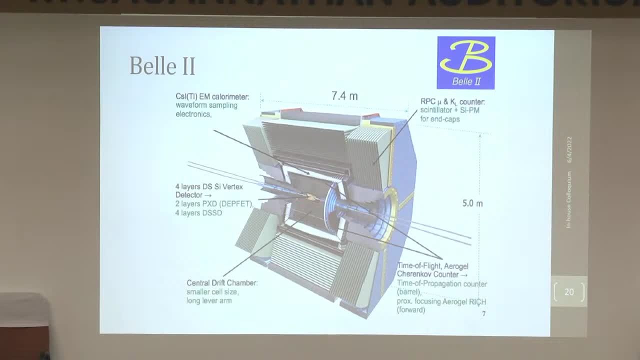 so we can measure the momentum. But we have an entirely new silicon vertex detector in here which has larger acceptance and much better precision. We have new particle identification- This time of flight- and aerogel counters. here We have the same calorimeter, which is a very precise crystal. 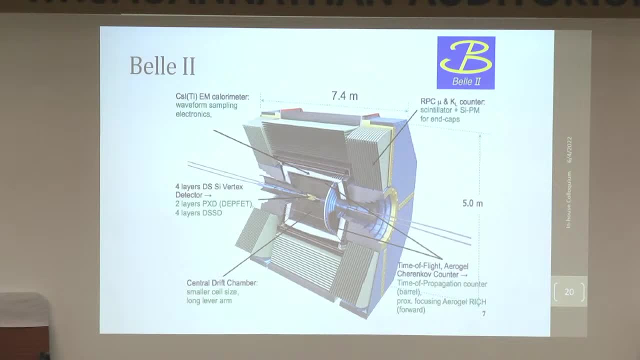 calorimeter, so all the energy of the photons absorbed And you get a good measurement of the photon energy and hence pi zeros. And because of the rearrangement of the detectors and particularly the magnets that have come in to do this squeezing of the beam, we've 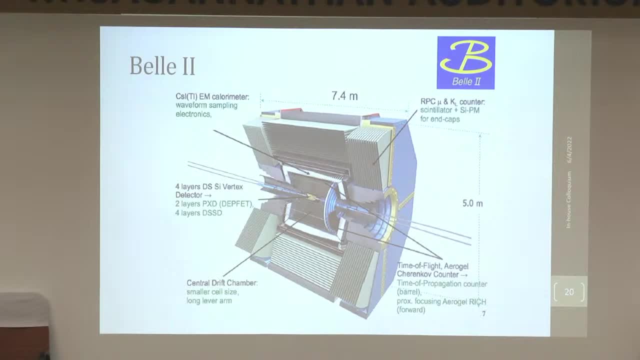 had to make a new drift chamber, which is just a wire chamber, But it's got smaller cell size to better protect against Against backgrounds that come off these beams. So I just want to highlight one part of this, which is the silicon vertex detector. 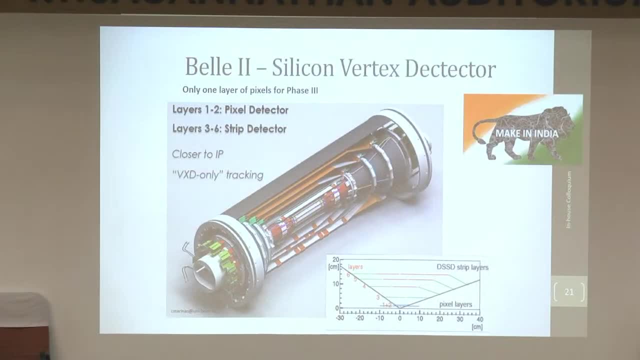 This was not entirely made in India, but partially made in India. One of these layers of the silicon vertex detector which is designed to make those precise measurements of the decay position of the bees and allow these time dependent measurements, as well as do tracking of low momentum particles. 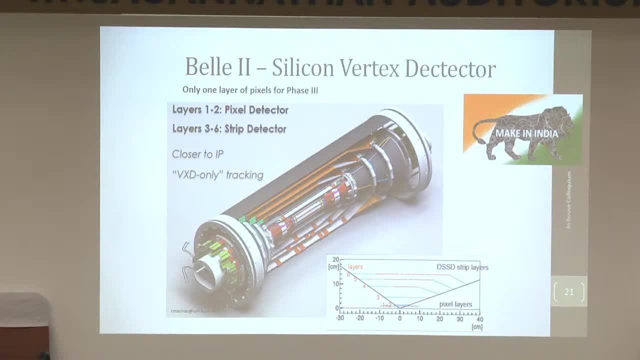 There are layers of pixels in here, but then there are layers of strip silicon: 1.2 Tesla solenoid which causes curvature of the particles, 2.3 silicon detectors. And this layer four was entirely built by a group of Indian institutions led 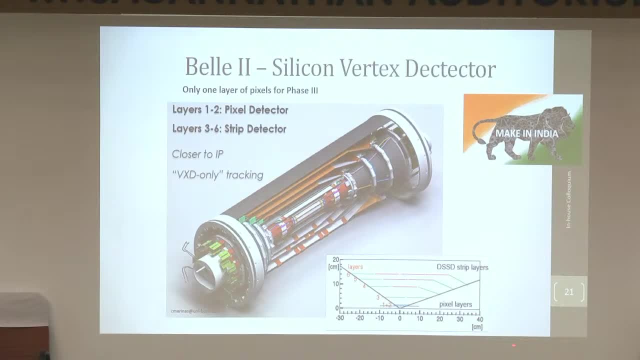 by Tata Institute, which one of my earlier PhD students, Resmi, contributed to the construction and commissioning of this detector, And we're now involved with the operations of this, which I'll tell you about- operations, I think- in the next slide. 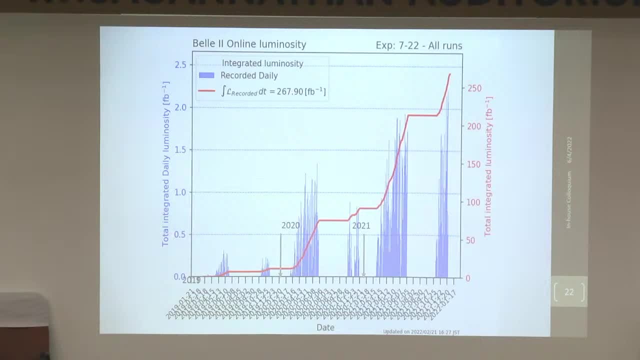 Yeah, So this is luminosity, the thing we really care about and how we've integrated it since we started in 2019.. So, don't ignore this, I've put the years here, So this is 2020 and 2021. 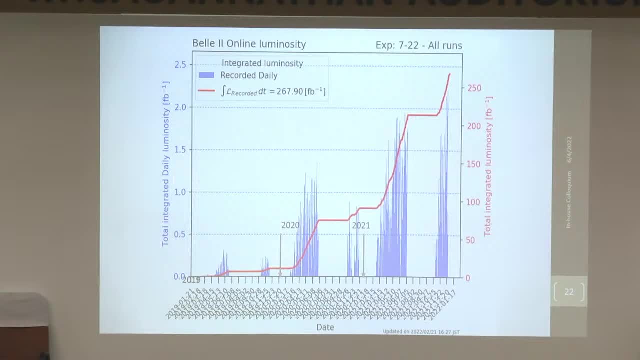 So, as with all new machines, you have a slow start. You're trying to get as much luminosity in a short period of time And we've slowly been increasing And you see we're accumulating data at faster and faster rates. The gaps are due to the fact we can only 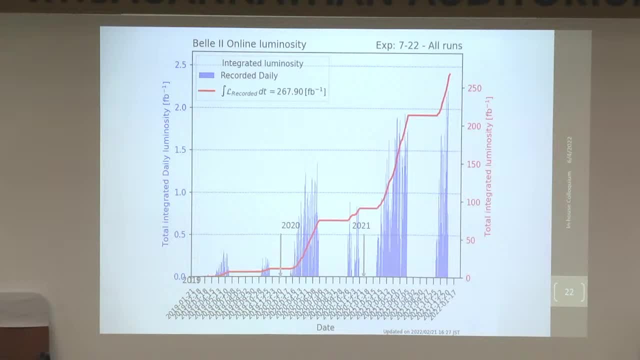 run for six months of the year To accelerate particles. it's expensive in terms of wall power of electricity. Every time these electrons and positrons go around they lose energy. You have to accelerate them with an RF system again, So in the summer, when they're using the most electricity. 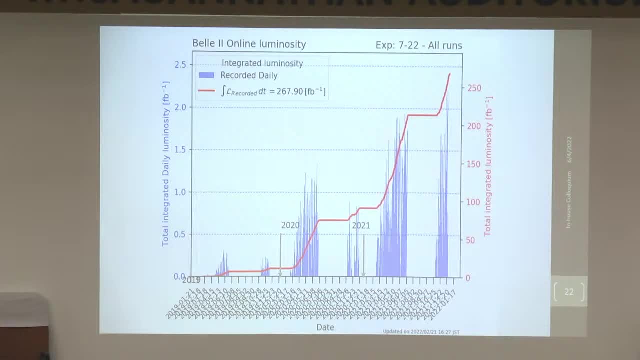 in Japan for air conditioning, we don't run. We now have problems that we have to truncate our run because of energy, But that's another story. So far we've accumulated around 250 inverse femtobonds, which is a third of the Bell data set. 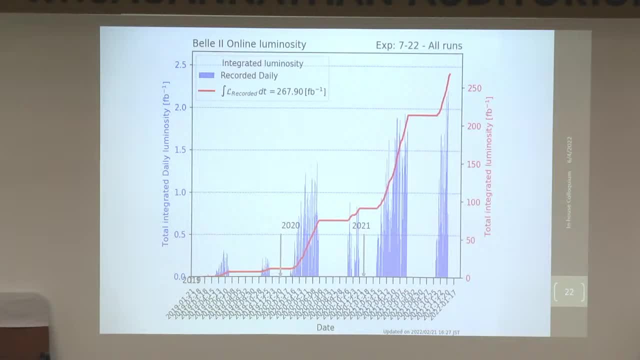 And we hope to get towards over half of it before we stop in the summer Note. we were taking data throughout the pandemic, So we were running this detector in Japan And all the sub detectors around it. the accelerator was running and we were running the detectors. 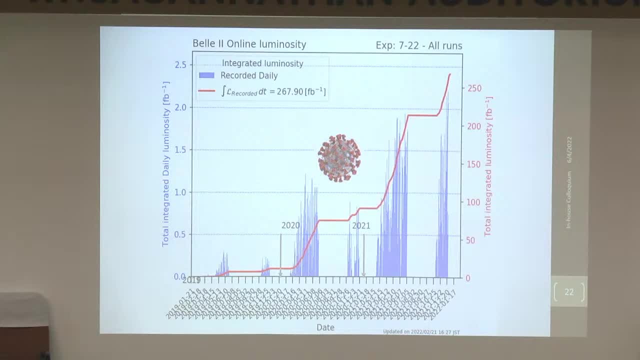 So for this vertex detector. for example, I was sat at my dining table in Chennai but had the ability to operate the silicon vertex detector. I could ramp up the voltage, ramp it down, put it in or out of data taking. So we devised systems to allow us to keep on running. 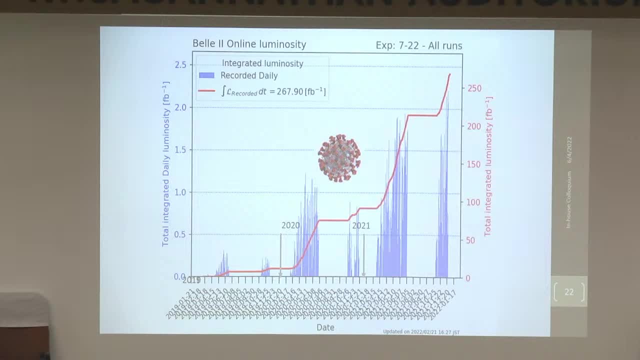 Of course we're not going to run it. We're going to run it. We were heavily reliant on our Japanese colleagues, who worked in difficult conditions, to keep this going, But it still worked And we're going some way forward with our data taking. 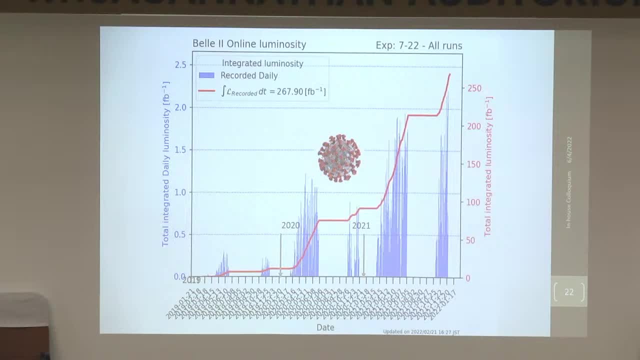 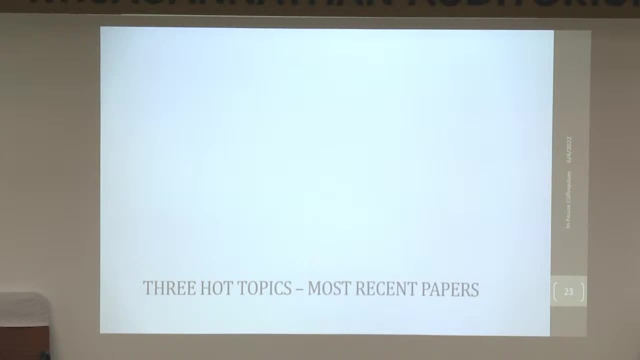 But we're still a long way away from that 50 inverse atobonds we want to ultimately collect. So in the last 10 minutes I'm just going to talk about three recent results, actually our three most recent papers from Bell 2, to show that we're 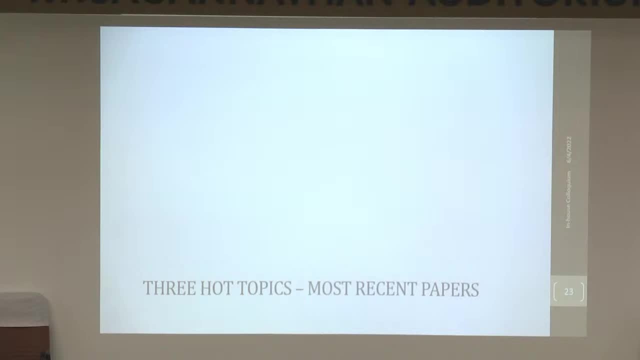 now producing physics papers, And they have quite a lot of, particularly the last one. So first, one of these just showcases our silicon vertex detector. We've measured the lifetime for demisons more precisely than anyone else has done this before. So these lifetime measurements, test models of QCD. 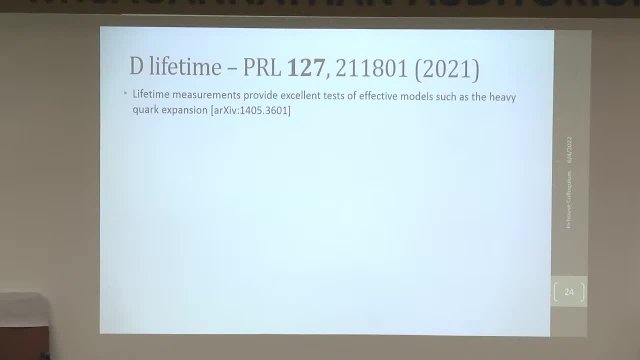 essentially of how these demisons should decay when you integrate over all their possible final states, And the most precise measurement was actually done 20 years ago by an experiment in Fermilab called FOCUS, And it's been used as a reference for all other lifetime measurements. 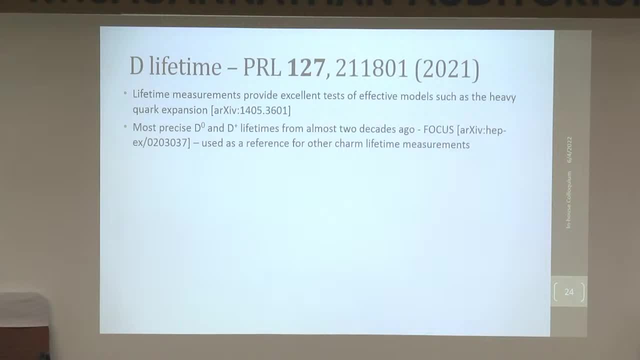 So there was a desire to improve this, or at least double check that that measurement was correct. So, as I mentioned before, we don't just make Bs, We make charm quarks as well. So E plus, E minus goes to CC bar. 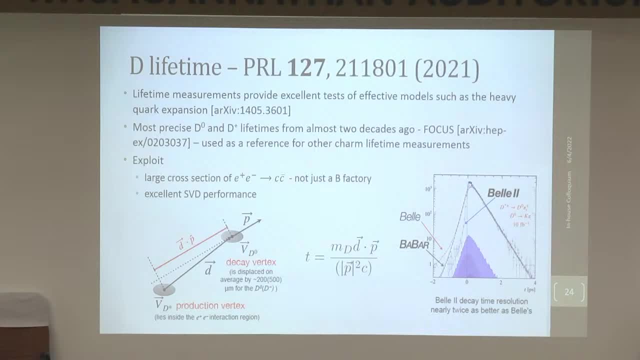 And they tend to produce what's called a D star meson which decays to a neutral D and a slow P OK. So you can make a vertex where the D is produced and where the D star is produced at the interaction point. 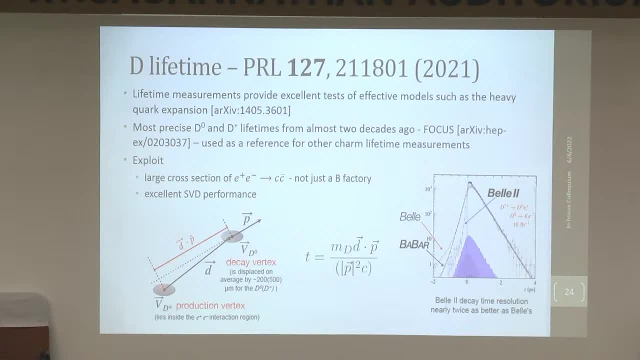 And then the D flies some distance and then decays. So you can measure both of these things And then, just using a bit of geometry about the position of the decay and the momentum of the decay, you can relate this back to the time it took to travel. 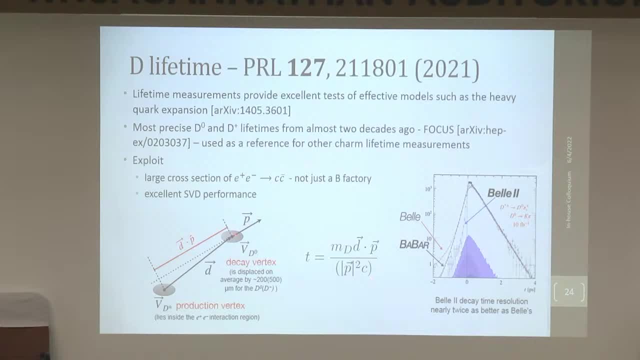 if you know its momentum. So we go on to measure the decay products and measure its momentum. So this relates you back to the time And of course this is a boosted time. So that's why the momentum's in here And what this plot here shows you. 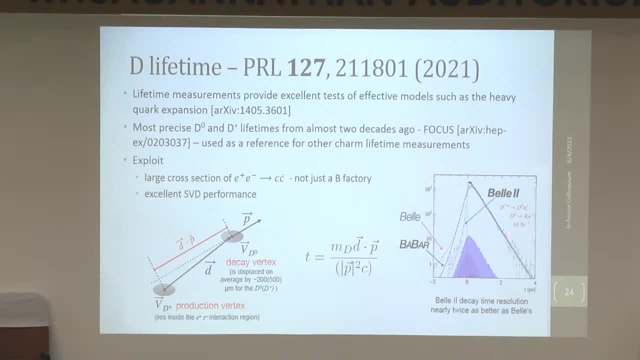 is the distribution of the time of these decays. So the left side, these negative times are things to do with the resolution of the detector And the stuff on the right-hand side which is going out to larger values are real decays that happened away from the interaction. 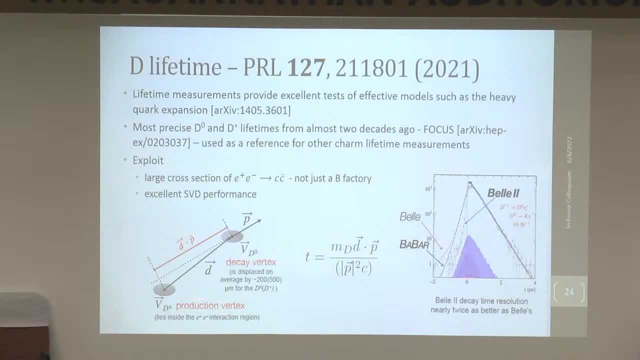 point here And then, fitting this very carefully, taking into account the background, you can make a precise estimate of the lifetime. So these are measurements of the lifetime. It sounds very short. It's about around 1 picosecond femtosecond. 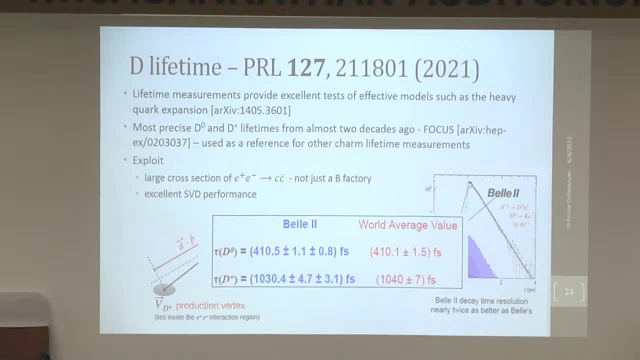 But we're measuring this to the order of 1 femtosecond for the D0. And the D plus, due to higher backgrounds, is measured somewhat less precisely. So this shows how the vertex detector is working. This would not have been possible with Bell. 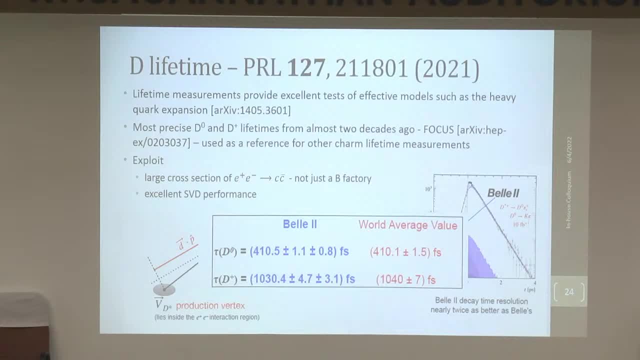 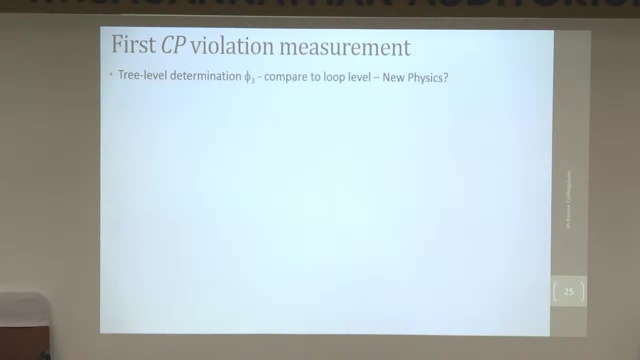 And that's why it wasn't done until we had Bell 2.. We need very little data to do this, because there are so many charm quarks produced. So now I want to talk about a CP. Yeah, just more precise, There's no problem. 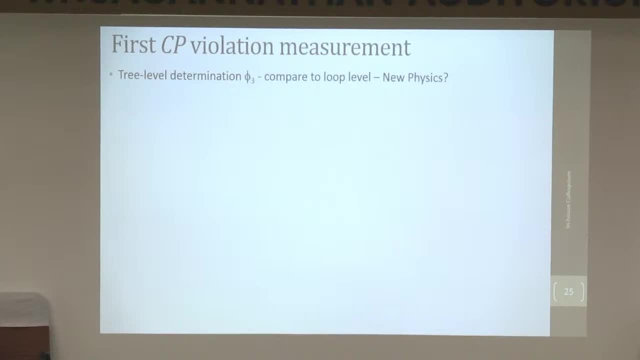 Yeah, going back to my unitarity triangles, one of the key components of making a more precise between the one affected by loops and the one affected by that it's unaffected is pure standard model. We think the tree one and no loops is to measure this angle. phi three: 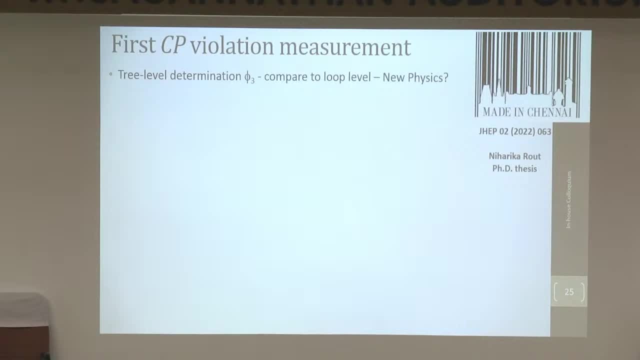 And here in Chennai, Niharika, who, for example, is also a rectangular model- Yeah Yeah, whose Fiverr was on Monday- has made this measurement, which is the first measurement of CP-violating parameter at Bell 2. 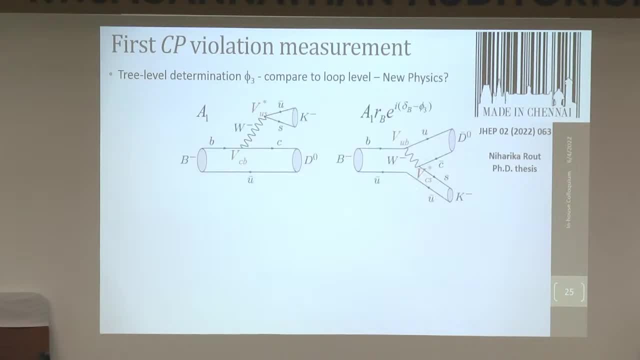 and is of this Phi 3 parameter which was published in J-HEP earlier this year. So what we're doing here is measuring this Phi 3 angle, or gamma, which relies upon the interference between two different decays of a B to a D0 and a K-on and a D0-bar to a K-on. 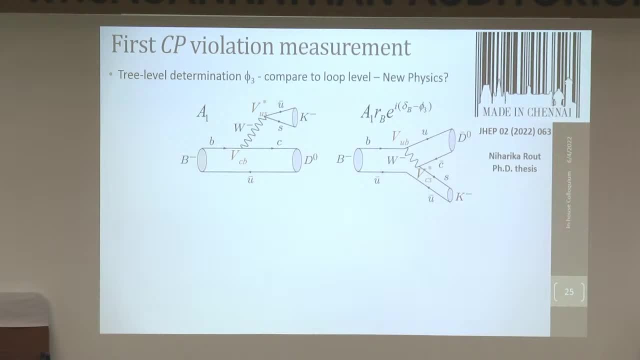 which have these quark constants given here. And this one depends on this VUB matrix element because you've got the B quark transitioning to an up quark. So you pick up this standard model of CP-violating phase Phi 3.. 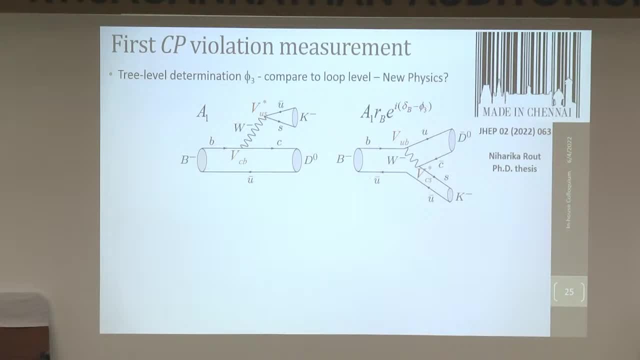 Now this delta B and this RB are QCD parameters, which are a nuisance to us, but we can actually measure them as well in the data, So we extract those as well, so we don't have to worry about any predictions. So this is very theoretically clean. 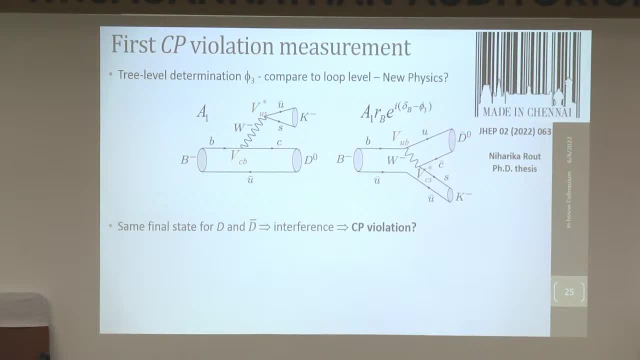 So as long as your D0 and your D0-bar decay to the same final state, all of this will interfere and you can get access to this Phi 3 parameter. So there's a very interesting technique that was proposed a long time ago. 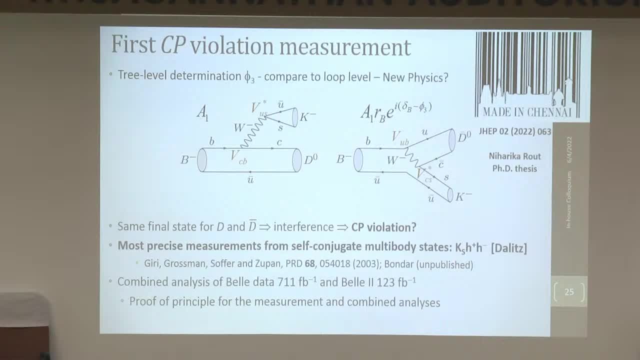 and then finally been implemented both by Bell, Bell 2, and LHCb, where we can measure this using a final state of the D0 going to a K-short, normally a Pi-plus and a Pi-minus, but we also use K-plus and K-minus. 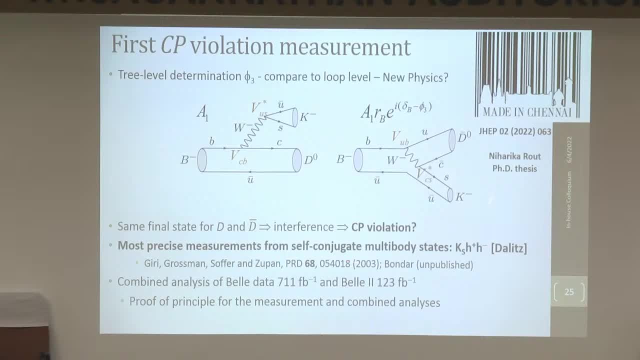 And it's a Dalitz plot, and I'll show that in a moment. And what's particularly novel about Niharika's analysis is we've actually merged the Bell data and the Bell 2 data, because we're not going to have much more than Bell for a while. 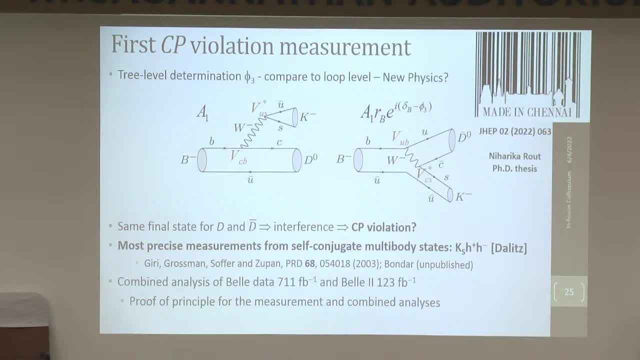 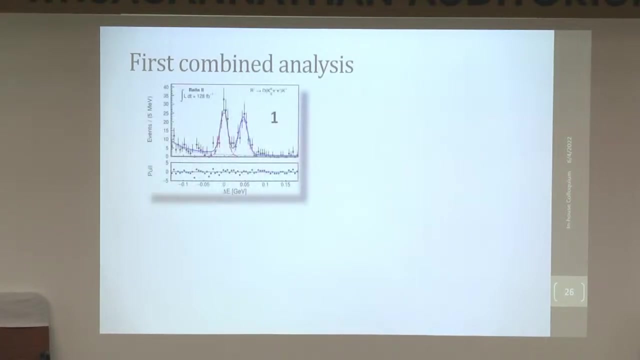 but we can at least reduce our uncertainties by 40% or so by combining two data sets and using improved analysis techniques. And there'll be many more of these in the next couple of years. So, just to guide you through this, this is what we look for. first is our signal. 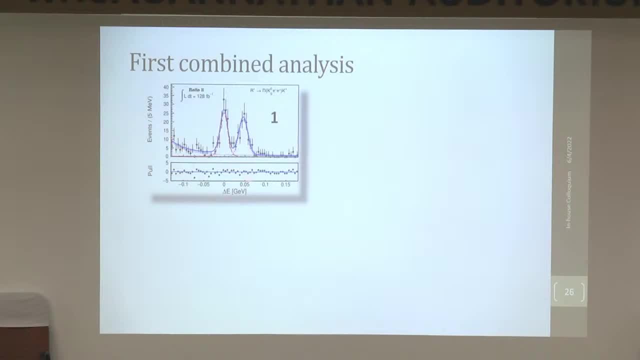 which is here in red against the background, And this is using a kinematic variable that relies upon the fixed knowledge of the beams beforehand and the energy of the beam meson when it's being reconstructed. It's called the difference between these two. 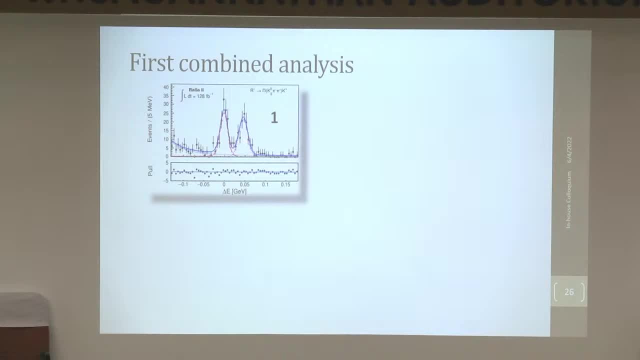 and it should be zero for a signal. This peak here is a decay of B to D Pi and is offset kinematically due to the mass difference between the pion and the kaon. so we can separate these kinematically. But this is a superb control sample. 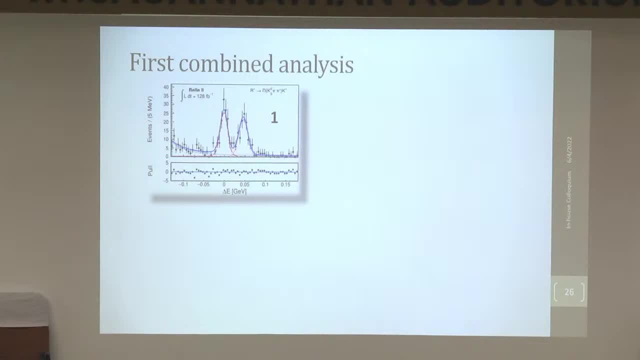 because it doesn't exhibit CP violations. so we can use that to calibrate everything. Then this is our Dalitz plot, which is the invariant mass of the k-short with one pion on one axis, so the pi-minus up here and the k-short with a pi-plus down here. 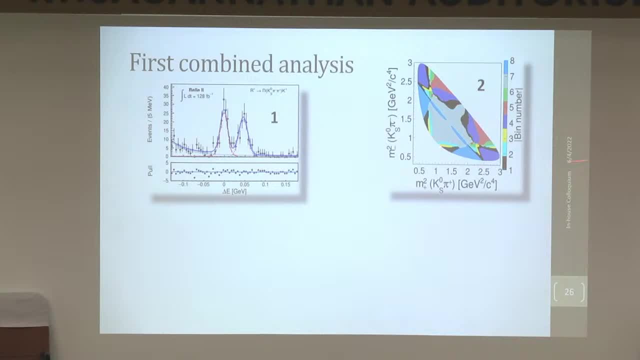 So this is a symmetric Dalitz plot and we bin our data in this Dalitz plot. Why we choose these bins is because they have certain values of those strong phase parameters which can help us get different amounts of CP violation in the different bins. 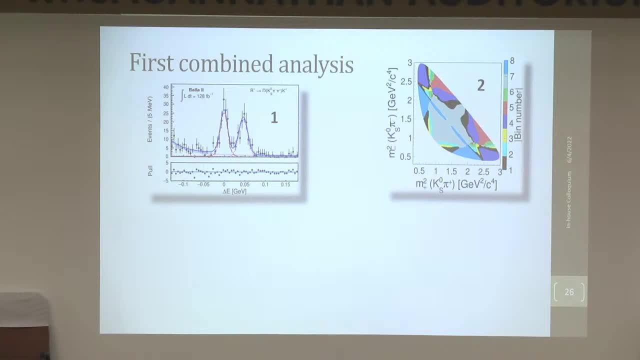 and we can therefore extract both phi-3 and these hadronic parameters, rb and delta b, in one measurement. So this is the asymmetry, the CP asymmetry between the b-plus and the b-minus, decaying and you see it wiggles around this line of zero here. 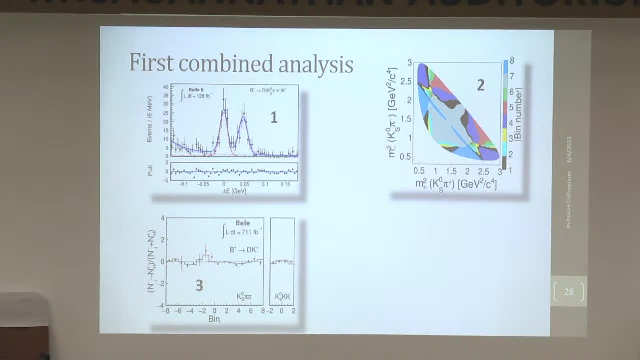 and if there was no CP violation it should all agree with this line. So it's not too impressive in this plot, I agree. but once you do the statistical analysis and you measure the value of phi-3, you get something that's significantly away from zero. 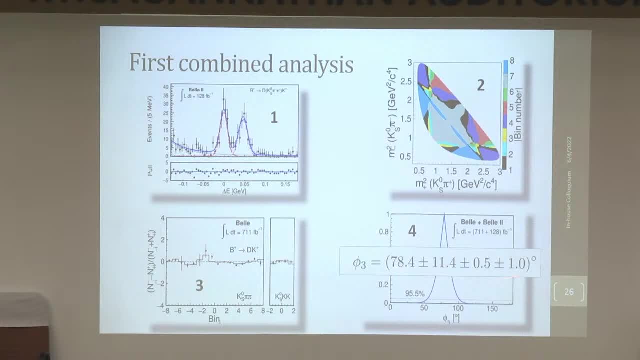 and we measure phi-3.. We measure phi-3 to be around nearly 80 degrees, with an uncertainty of around 11 degrees, which is much more precise than we managed with the earlier data and because of largely the techniques that we've introduced. 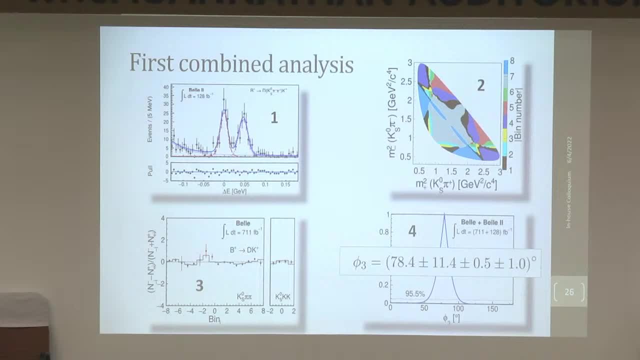 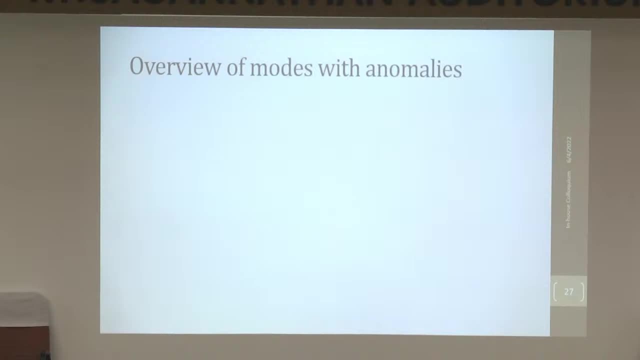 we've reanalyzed the Bell data and improved the measurement by- statistically it's about a factor of two- by just adding this little bit of data and improved techniques. So in my last five minutes I will move to the hot topic in flavor: physics. 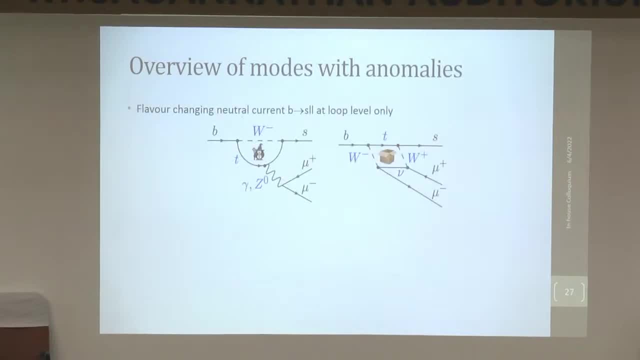 maybe some would say in particle physics, and this is what's so-called B anomalies. These are flavor-changing neutral currents where you have a B quark turning to a strange quark. So these are both quarks with minus a third charge. so that's why it's called a neutral current. 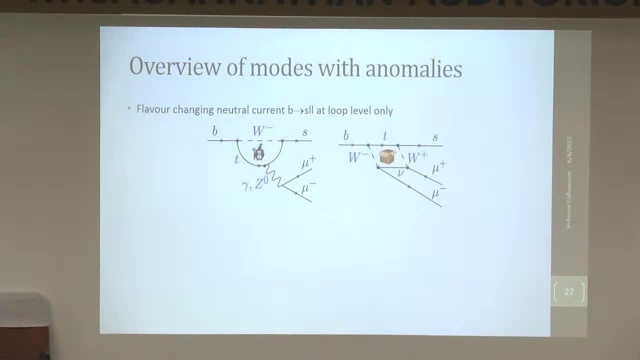 and then it has two leptons in the final state. So I have Feynman diagrams that can do this. One is called a penguin diagram, where you have a W and most often a top in the standard model, and similarly you can have a box diagram. 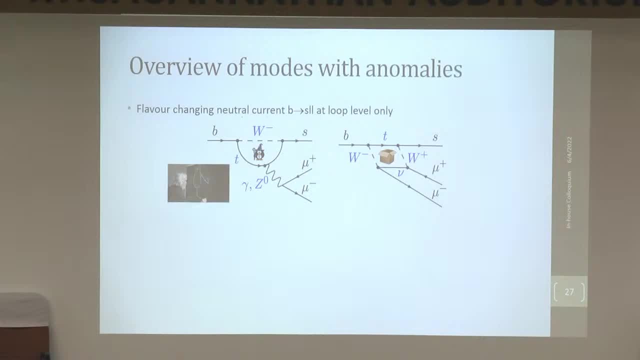 where you have a top and a neutrino. Now, why this is a penguin diagram is an interesting story. So John Ellis, who visited us pre-pandemic so a long time ago, he came up with the idea of a penguin diagram. 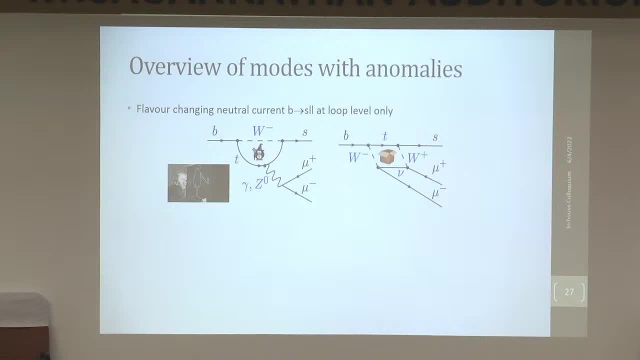 to basically win a bet. He'd lost a darts match, so he had to get the word penguin in his next paper and he reckoned that this looks like a penguin. You can read more about this and you realize why he might have imagined. 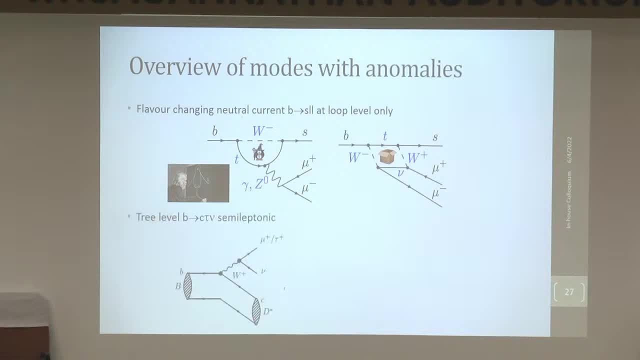 it looked like a penguin. So this is one class of anomalies. These things are not agreeing with what we expect in the standard model. and then there's another type as well, where we have a B to C transition, which is the most favored. 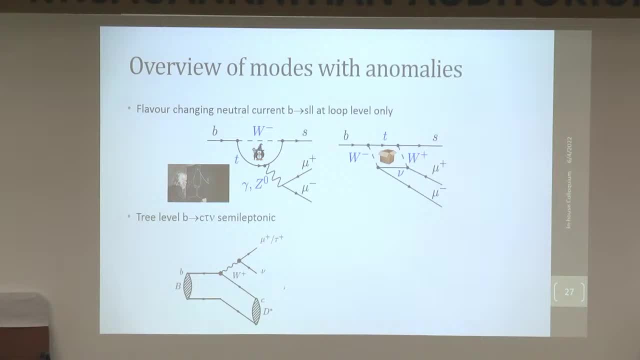 and then the W produces a tau lepton and a neutrino and this can be compared to the muon. You can make a ratio and this ratio is not agreeing with what we expect. So these two types of anomalies, this B to SLL. 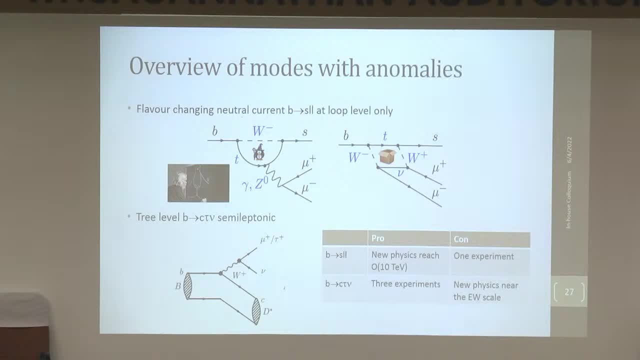 because it's purely loops, has huge reach in terms of higher mass scales, much beyond what we can look for directly at the LHC. Unfortunately, only LHCb has seen this so far, so we always like to see confirmation between two different experiments. 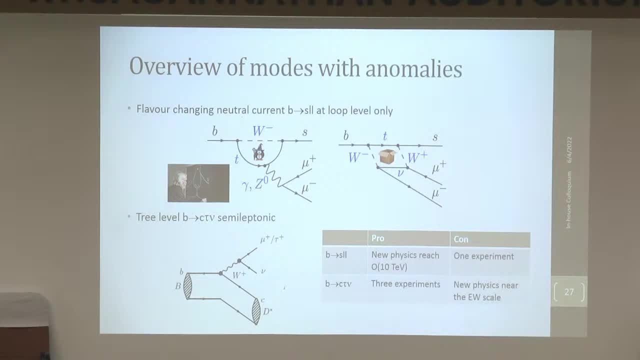 Whereas this B to C tau nu anomaly has been seen by Bell Babar and LHCb, and this is much easier at Bell 2 because of this neutrino. so we are the experiment that's supposed to finally see whether this is true or not. 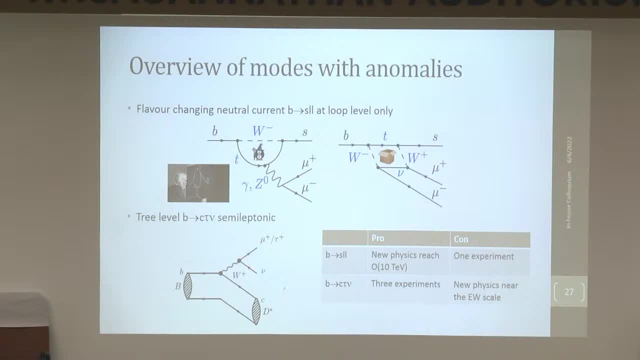 Now the interesting thing potentially about this anomaly is the new physics must be much lighter. It has to be much lighter. It has to be at the electroweak scale which is around the mass of the W, which is 100 GeV or so. 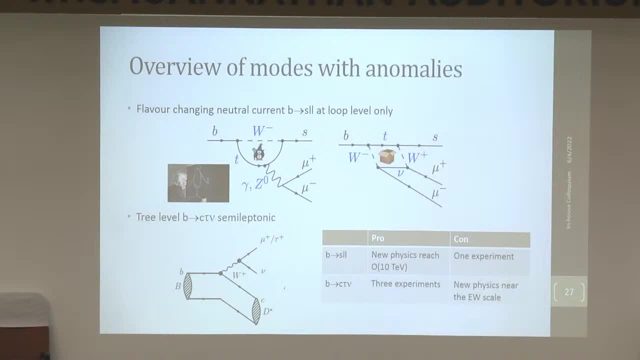 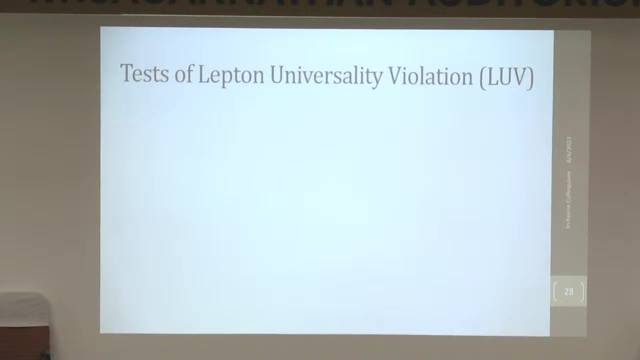 So it's much lighter new physics and that's hard to explain given all those limits that have been set at the energy frontier. So this is more problematic theoretically to describe Here. there are many, many possible new physics explanations. The rates don't agree with the prediction. 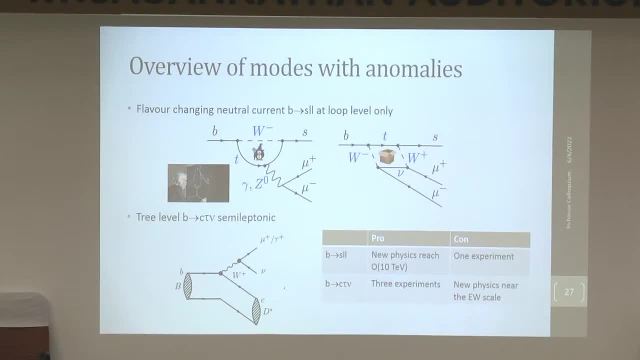 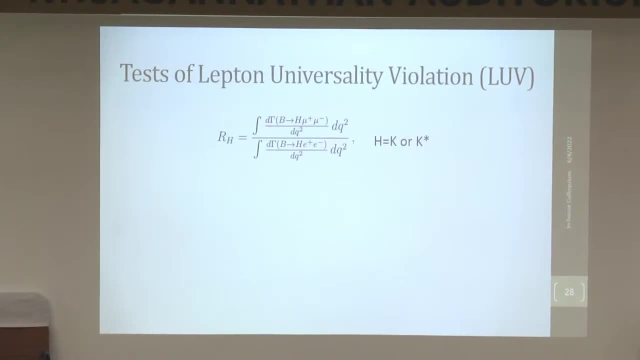 It's just a ratio. I'll talk about this one. I don't have time. I don't have time to talk about this. I'll have it in the backup. So what we measure is: you measure the rate of the decay where H here is a k-on or a k-star. 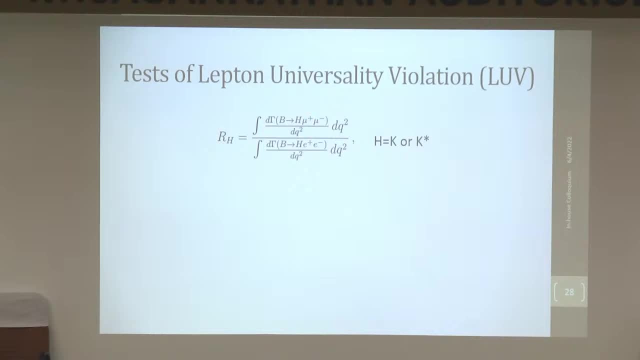 for this B to k-mu-mu over B to k-e-e, And in the standard model we expect the rates of these two to be almost exactly the same, because there's something called electron universality, where the electron and the muon couple with the same strength. 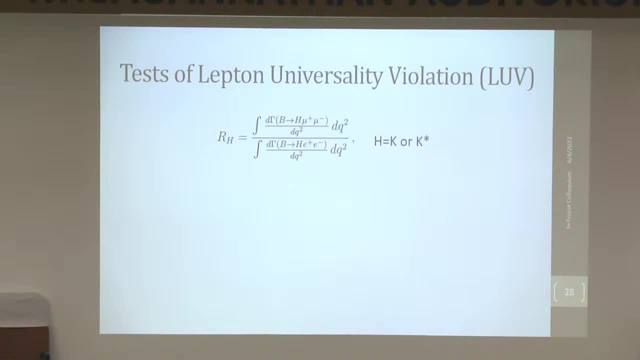 to the W, the z and the photon. So this can be really well predicted and all the theory uncertainties- or most of the theory uncertainties- drop out in this, because all the things to do with form factors are the same, because that's on the quark side. 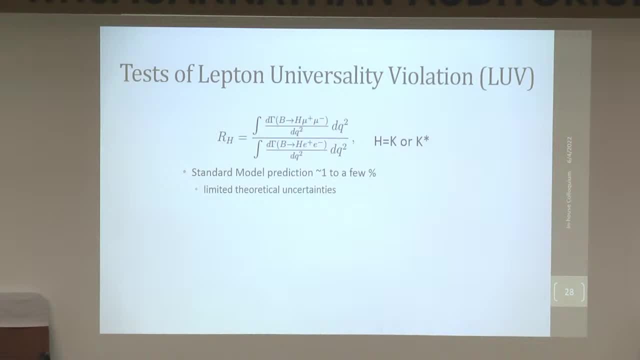 and the new physics is on the lepton side. So this is predicted to a few percent. So this is a really good observable to try and challenge with a precision measurement. So LHCb have done this and this is their control channel where they have a Jsci which decays to two leptons. 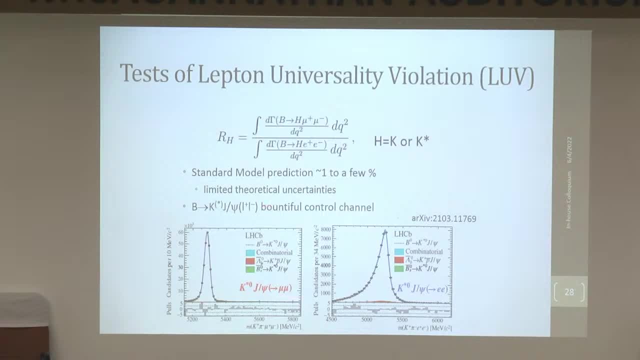 It has charm quarks in it, so it's produced a lot from Bs And you see here their B-mass peaks. You also see, this is not a Monte Carlo simulation. They have barely any background beneath this. But you do notice that their electron resolution is very broad. 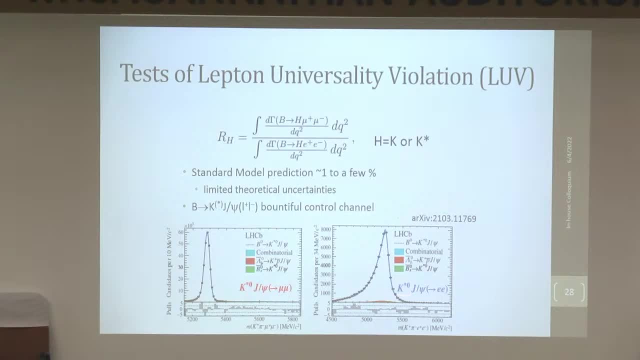 and this is a cause of concern- that there might be some problem here, and that's due to the fact the electrons, as they pass through the material of the detector, are likely to radiate photons and you don't reconstruct all of those photons. 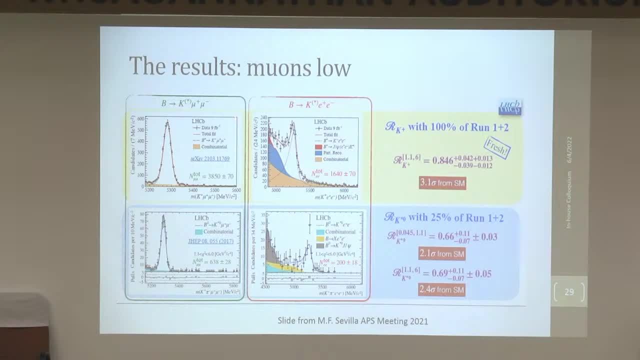 so-called breakouts. They're M-strong photons. When they do this on this mode away from the Jsci, they see the muons very clearly. They also can see a nice electron peak as well, and they take the ratio between these two. 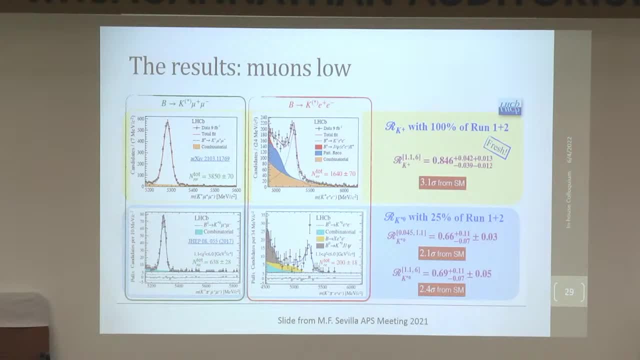 and they do not get one. They get around three standard deviations below for the kaon, and then there are two different measurements where they're getting around two standard deviations below. So that in itself is not very interesting. Three is very interesting in one measurement. 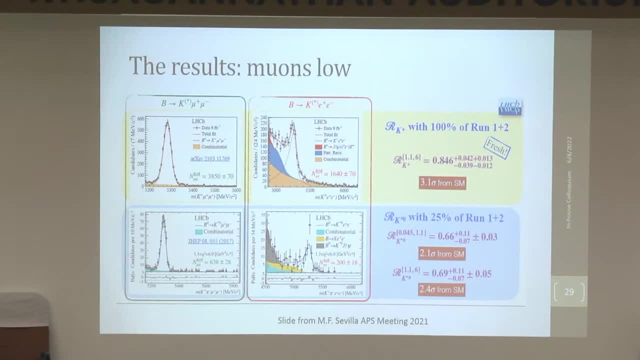 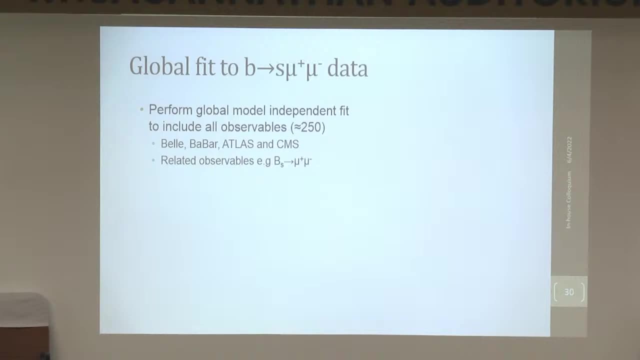 So these are the LHCb results. They're not very interesting in one measurement- They're not Bell 2, so I'll move quickly over these and just describe what people think might be going on, So you can actually make many, many more measurements. 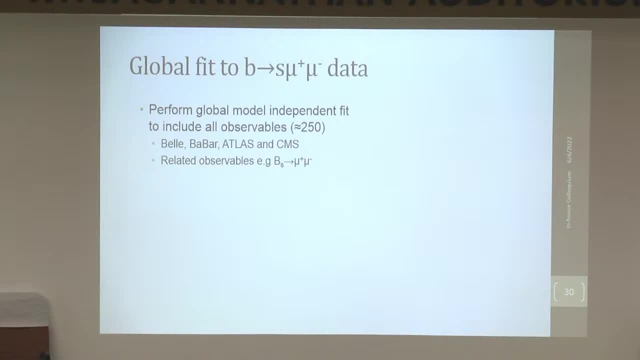 particularly for the K-star case. You have lots of angular observables that you can measure and in fact all these experiments, LHCb including these, have measured about 250 different observables that are sensitive to this BSLL process, and there are other variables. 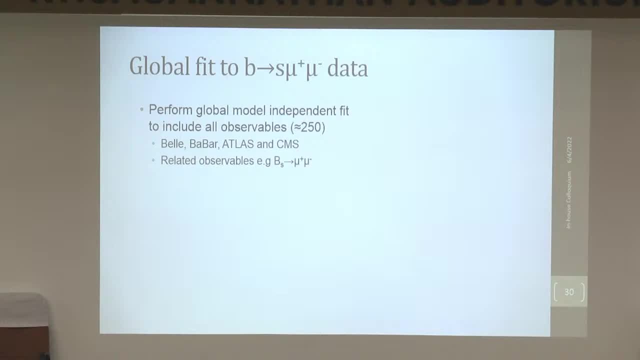 related to very rare decays of Bs, to the analog of that K-long that I started with in a B meson going to two muons, which is also related, And what you can do is you use expansion where you have something called Wilson coefficients. 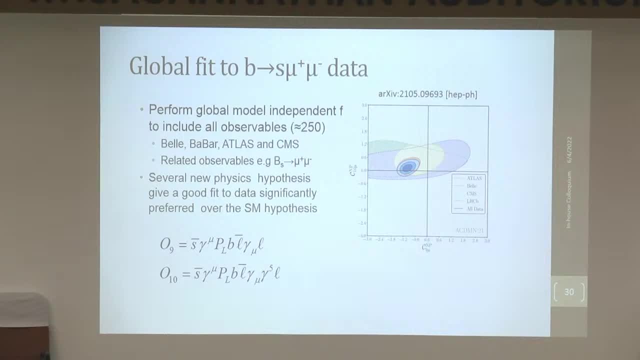 where you integrate out those heavy mass scales and you just have point interactions, like old-school Fermi theory in nuclear physics, if you're familiar with that, where you integrate out the W and you can see how much new physics is required in these observables with these four Fermion operators here. 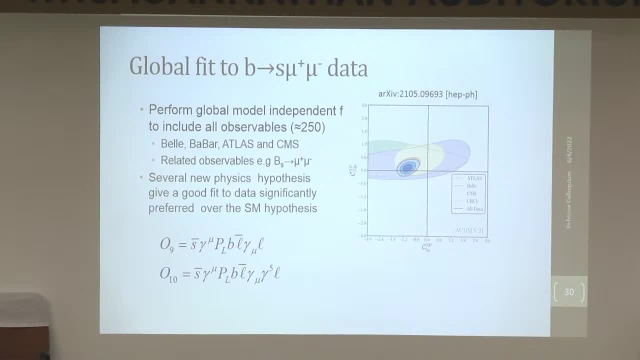 So this is the S quark, the B quark and the two leptons, and this is a different one with a different chiral structure. And what you see this is the best fit is, if there was no new physics, it would be here. 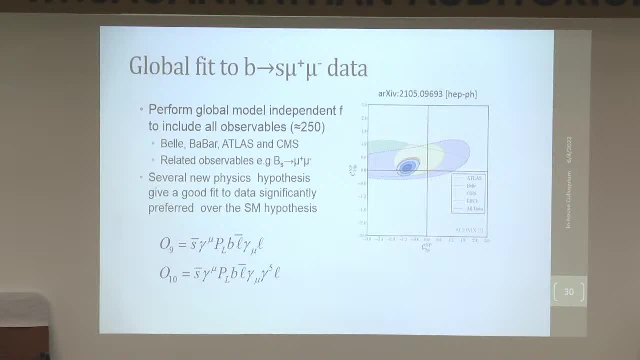 but it's some way away And these fits will show you. depending on the assumptions that you make, you can get anywhere between six and seven standard deviations from these anomalies. So this is all very exciting, but it's not one single measurement. 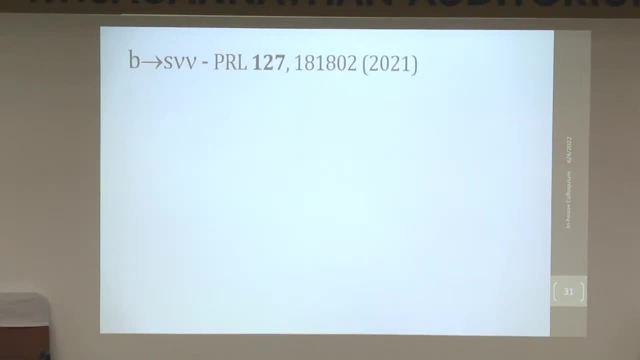 and the whole picture is not entirely clear yet. So what Bell 2 has managed to do is to measure a complementary process, which is the B going to the S, but not to charge leptons but to neutral leptons, And this was published last year. 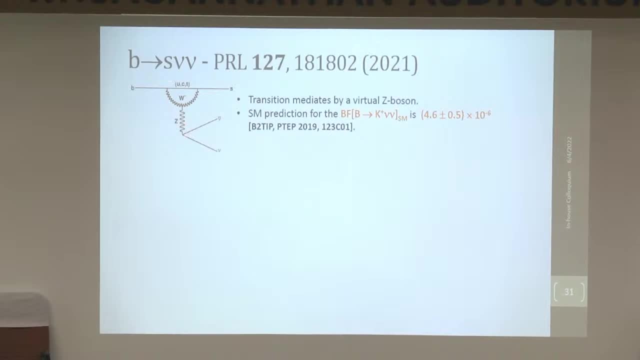 So this has one of these diagrams contributing, this so-called penguin diagram, because we just need the Z here, We can't have the box diagram. So this, essentially, if there's new physics contributing, it would contribute in some different way in this measurement. 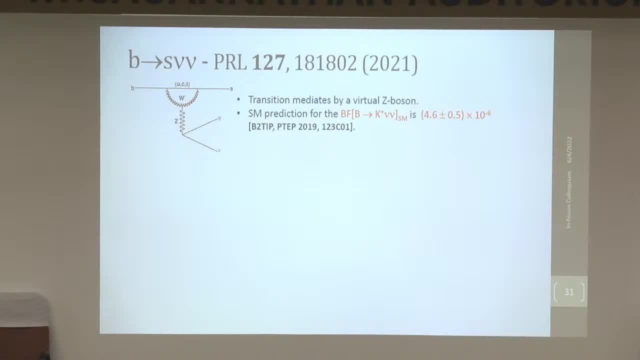 So there's a reasonably precise- 10% or so- standard model prediction for this which we can compare to, And we developed a technique which uses machine learning to basically differentiate between our different types of events. So if you have BB bar events, all the decay products come out. 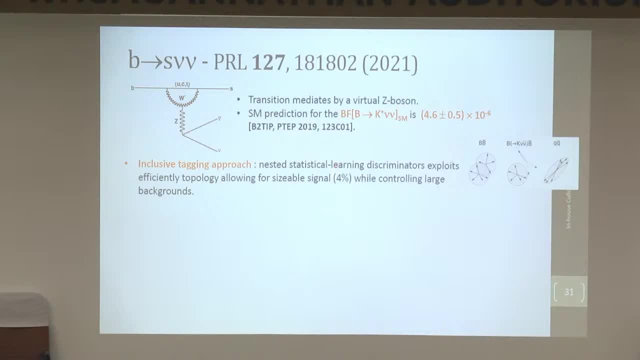 relatively isotropically over the 4 pi solid angle QQ bar events. they're collimated with one another because they go out back to back to one another. But in these events where you have two neutrinos you have some weird intermediate topology. 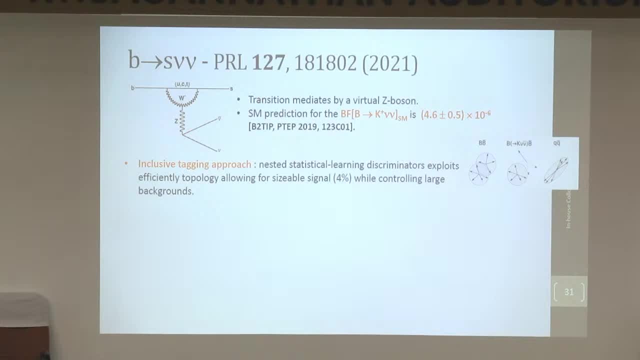 which is distinct from these two. So we trained on simulated samples which are calibrated on data, which were then calibrated with data samples. So it's a data-driven approach And we could distinguish this final state And, unfortunately, the variable that comes out. 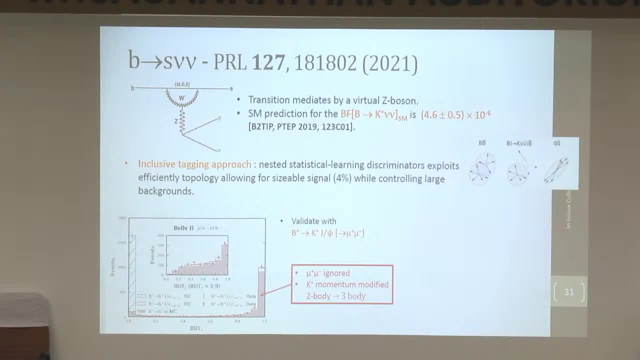 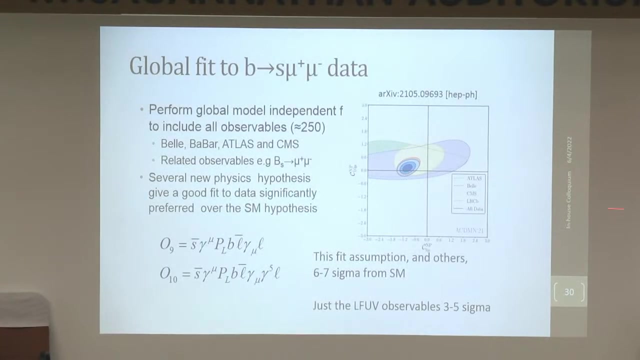 is one of these multivariate discriminators. It's a boosted decision, It's a boosted decision tree, But the signal would peak up here and backgrounds would peak down here. So this has been carefully validated. Okay, What you trust, right? 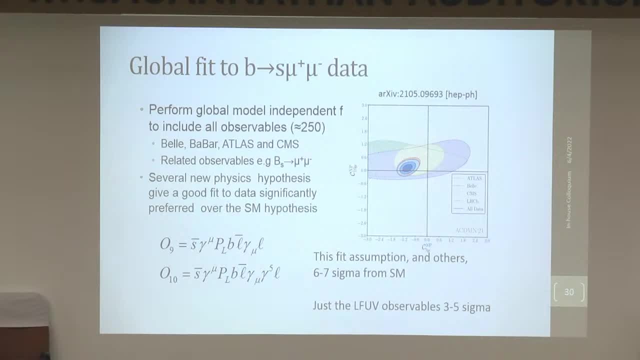 We, we, these other, these other experiments don't have the precision, But there are some interesting variables that are measured by Bell, that are not measured by LHCb. This pink circle in behind that's LHCb. The whole thing is driven by one experiment. 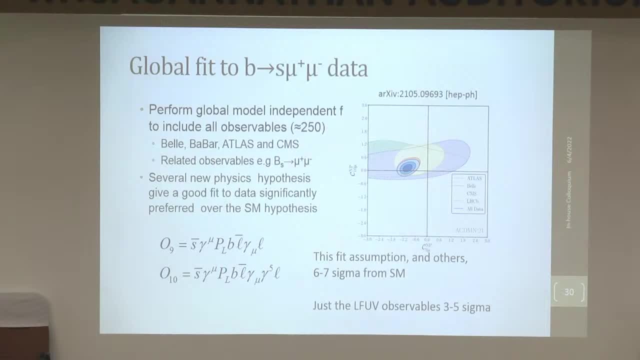 Okay. So your question of trust is whether other experiments will see the same effect. Yeah Yeah, The process of prediction, the standard. this is saying if, if standard model is there, these Wilson coefficients, they're relatively straightforward to calculate. 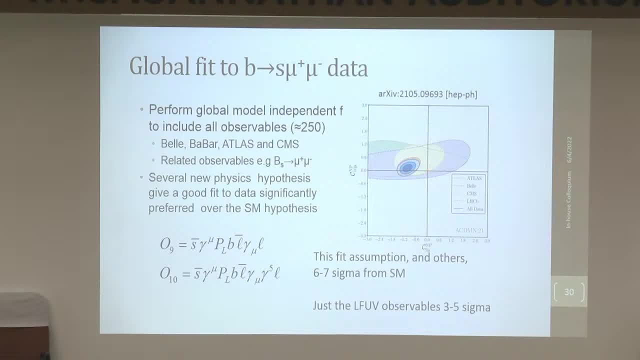 They would predict that there could be no this. so this is a Wilson, the Wilson coefficient. you measure less. the prediction And whatever's away from zero is not coming from anything we know about in the standard model. I can't tell you what it is. 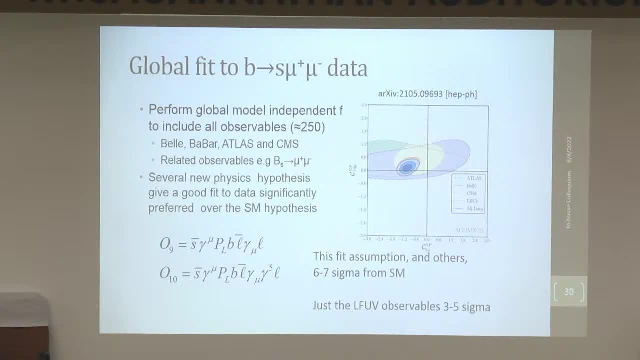 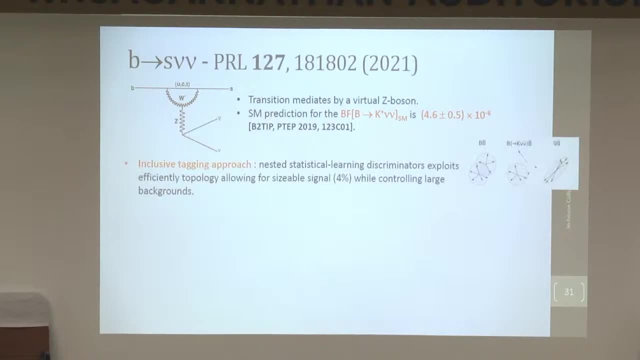 It's just because we've integrated out this, this heavy degree of freedom, So this is like effective field theory type of thing. Yeah, So what's interesting is we're we're getting to a level now with this. It was quite precise upper limit with a very small amount of data. 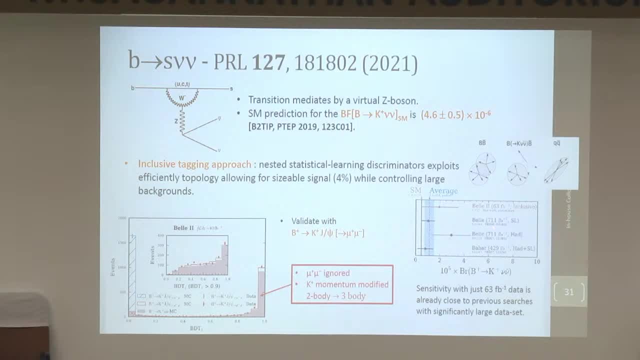 around around 10 times less than previous experiments, And we're updating this at the moment And we we we will potentially be able to measure the standard model value, And whether that disagrees or not with the prediction will be a key indicator. 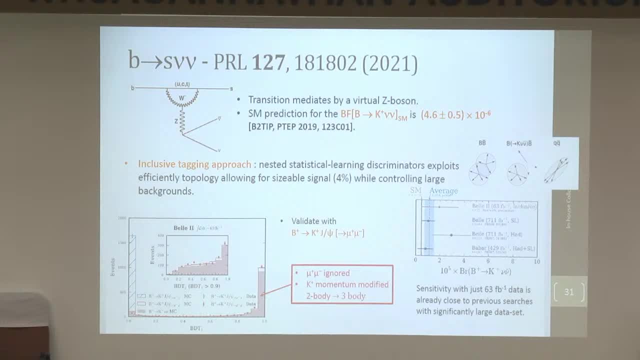 as to whether these anomalies are real, a lot of complementary information about these anomalies and if it's different from the standard model prediction, I think people will really start to believe that this is something new, because it's in a completely different process to this B2SLL. 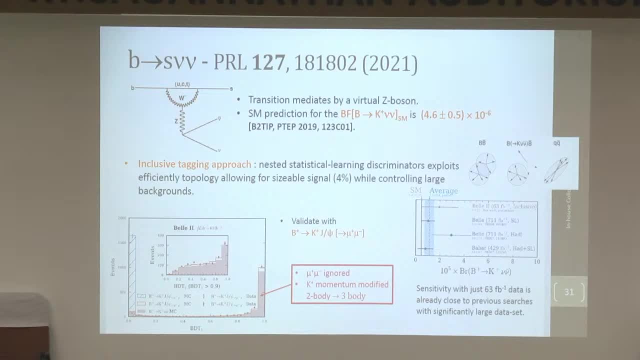 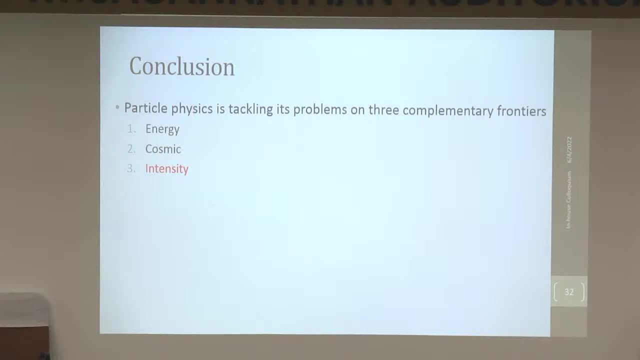 so essentially, I'm telling you here to stay tuned. sorry, I've gone over time. so what I've tried to tell you about today are these complementary approaches to how we're tackling the problems of particle physics and these three frontiers- and intensity frontier is where flavor physics is going- 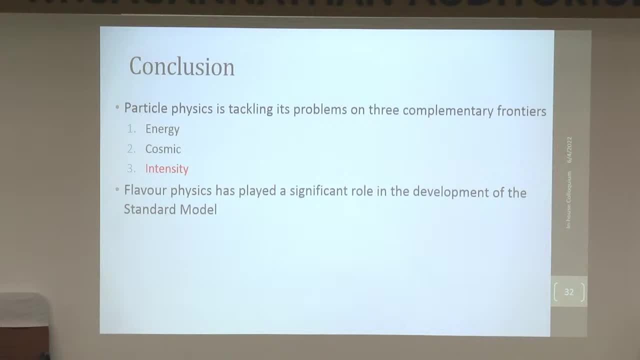 and how. in the past we've helped push the standard model to where it is today, and we hope to push it with some new physics discoveries in the years ahead. so this will, of course, be done not just by us, but also by LHCb and also ATLAS and CMS. 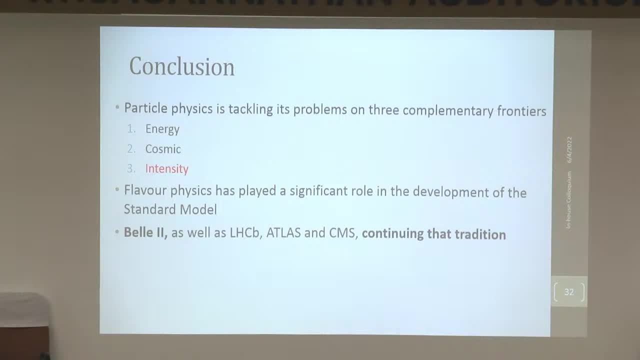 the large detectors at the LHC are becoming more and more interested in B physics because we're seeing these differences away from the standard model and there's a huge amount of resources going into that in the next runs of the LHC. so by the summer we'll have this data set. 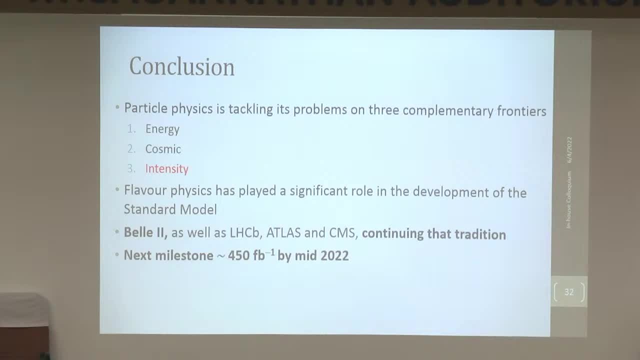 which is roughly the size of what the bar had and half the size of bell 2. then we're shutting down for some work on the detector and the accelerator and we'll start again in late 2023 and from there we'll push through to the next decade. 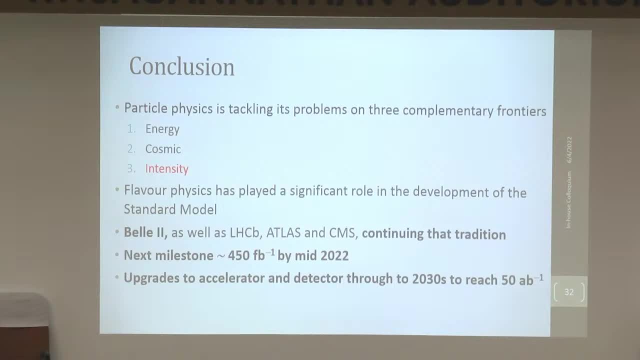 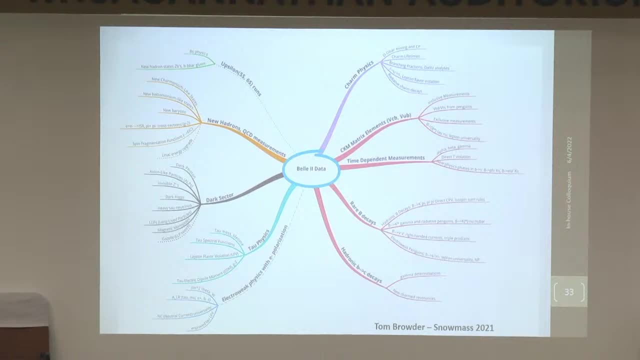 particle physics is a long business to try and reach our 50 inverse atta binds. so just to leave you with a few things, I've got two slides left, both with big images on it, to see if you're still awake. so this neuron diagram was created for the so-called 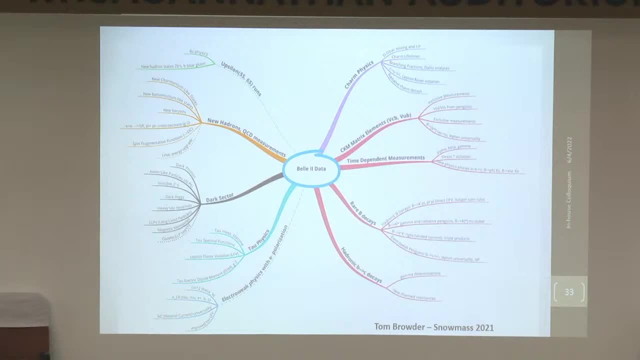 SNOMAS process in the US, which is once a decade. they define the program for particle physics. but these neurons that come out here are supposed to show different areas of flavor physics and QCD physics here, and also this dark matter stuff, Tau physics. these are all different things we can do here. 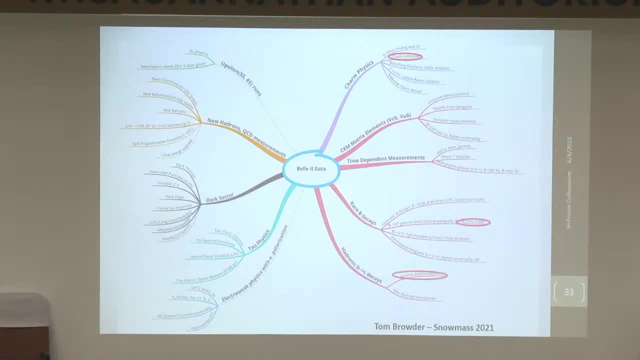 you can't read any of this, but what I told you today is just a little bit of information. but there's three of these things. so there's a huge program of work that goes on bell 2 that keeps the thousands of us busy, and one can expect to hear much more about bell 2 in the years ahead. 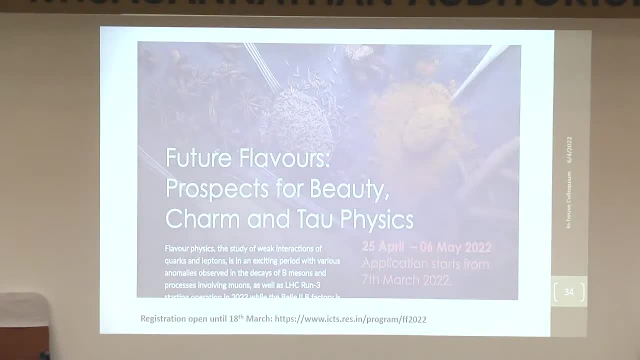 now, if I have made you interested about flavor physics at all and you are a student or a postdoc, we are actually running a school at ICTS, not at ICTS we were. I think we will be one of the last online experiences. it's all about flavor physics. 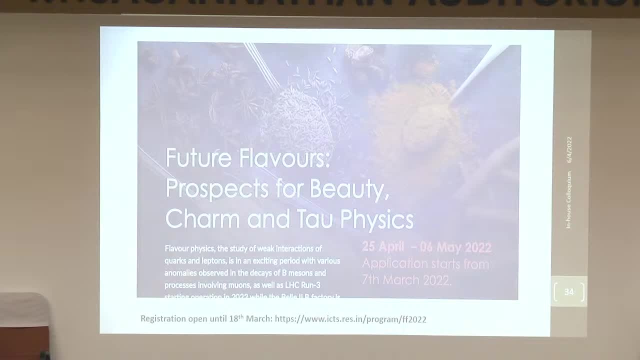 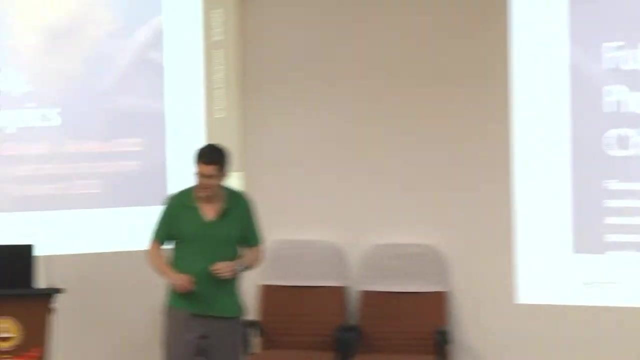 we've got eight lecturers who will introduce various aspects of what we've been talking about in much more detail, so if you're interested, please register. finish with the flavorful theme. you can see how we have done our advertising here, okay, so thank you very much. that's all I have to say today. 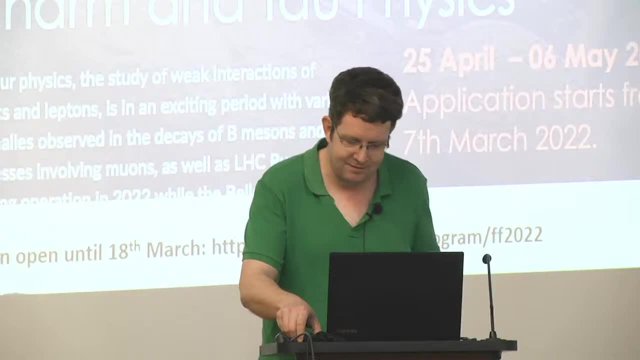 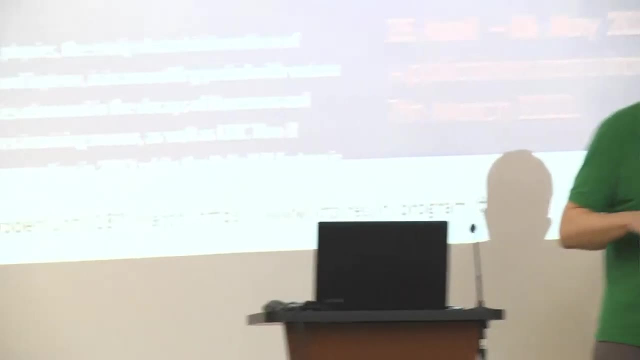 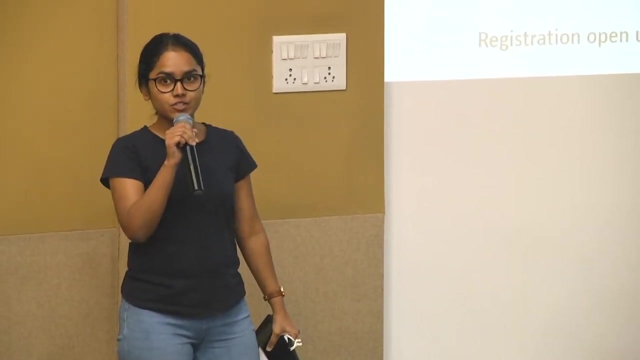 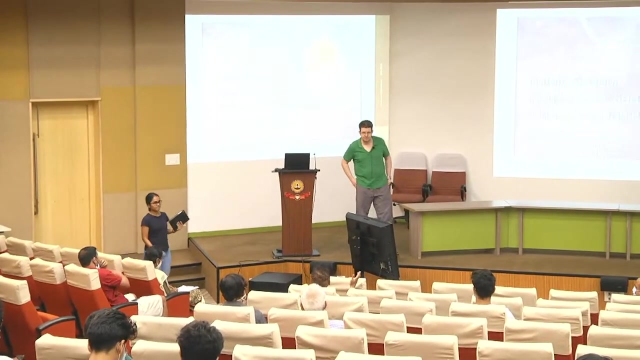 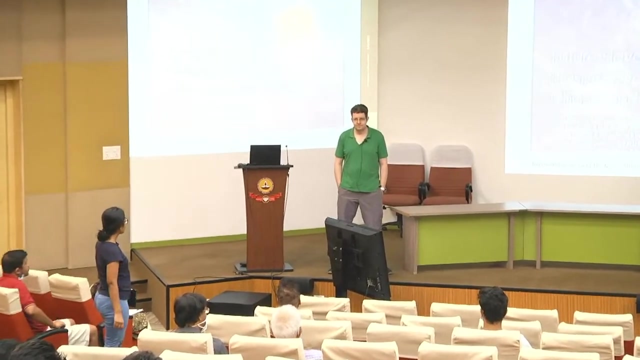 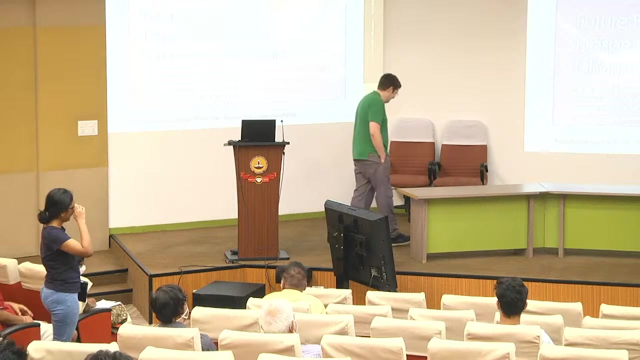 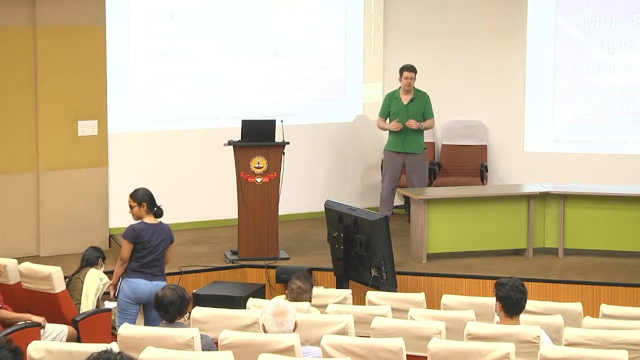 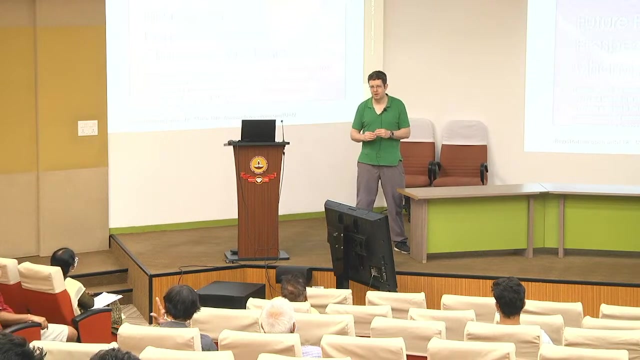 thank you, Professor Libby, for the nice talk and a very wide audience. if you should have any questions, you should. the ambulance was chased. yes, yeah, to explain the. he's a. well, oh, I'll, yes, now, thank you, all right, of course, it looks like a어도. 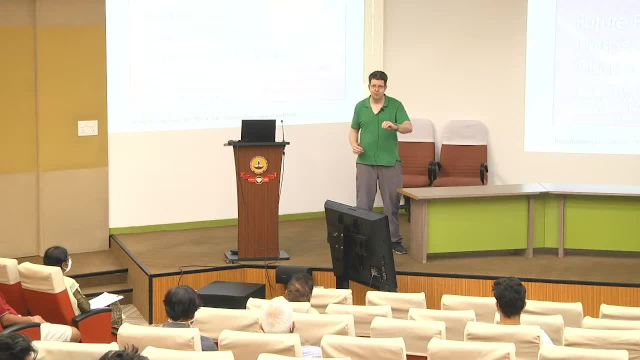 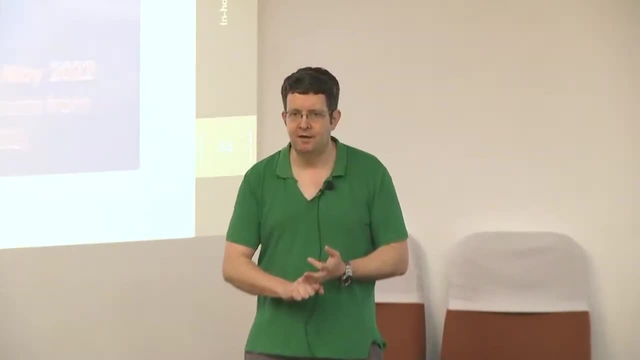 we'll come back and speak a little bit to you later. goodbye. can't have anything in the first generation, Otherwise we would have seen it somewhere else. So that's, to my knowledge, the only theory that seems to be working, with all the anomalies together. 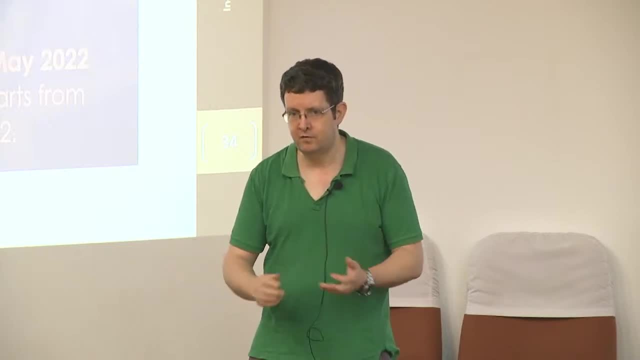 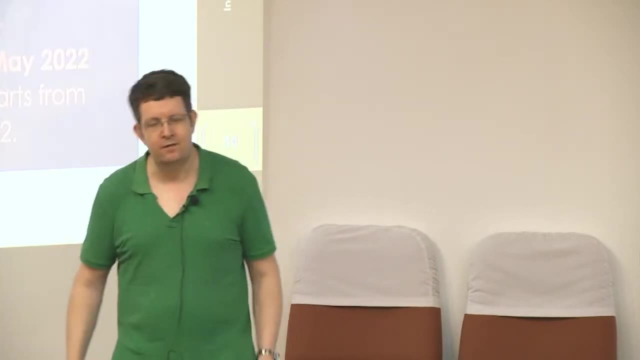 B to SLL. essentially you can whatever you want, whether it be supersymmetry or additional Higgs sector. the gauge symmetry Z primes, all of this is possible there. So people like an extra gauge symmetry, a new force-type. 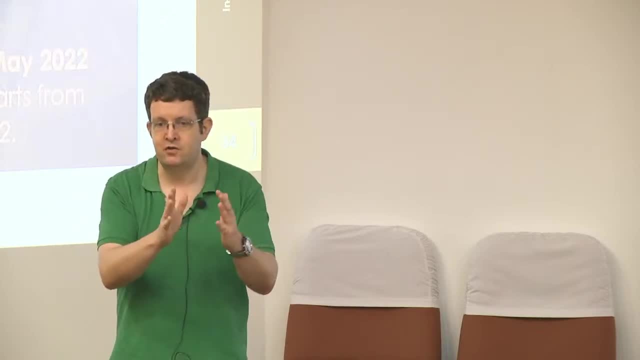 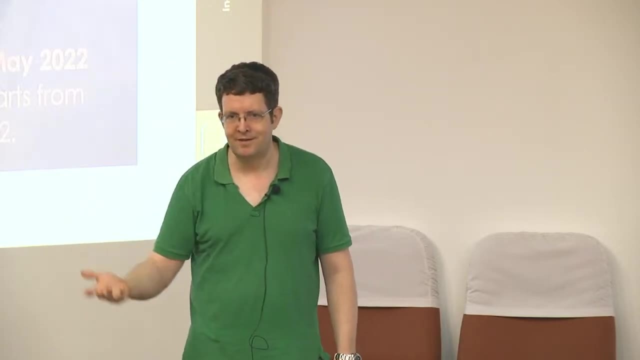 thing where you'd have a new Z prime which would be introduced in that box diagram and not elsewhere, And it would be at a mass scale that's so high that we would never have seen it at LEP or anything like this, And it's not being produced at the LHC. 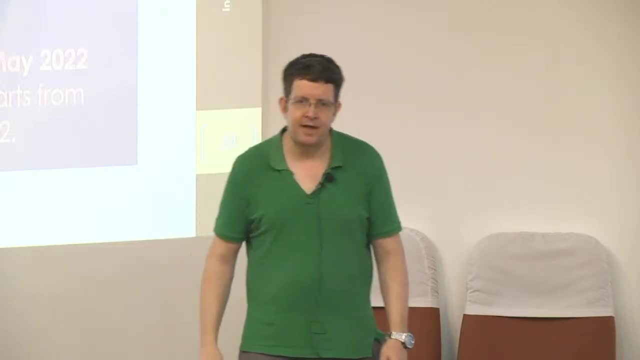 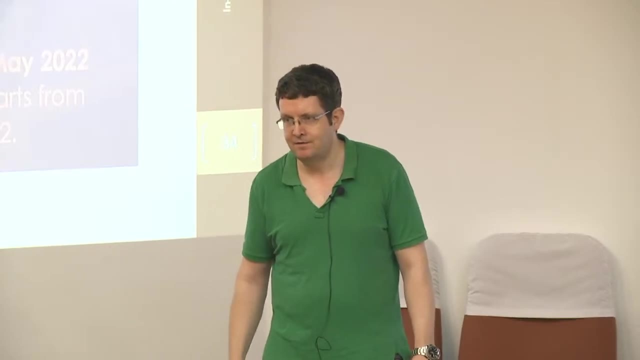 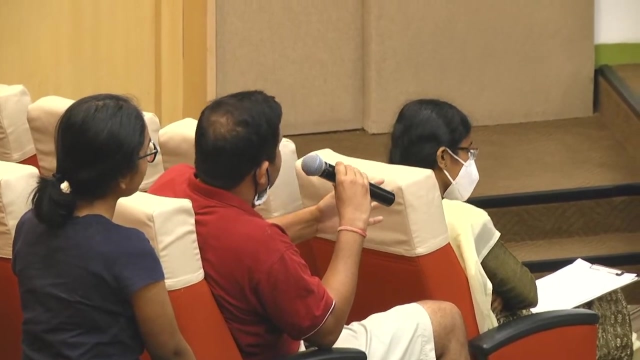 because, again, it's so heavy that it's not within the kinematic reach of the LHC, talking in quantum mechanics. so these particles, let's say B0 bar to B0 transition, it is small, Yeah, Spontaneous, correct. 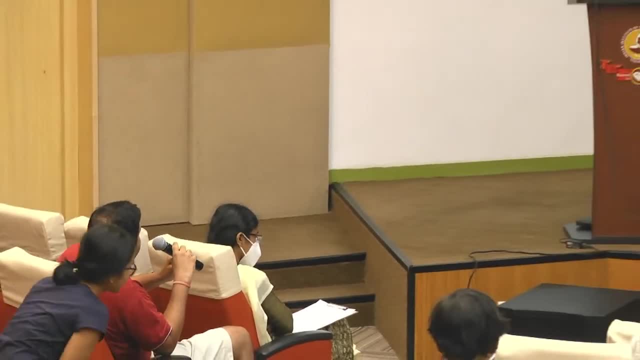 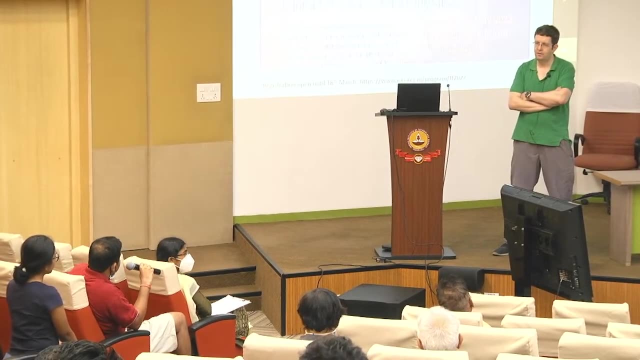 Well, it goes through this box diagram. So it's not spontaneous. It's happening, But as it propagates it oscillates via the box. Yeah, So I think D0 has a very less rate compared to B. B is very almost spontaneous, they claim. 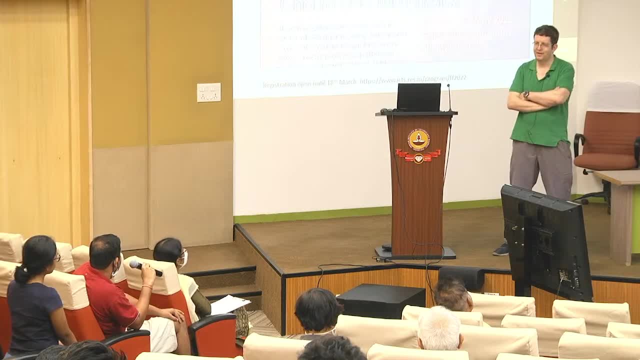 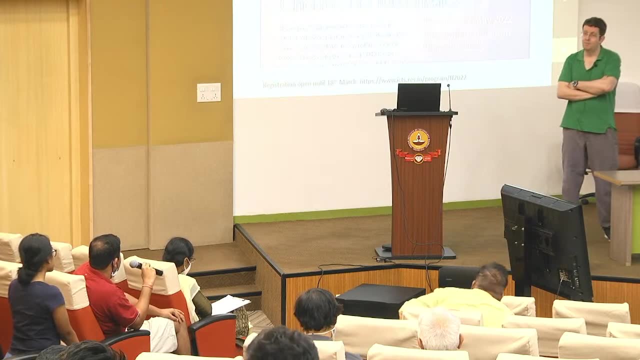 in quantum mechanics. The thing is that I'm not quite sure what you mean by spontaneous. It has a time associated with it. The mixing rate is known. We measure the frequency of the mixing And we measure the mixing frequency in charm quarks. 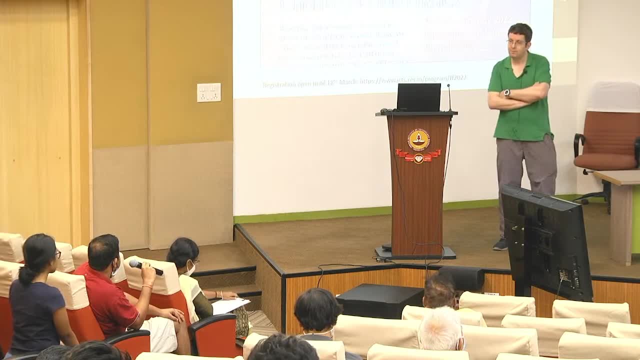 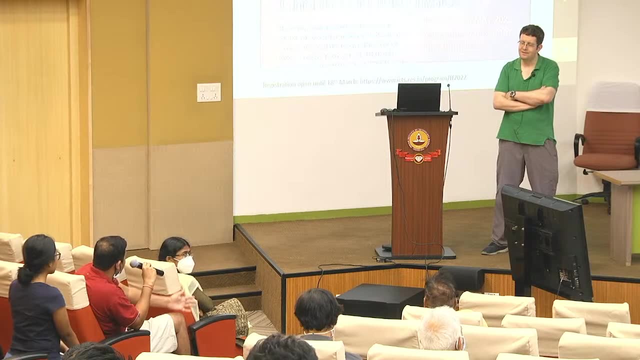 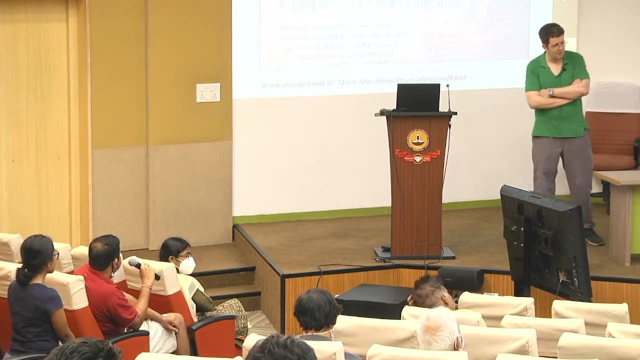 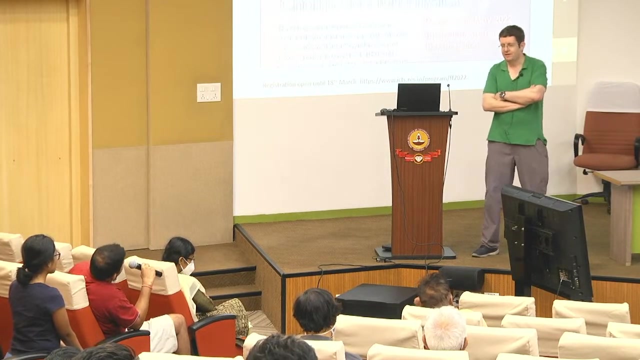 now as well. X and Y are measured really well, So we know. So that's what I think. So the question actually led from here is: what is the definition of a particle? So in terms of you mean B, mixing the fact? 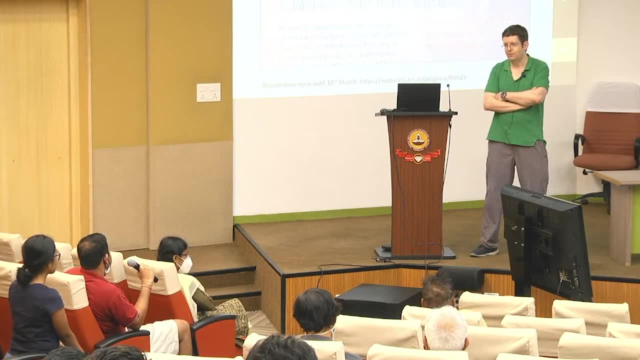 that you can turn from a B0 to a B0 bar. these deltas. Yeah, So it's a delta B equal to 2.. Yeah, As their composite it's OK. right, I can write down a diagram in the standard model. 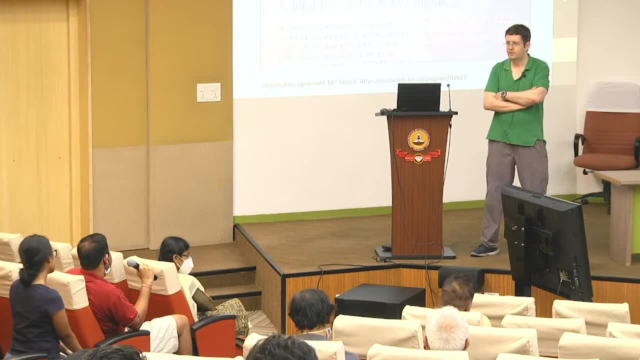 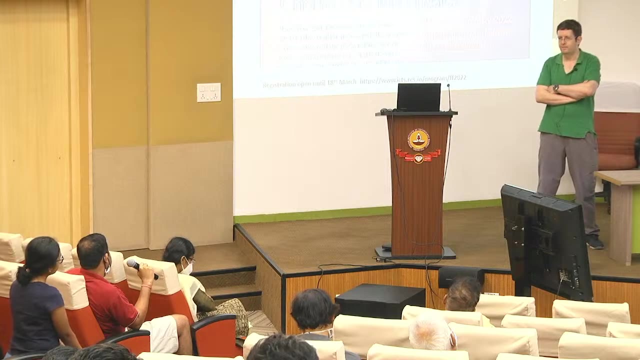 which converts, And because there's this small mass difference between the two weak eigenstates, light and heavy, I get the mixing OK. So there's no issue here that I'm violating matter and antimatter because mixing is here, Because it's not a. 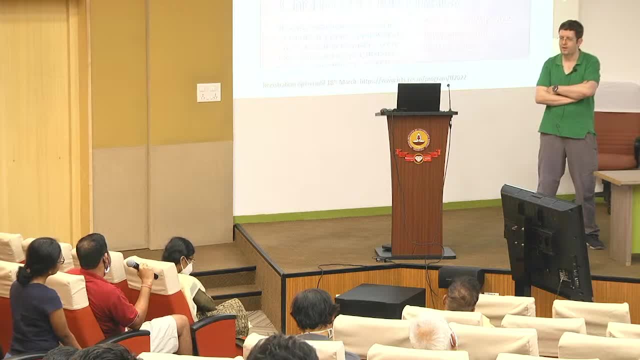 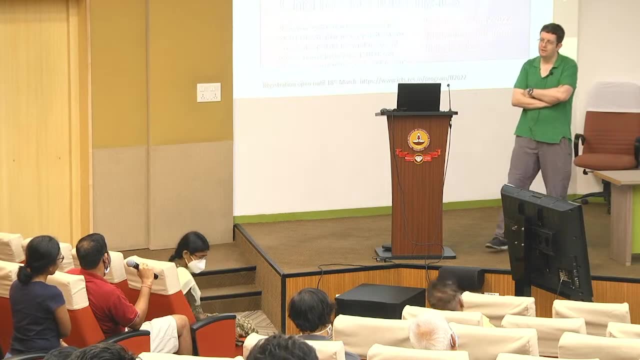 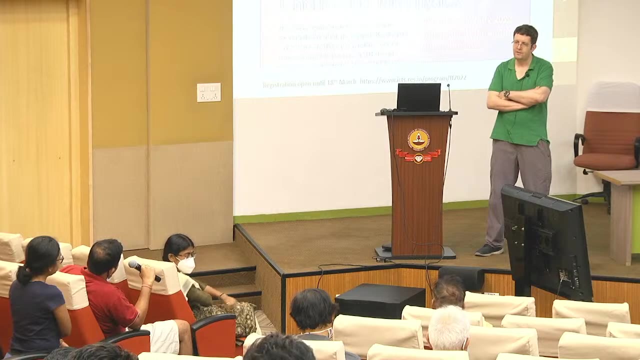 Mental particle. I do it through that box And that box rate. you calculate this And given the mass of the top quark, you predict the mixing rate. And similarly, charm mixing is driven by the bottom quark mass. B mixing loop. 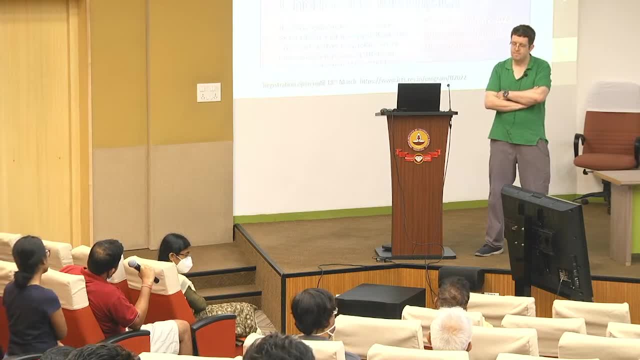 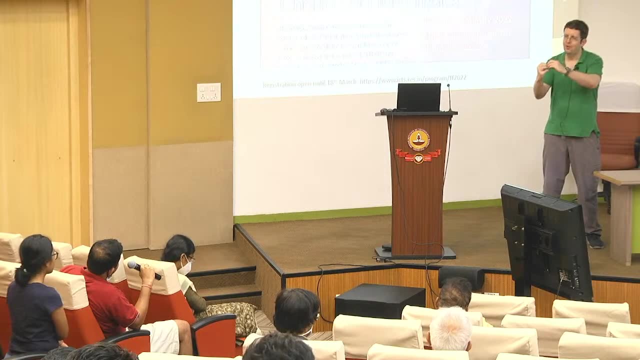 So these all come out and they're all predicted reasonably well. B mixing less so, because there are long range effects where you can get it going to two pions decaying to two pions, and then the two pions merge to form a- D. So that's the way. 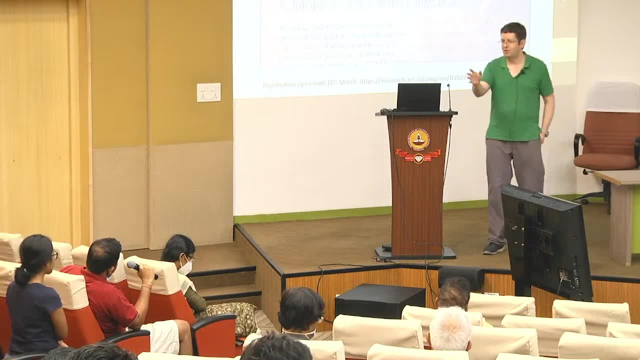 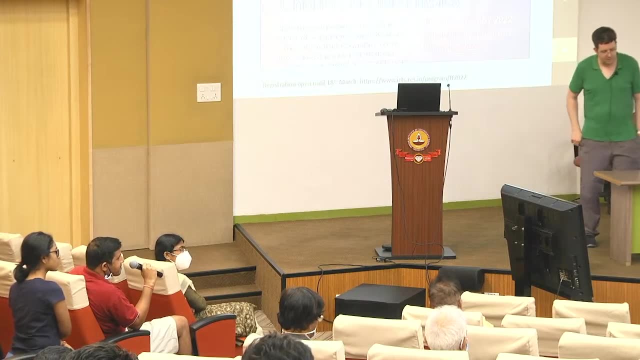 That's the long range effect, because there's hadronization there. So that's maybe what you mean by spontaneous short range, long range, Yeah, So I don't exactly recall. You know when I'm saying that I'm turning a B0 into B0 bar. 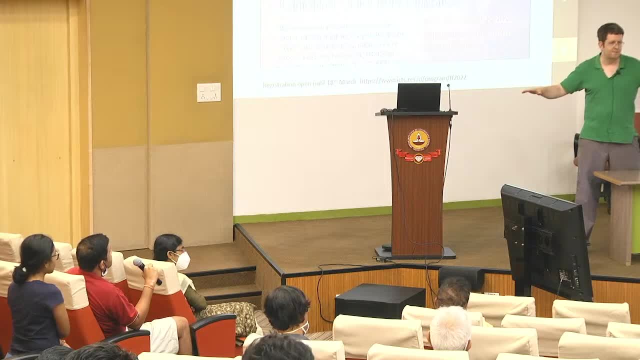 it looks like I'm violating matter antimatter right, But in fact I'm not, because I've got two quarks that have changed. So the overall baryon number remains the same. So the idea that what I asked is because correct me. 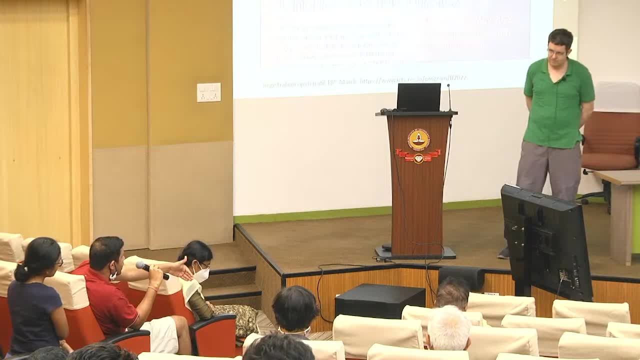 So the idea is, if you talk about quantum mechanics, quantum mechanics will tell you that the transition between this flavor mix, this is what is called oscillation Flavor oscillation B0 to B and B to B0. And this, what I know, is supposed to be spontaneous. 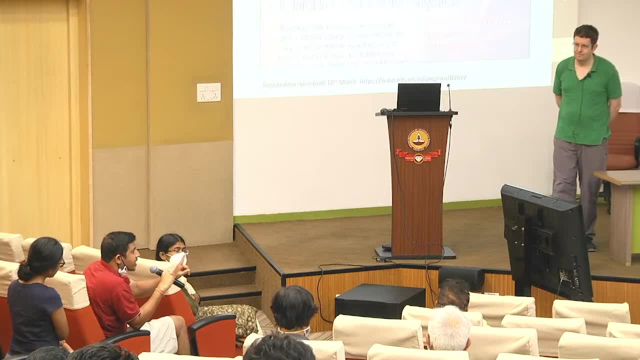 in case of B measure. And if that is true, then which one is a particle and which one is an antiparticle? It's actually the same guy. So the entire definition of a particle and antiparticle is a completely complex thing. 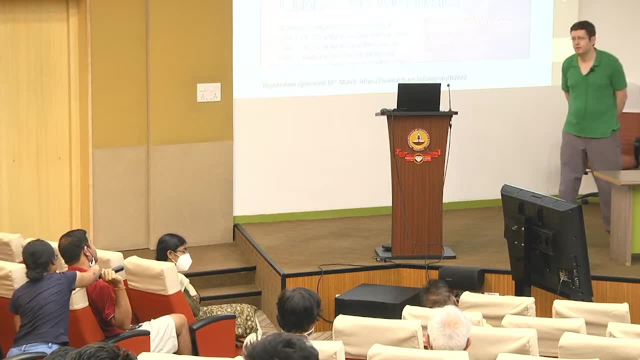 No, no, that's CP conjugate. Sorry, But as soon as one of them decays, you know, unless it's going to an eigenstate, Jim, I think that is true for D measure, But I am talking here B0 to B. 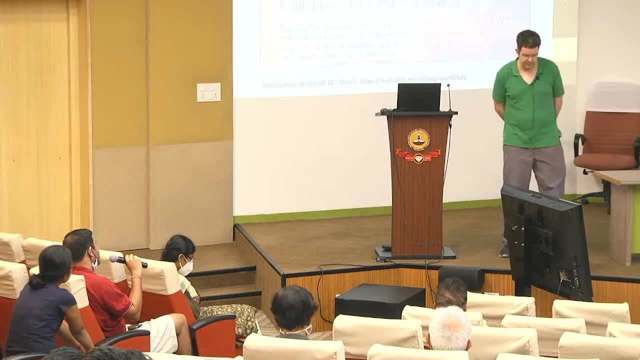 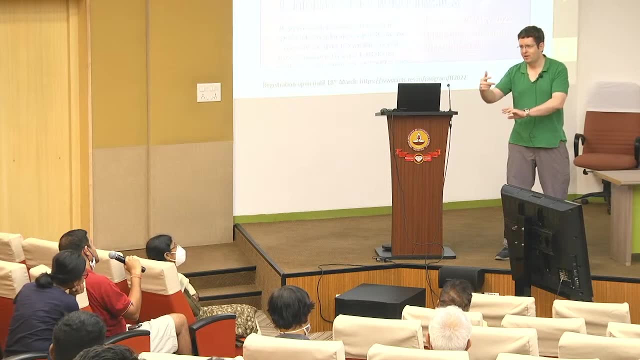 B0, semi-leptonic decay. If I know it's going to the charge of the lepton tells me unambiguously what it is at that time And I can also know how it was formed by tagging the other B. So I know what it was born as and I know what it dies as. 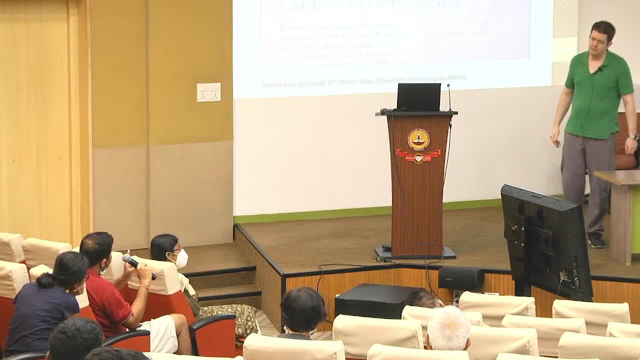 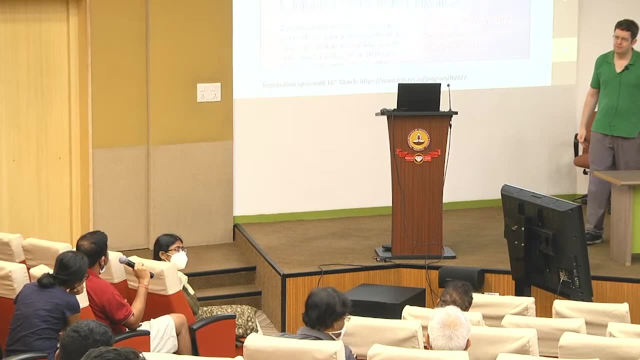 And hence I know whether it's mixed or unmixed, Because what I think is B decays very, very fast compared to the rest of the B0 and other stuff. So that's why the confusion was: What is the definition of a particle? 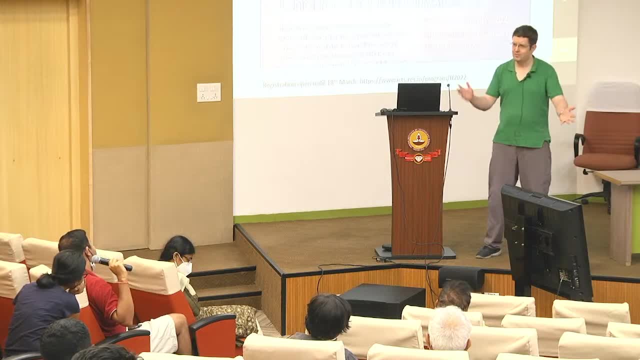 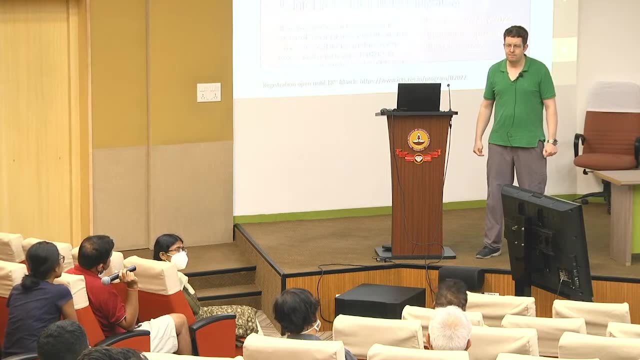 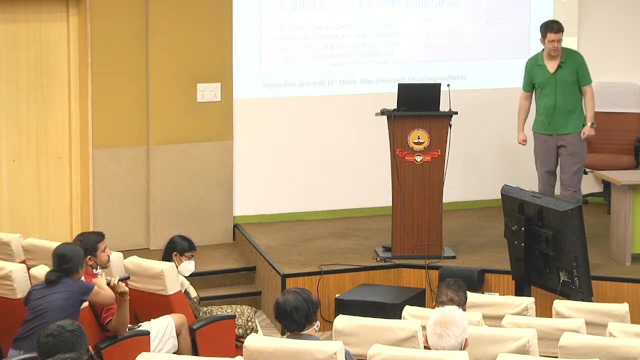 When they try to. I think it's clear to me. I know which one's, the one with the B quark and the other with B minus. That's clear, But neutral mesons. this is not an issue as far as I'm aware. 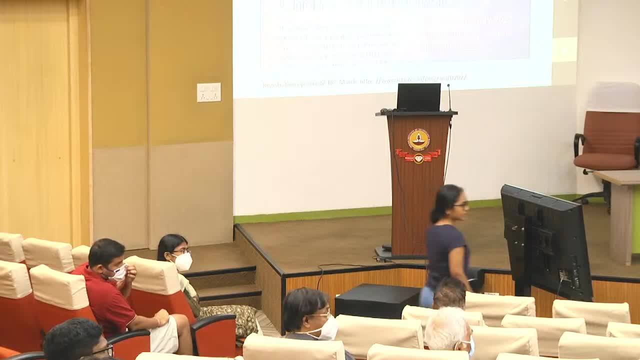 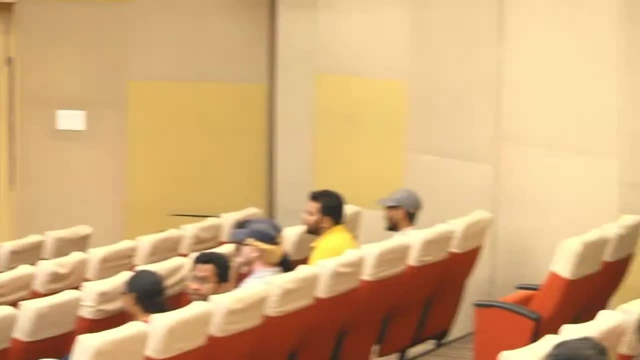 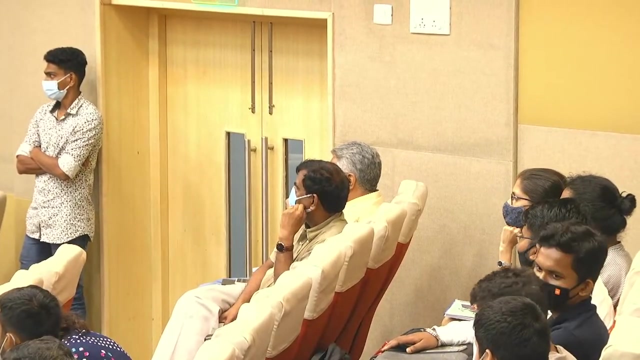 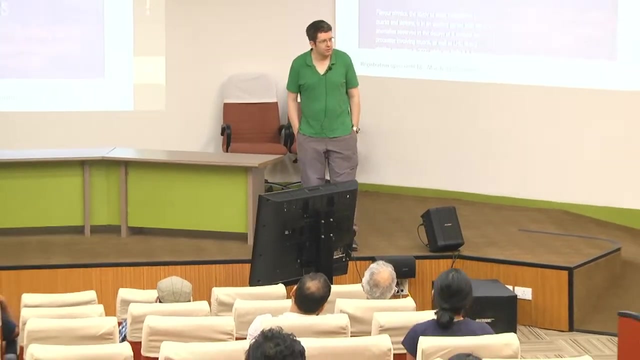 Jim here. Yes, I'm here. Yeah, Yeah, So, Yeah. So what is the distribution of anti-matter in the universe? We know that stars and galaxies are matter, but So there are various things that have been measured. There's a famous experiment called AMS, which sits on the International Space Station, which measures the relative number of protons and anti-protons in cosmic rays, And the ratio there is small, It's like 10 to the minus 6. Though you can locally produce with higher energy cosmic rays. 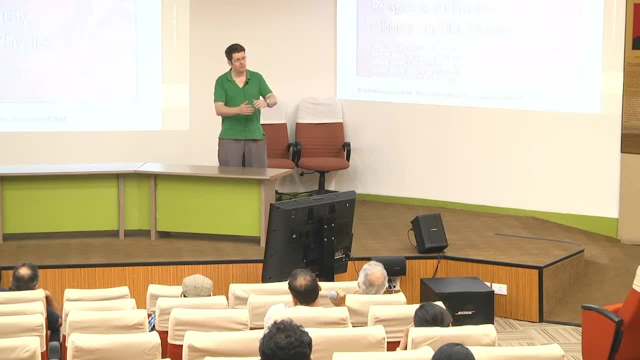 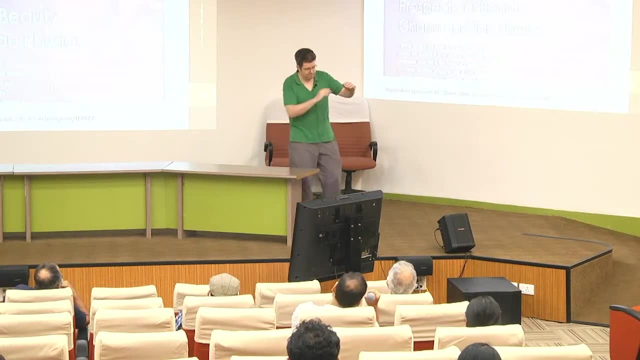 you can easily produce a proton-antiproton, So you expect some anti-protons, But the rate is suppressed. But what we do know is that the ratio of matter to photons in the universe is, I think, around 10 to the minus 9.. 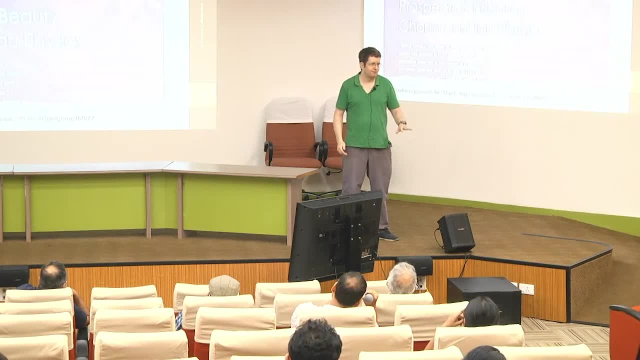 So the abundance of matter relative to photons is telling us somewhere the anti-matter disappeared And in the early universe there was a time when things dropped out of equilibrium and there was a process that took place that essentially violated what we consider baryon number today. So does it fit? Does it disappear in the sense of energy lost? Not energy lost, It's just there was a preferential decay to matter, So the process which was in equilibrium was producing more matter than anti-matter, And that had to come from CP violation. 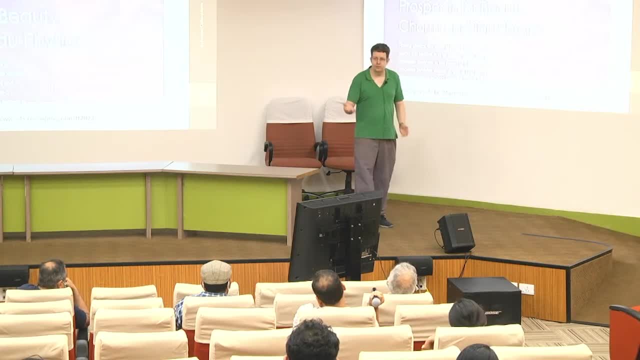 And we can do this to a tiny level in the lab, but we cannot do it to the extent that's required. But these theories in neutrinos, which are called leptogenesis- it's a big claim- can actually drive the whole matter-anti-matter asymmetry in the universe. 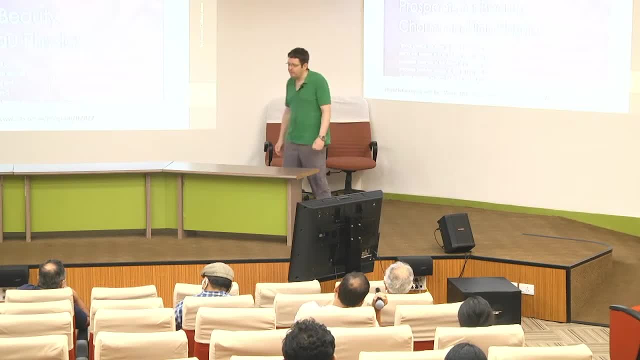 And if we see CP violation in neutrinos, that would be a hint of that. But it's a very different scale at very early times in the universe. so it's hard for us to probe experimentally because the energies are so large. 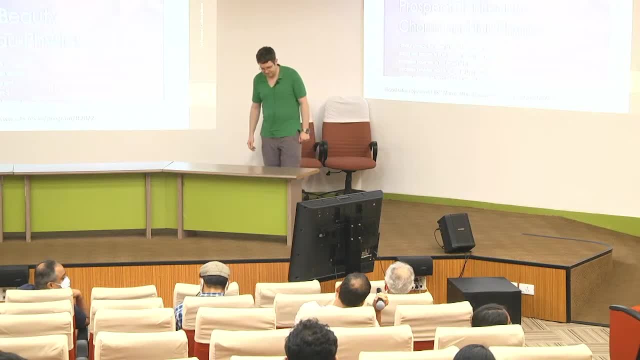 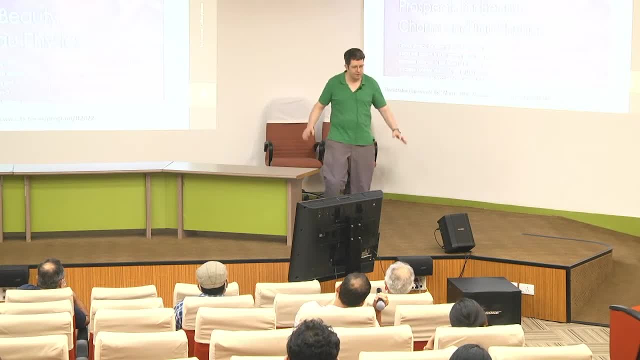 And then the empirical piece of evidence, because people argued that maybe the universe is clumpier than we think, Maybe bits of the universe are made of anti-matter and bits are made of matter And we've just been fooling ourselves because it looks largely symmetric. 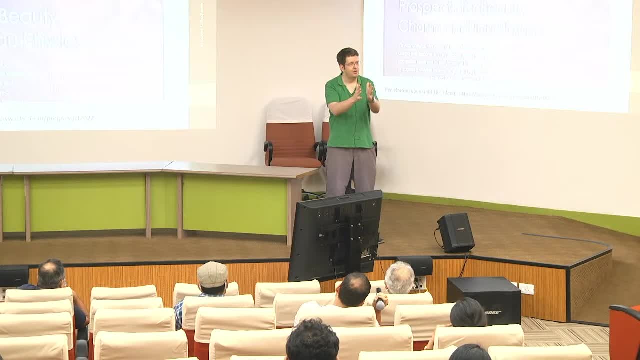 But there would be a place where the two interface with one another And you would be expecting a background of very high energy gamma rays coming from such an interface between these two parts of the universe, And that, of course, has not been observed. 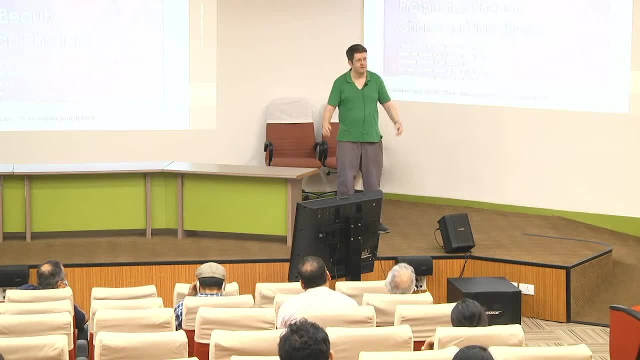 So that's why we think the universe we see, even back to the earliest times, is matter-dominated, And this matter-dominance happened behind that CMB radiation point, where we can't see anymore how it happened, And it probably happened in the very earliest. within, I think, 20 or something I hear, But I can't remember. You may remember the time scales better when the matter-antimatter very much left. Yeah, very much left. I can look it up the book. 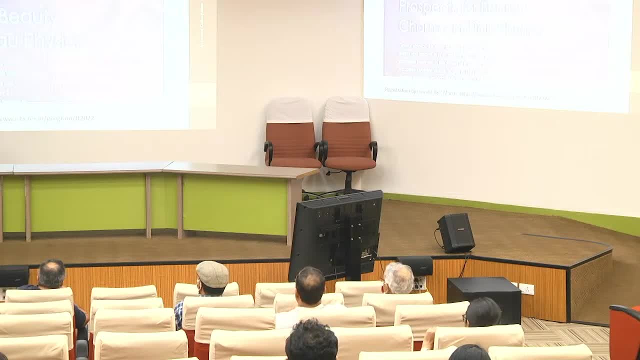 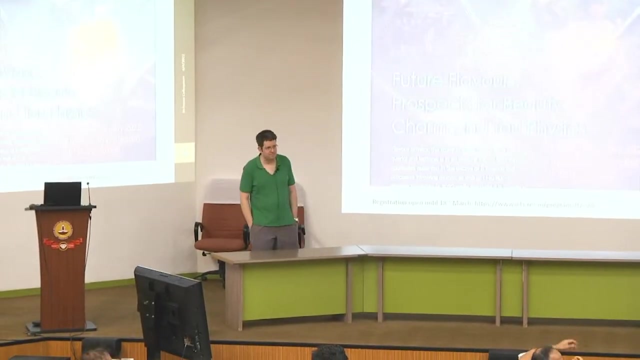 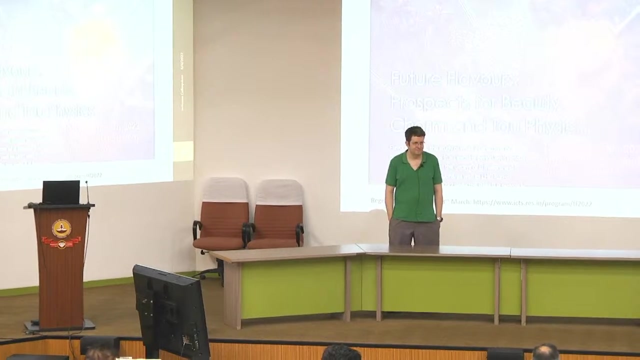 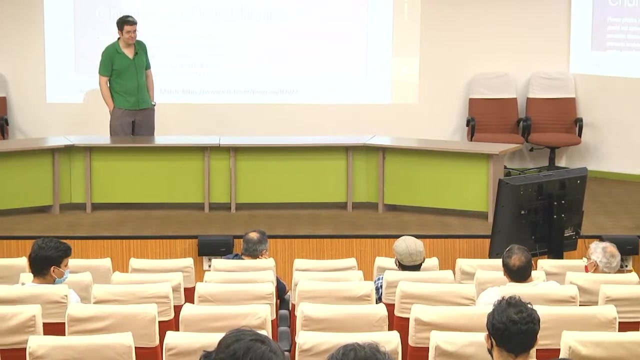 I can look that bit up. The cosmic microwave background experiment doesn't give a direct evidence of how much of antimatter has been lost, right, interesting talk. so it gives our basic concept of particle physics. okay, what do we read in master's level? so i have a general question regarding this. all types of particle detector. 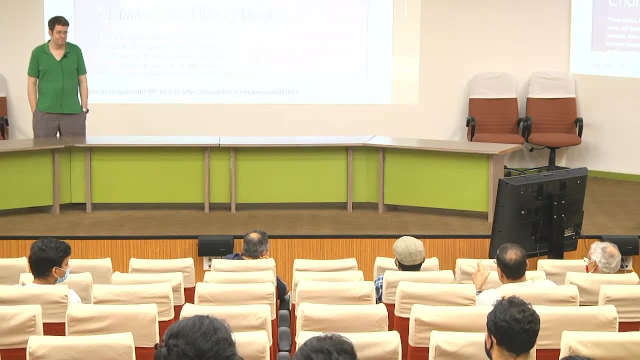 we have the cms on cms detector and this atlas detector, barber, and now you are talking about this bell 2 detector. so how can you understand this? so all the objective, all the detectors are the same, or they are all the competitor, or they are the parallel set of detector. 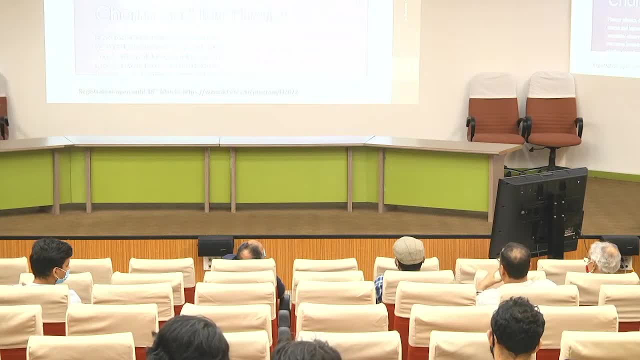 so how can you in layman language, how can you understand all this? particle detectors in terms of efficiency, or so it's specialization, okay. so, um, cms and atlas are detectors designed to measure new things, primarily the higgs boson at very high energies. you so we're talking about tv collisions there, whereas bell 2 is at 10 gv. so that immediately means 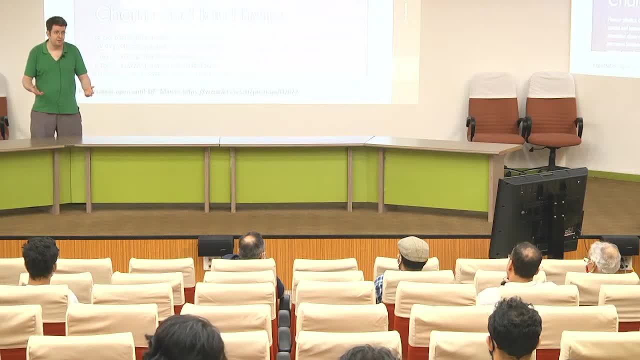 particles are much slower, lower energy, so you need to have different detectors which are sensitive to those lower energy particles. so many atlas and cms measurements cut off at gvs- that's their lower limit. whereas that would we'd lose everything. we have very few gv particles in our detector. 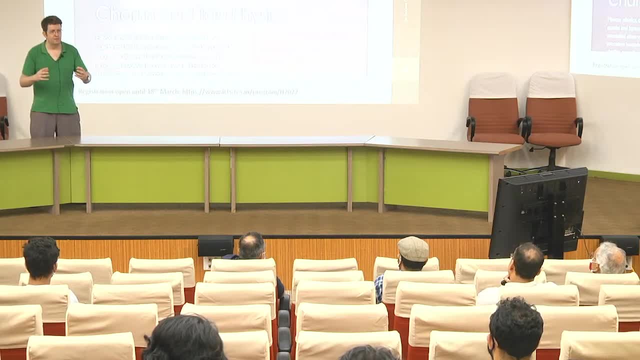 so there's a lot of different detectors that are sensitive to those lower energy particles. the detectors are designed to measure things at the appropriate energy scale and they're looking for different things. so this is this intensity energy frontier. in the intensity frontier you've got a well controlled and well understood process. but my epsilon 4s- i know it decays to b's. i'm just 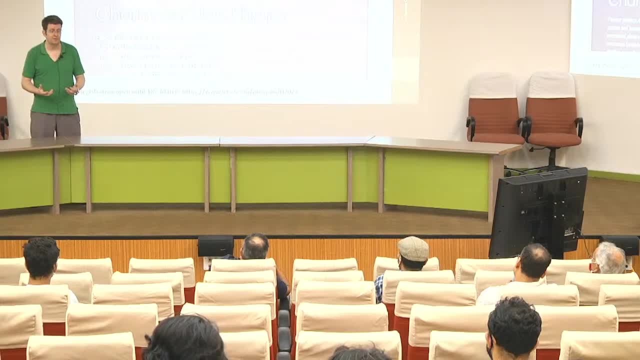 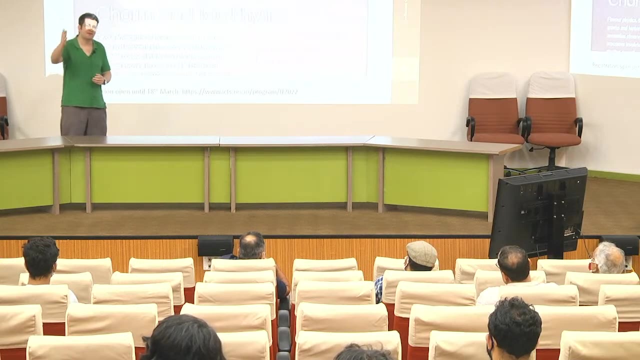 trying to produce more and more and more, to do that statistical measurement at the lhc it was. you know, let's do this, let's push the frontier, let's see if we can produce something new. so they're complementary to one another. now, a more controversial statement. have they turned the camera off? 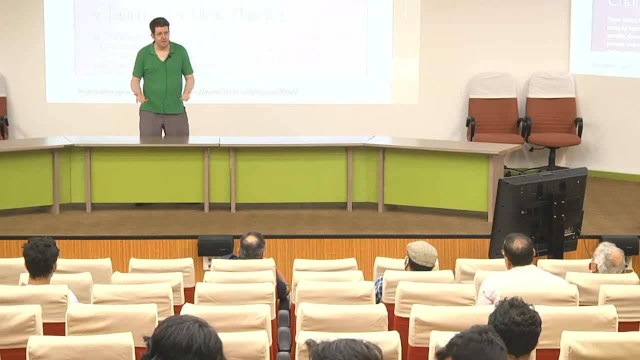 it's the lhc experiments, because they've seen nothing and they're going to run for another. well, there are hints of various things, but they're going to run for another 15 years. they are also doing precision measurements now. a lot of this next run is about measuring. 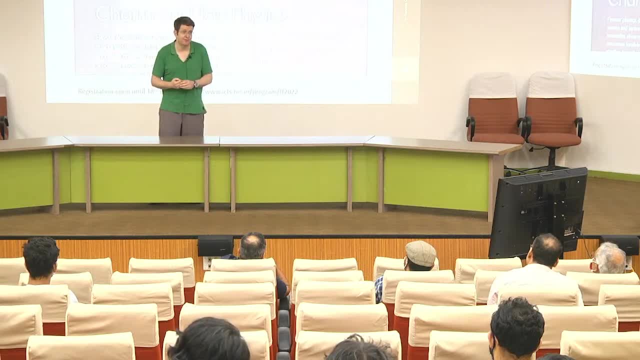 the higgs boson very precisely. they are also doing intensity frontier physics- though they like to still call them the higgs boson- but they're not doing the higgs boson. they're doing the higgs boson themselves, energy frontier physics- but they're measuring things very precisely and looking for 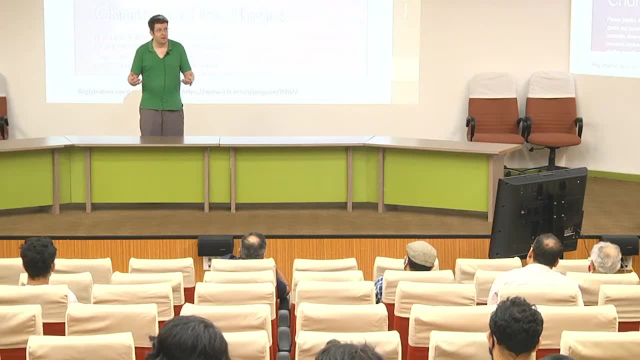 discrepancies. that's really what we're doing now, because we don't have the technology at present to make that big step forward. another order of magnitude, to start looking for new particles of 10 tv mass. it's talked about there's something called fcch which would be built at near cern and 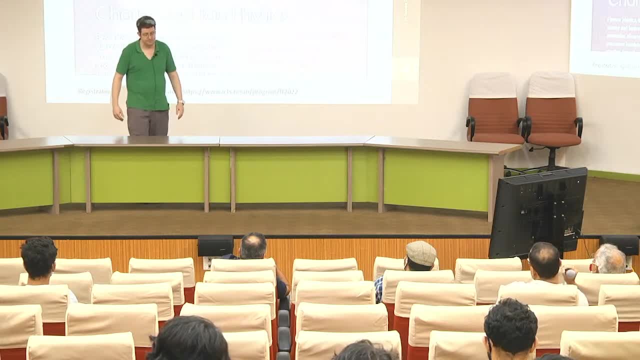 have a hundred kilometer diameter um diameter circumference ring, compared with around 21 for lhc. that might possibly be able to do this, but we're talking about 20- 80s for that to be realizable, so i'll just be happy to be here at that. 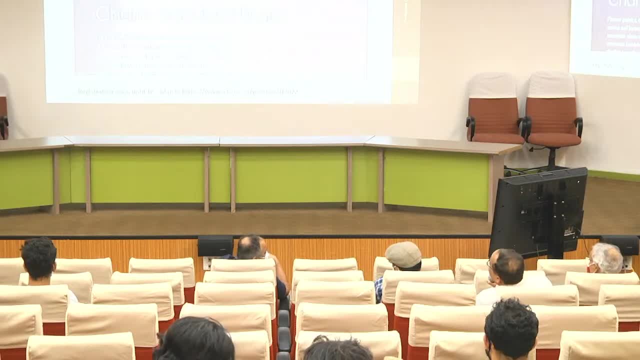 point and one hypothetical question: is there any plan of any particle detector to be said in india? so there is a neutrino experiment that has been much talked about since i came to india, called the indian neutrino observatory, or the ical, which would be sitting. 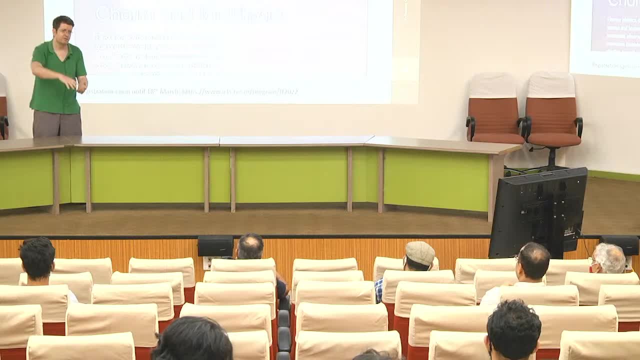 under an overburden of rock to filter out cosmic rays and then measure neutrinos from the atmosphere. that is the biggest indigenous project. they've had problems finding a home. their home was in tamil madu for a while, but that seems to be becoming less likely. now they may move to the himalaya. 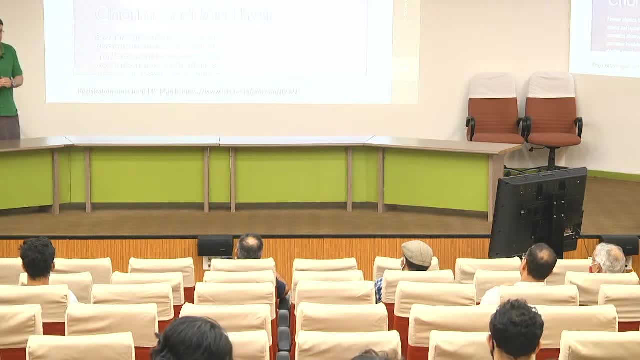 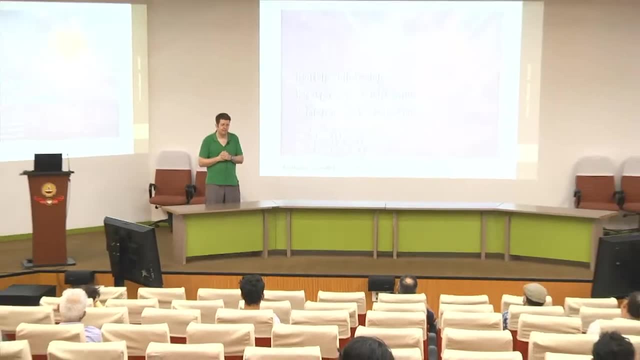 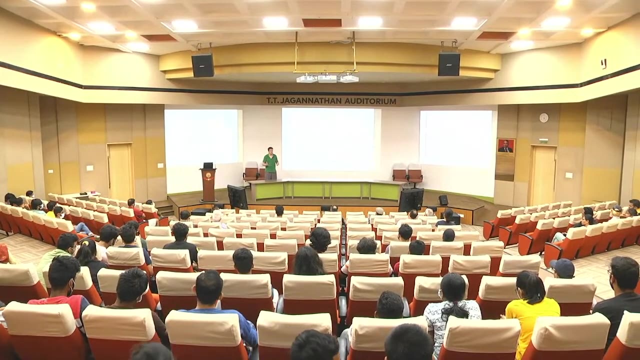 so i it's still on the cards, but it's been very hard to get it moving, so that would that would be it. there are some talk of some smaller things: measuring dark matter, measuring neutrinos, double beta decay- again, these are smaller scale experiments, but there is nothing on terms of colliders. there's no. 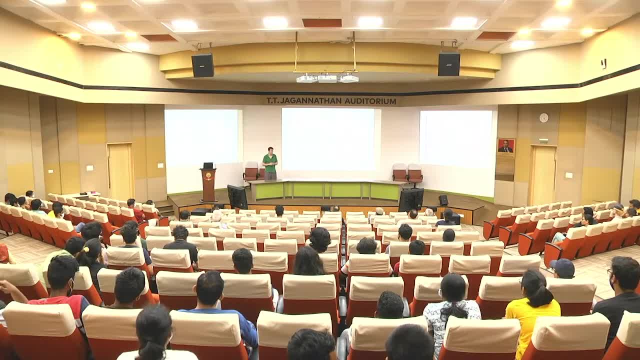 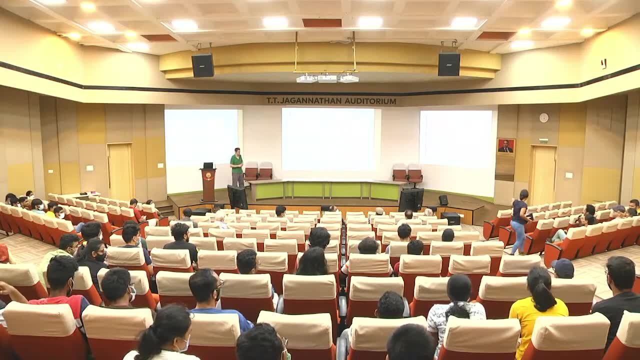 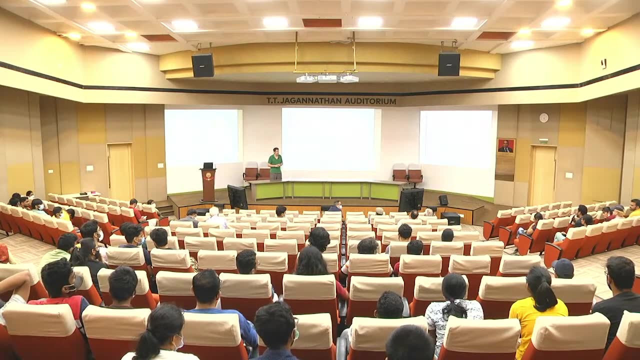 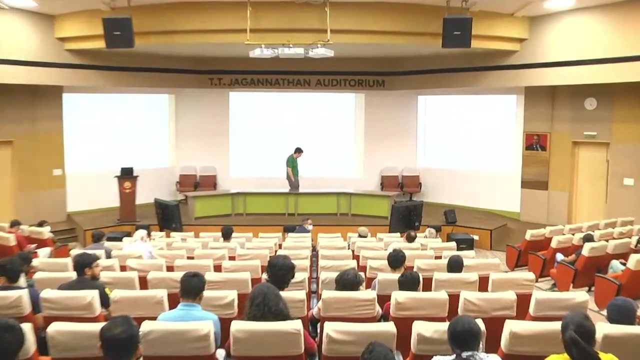 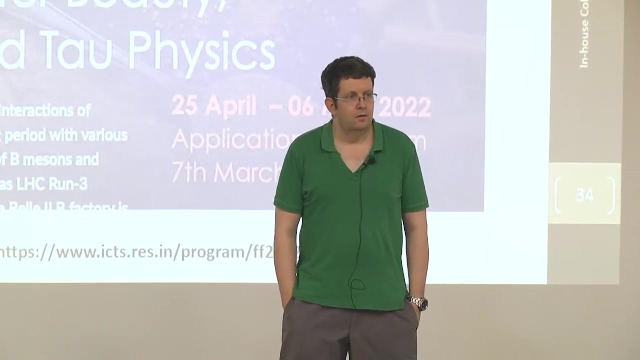 accelerator program to build a collider in india at present. okay, thank you to sir for this nice talk. um, it's sad there is a fourth kind of neutrinos for generation of neutrinos. so, um, if there could be four generation of quarks and oh, uh, this. 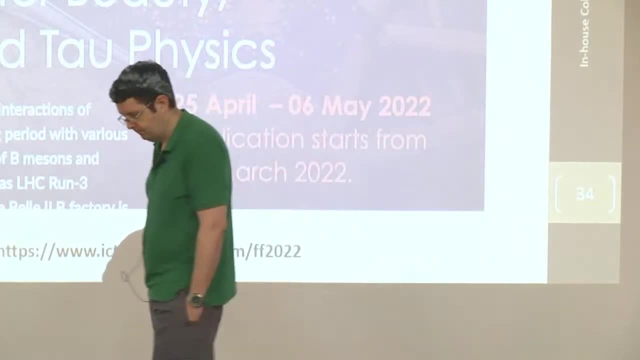 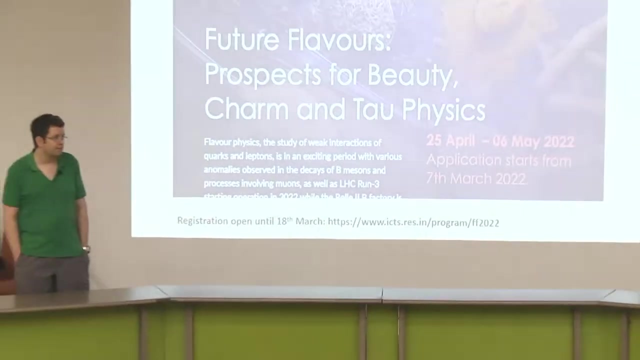 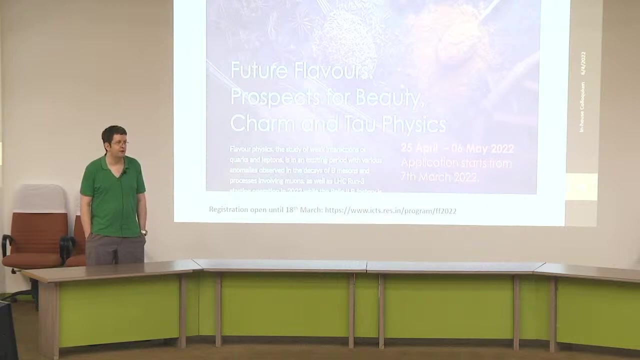 so the all of the measured elements- generation of quarks- are there. there are there. i think there are two questions there. so, on the neutrino anomaly you're talking about, there are a certain set of neutrino experiments, largely based on low energy beams, which have seen an effect that can only be described if you include a fourth neutrino. 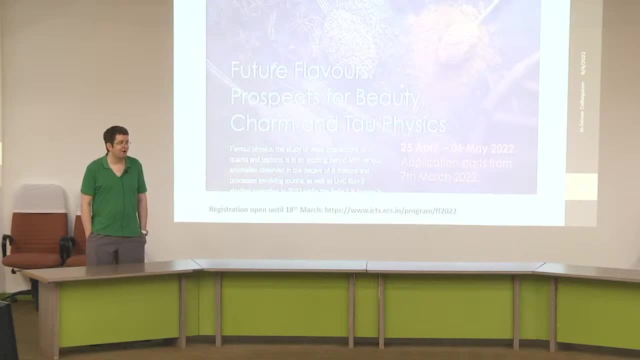 so, but it gets given the name sterile. yeah, yeah, yes, so that tells you that it's not coupling to the standard model in the same way as the other neutrinos. it's already different. it's not really another generation as such as we have in the standard model, where they have the same couplings. 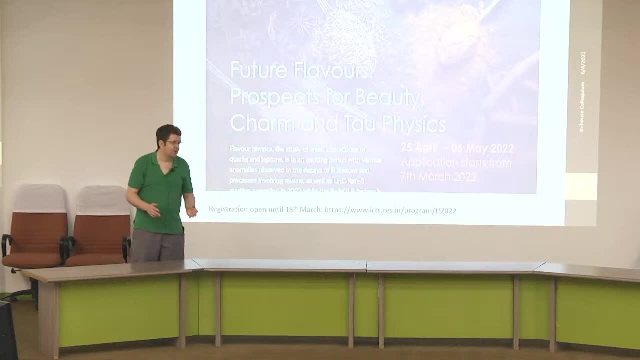 to the w. all right, so that fourth generation in the neutrinos could be something entirely different. and it doesn't necessarily have to have a quark partner, because it's just a neutrino's weak interaction. you know why should it have anything to do with the quarks? 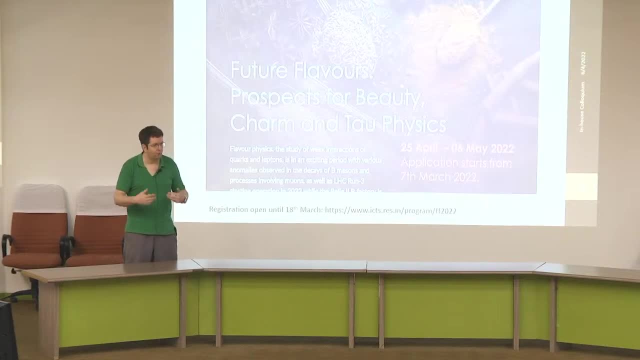 of course, in a grand unified theory on to fourth generation, and people talked a lot about this for a long time- t primes and things, and b primes, the experimental evidence, uh, for the various things, the non-closure of the unitarity triangle, it's very it would lead to that. 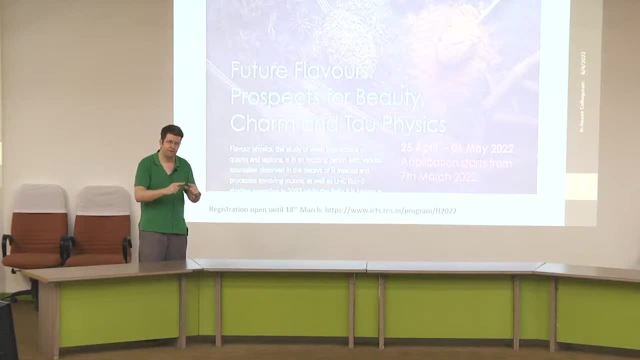 unitary triangle being open, essentially and- and it looks very closed- it's- um, it's not the most accurate explanation, but it's a very, very good example of how we can try to explain flavor of the unitarity triangle and the way that we try to explain. 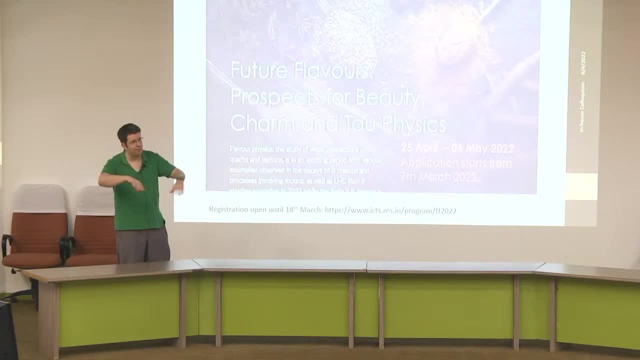 flavor anomalies and things fall into traps when they try and add a fourth generation. because they would have unitarity triangle. because if you've got a four by four unitary matrix, you've got a whole load of other phases that you can add in. okay, you can absorb two more, but you've got more. 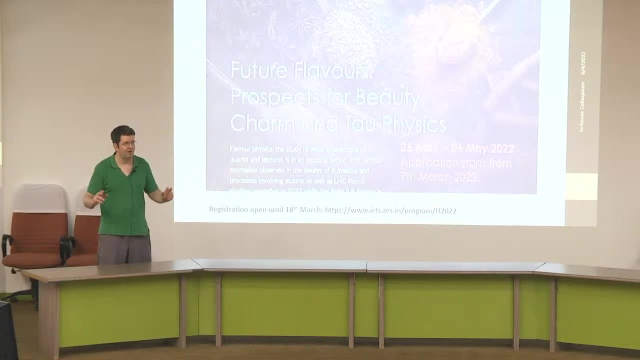 from the unitarity and you should be seeing odd cp violating effects among again have to be sterile in some way in terms of how it mixes with the ones that we already have, And this is less appealing aesthetically, right If you have a fourth generation. why is it so different? 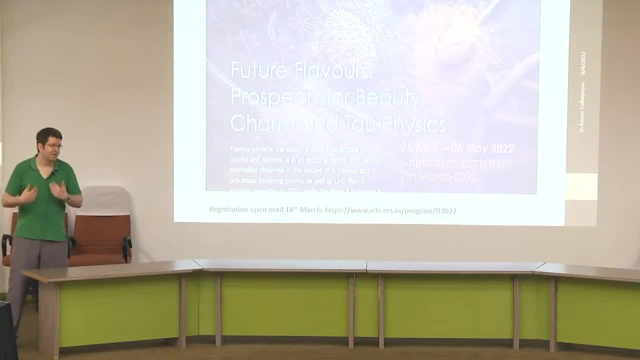 Okay, It might be true. I'm an experimentalist, I don't worry about these things too much, But it's got less appeal. Thank you, I'm not a person to ask, I don't know. That's only constructive. 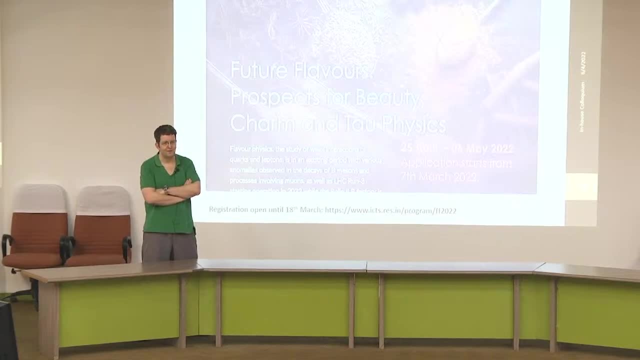 These things are really sterile. So, yeah, most people Are they massless. So there are theories where they're very, very massive ones as well, which would have very different behavior. I would not be ultra-relativist. I'm not the person to ask about this. 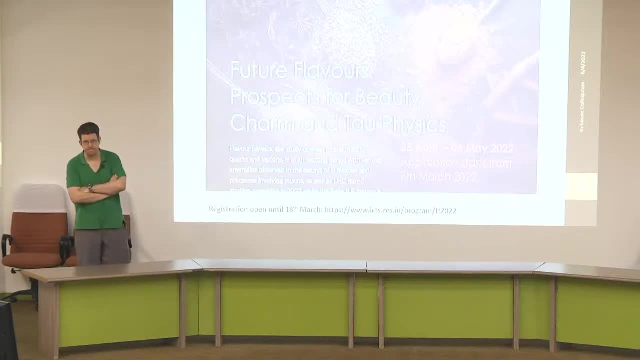 He will give you a much better answer. Hi, Hi. So thanks for this talk. So you just explaining about the CP violation. So this CP violation is mainly generalized. CP violation means weak interaction as well as strong interaction. you are talking here. 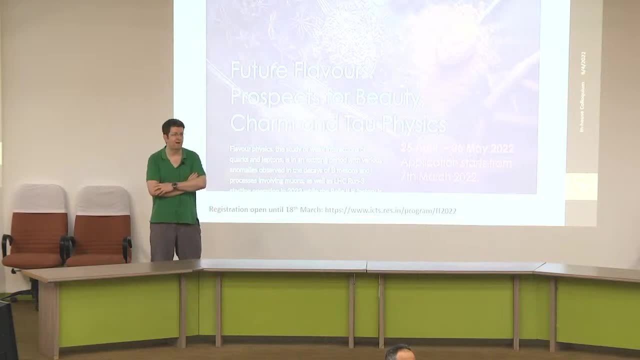 So it's a purely weak effect. Many measurements that are purely strong indicate that strong interaction is CP symmetric. So any collision or any process that's dominated by the strong interaction, you see no evidence for any CP violation to high order, And this is an issue. 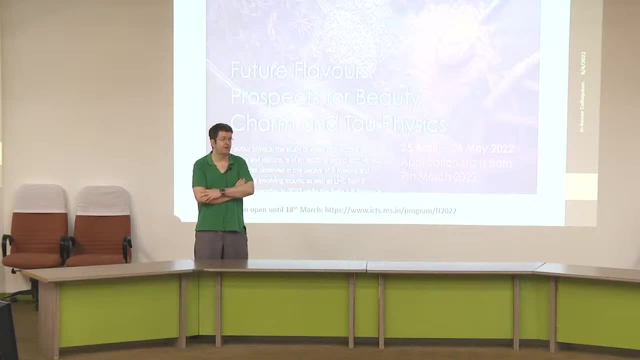 It's something called the strong CP part that, for whatever reason, there you know, you have three colors. you could have in principle generated some CP violation in the quark sector amongst the three different colors of quarks, but it's identically zero. so some people add a. 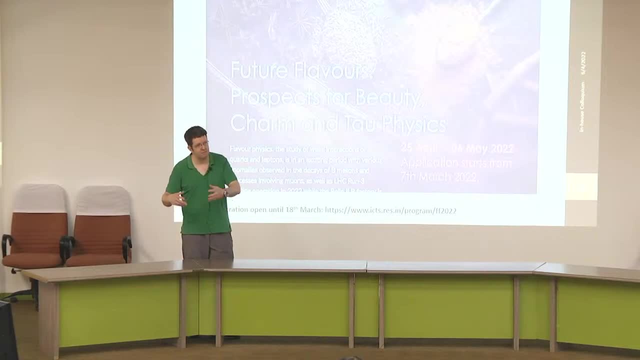 19th parameter to the standard model, which is the Theta strong, the CP violating phase in the strong sector, which seems to be zero. now, yeah, some interesting consequences, but basically, with a strong interaction, is CP symmetric, as far as we can tell? empirically, yeah, actually, but for non. 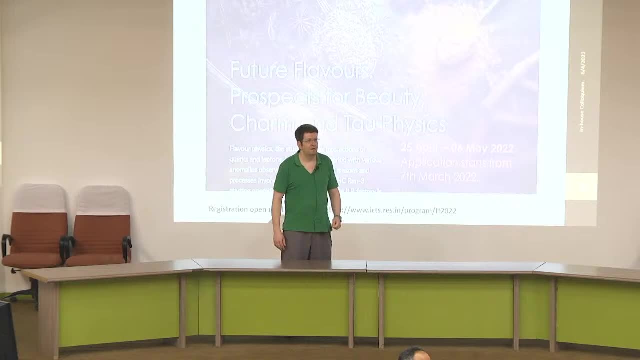 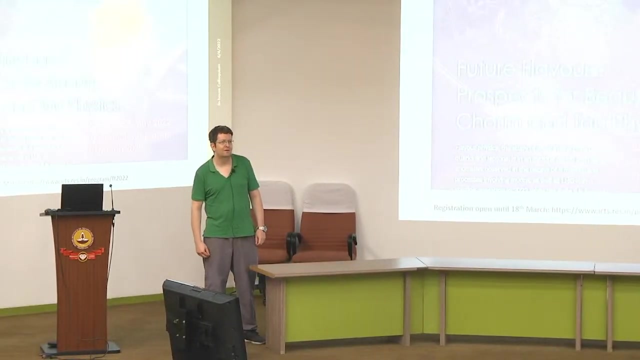 zero neutron electric dipole moment and magnetic dipole moment- yes, I can't hear you very well. science, yeah, the non zero neutron electric dipole moment. and man, we've not measured no local CP globally. then it's, it's conserved. actually I know if you're. 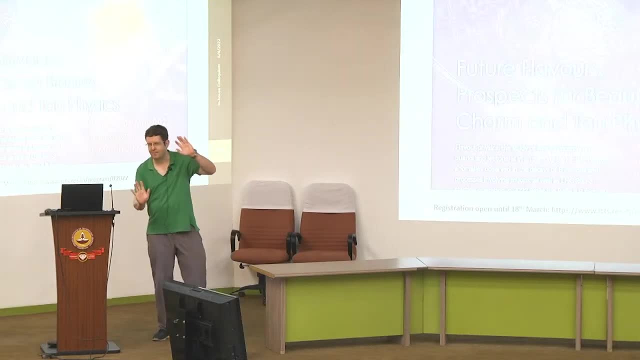 talking local, then we're not somewhere else. that means the opposite. yes, this is locally, not globally, yeah, okay, okay, I'm with you. yeah, that's different, yeah, because, yeah. so so here that asymmetry, you are talking the asymmetry and it, if this is a non zero. so it simplified that. 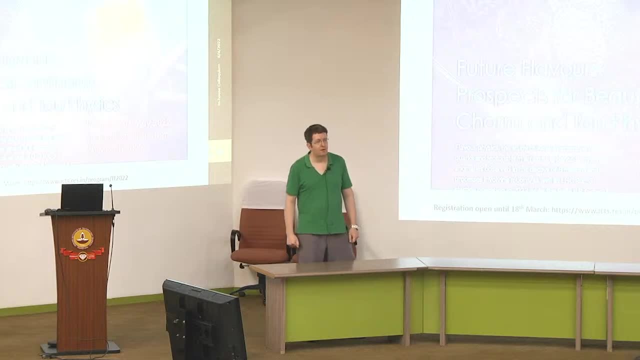 so let's try to understand sim stickers. let us assume that first of all you have a C P separately and then we are hoping a somewhat a regular study first. we're not actually having an example of anолоids K today, but we are just saying that you were saying there could be a ר violation, so you can see. certainly there could be a super violations, right? yeah, so N plus minus and minus by this total. so, as an example, the textbook example of this is actually from neutral cihans, but you have a semi-ottronic decay of a long lived neutral cahen the k long and going to weiß. 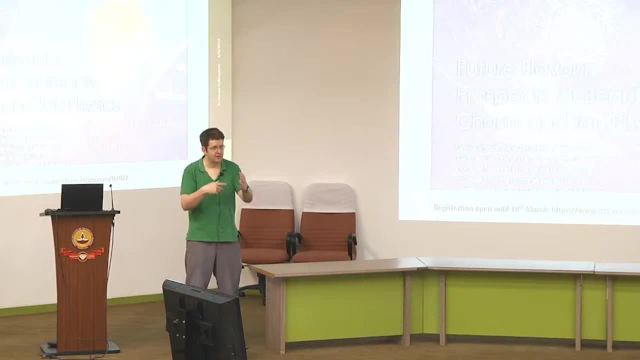 And then it would be a pi plus an electron, a new anti neutrino and then, if you look alom The protections off, pobre هذا conjugate of that, still a k long going to a pi minus and a positron and a neutrino. the rate of those two decays are different. So in fact you produce more positrons than electrons in that given decay. That's a distinct difference between matter and antimatter. That's not local. It's really producing more of one type than another. It's the wrong way around. 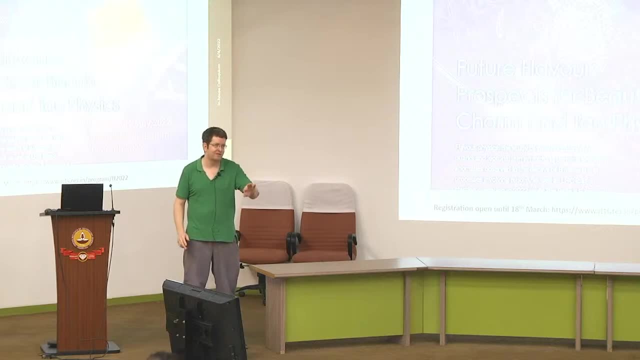 for what we want to do. but that's true of the particular process. So that's what we mean by CP violation. There's a real difference between matter and antimatter's behavior. So the reason of that asymmetry not equal to zero, that number of positive charge and negative. charge. that could be not same. So I know that one reason is chirality imbalance. So is there any other reason that could affect of that? This has got nothing to do with chirality. This is matter-antimatter, not left and right.